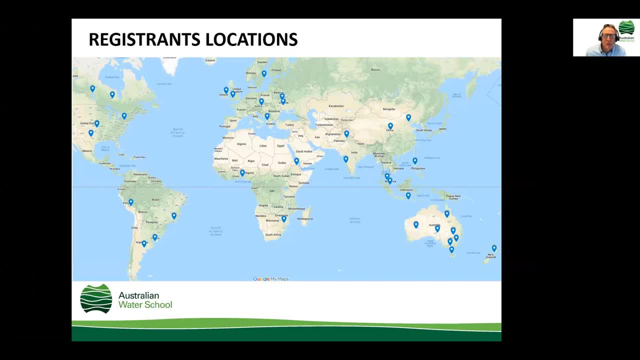 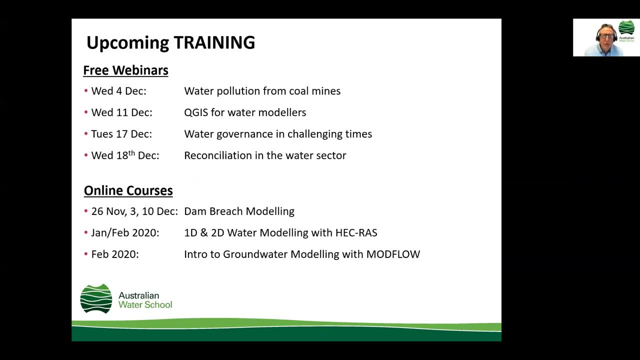 terrific to have this wide group of participants today and I know it's going to be a fantastic time. Upcoming training. you can see their free webinars and online courses every month. This is the program. It's quite big and we invite you to go to the website. 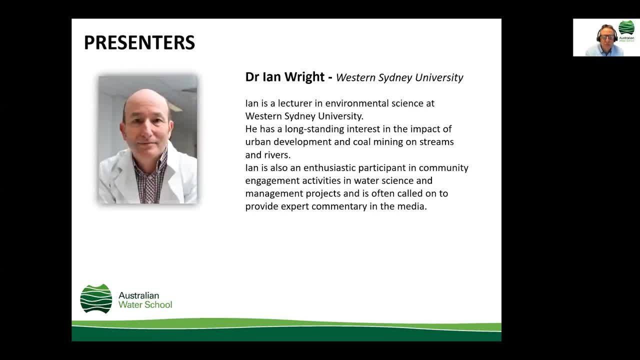 You'll find all the details. It'll be fantastic. So right into it, Let's introduce Dr Ian Wright. Ian's a lecturer in environmental science at Western Sydney University. He has a long-standing interest in the impact of urban development and coal mining on streams and 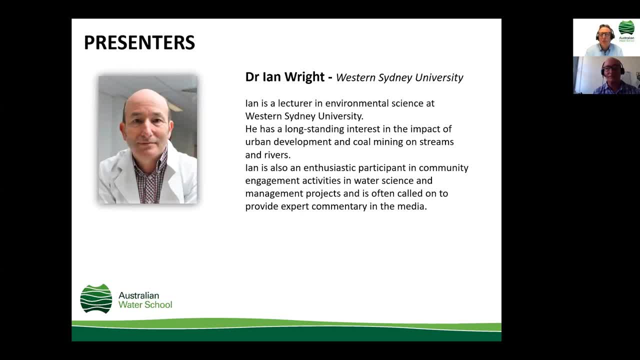 rivers. Ian's also an enthusiastic participant in community engagement activities in water science management projects and is often called on to provide expert commentary in the media. It's a pleasure to welcome you, Ian. How are you today? Very well, thanks, Trevor, Great thrill to be here. 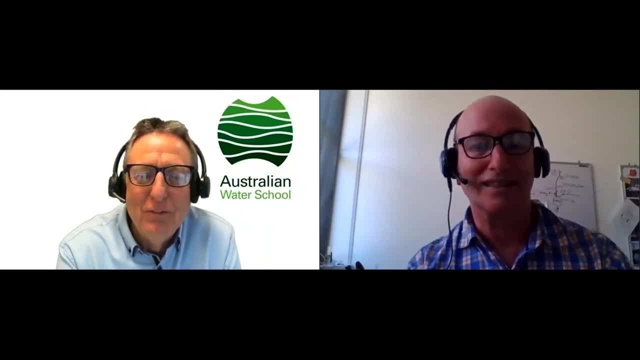 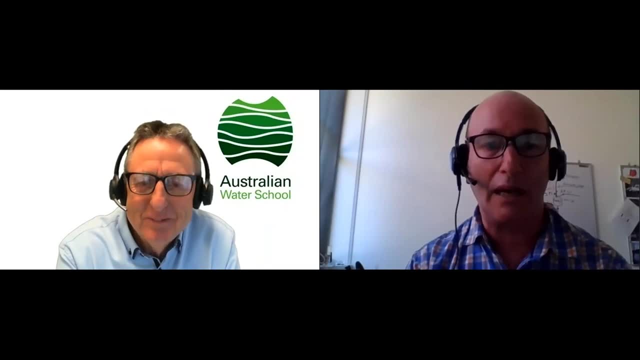 Fantastic. and that last little line about the media. I believe you might have had some work in that area on the weekend. Yeah, we have. indeed There's been some media reports about contamination in a couple of Sydney's water reservoirs. Always issues with water and coal mines. 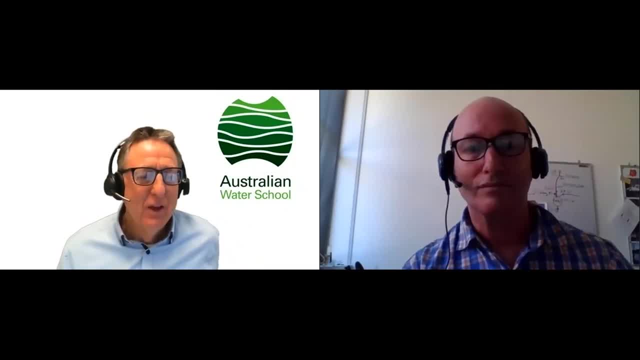 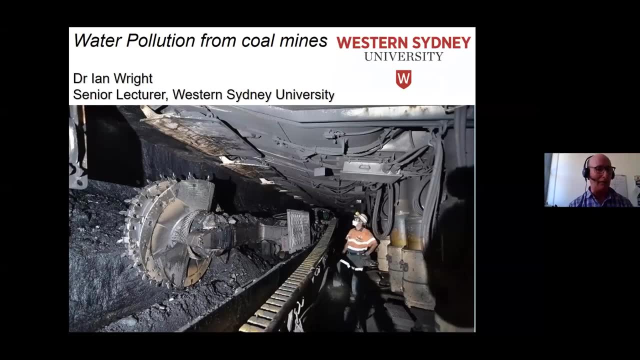 Keeps you on your toes, I imagine. Absolutely Well, I think we'll get straight into this, Ian, Thank you. Okay, thanks so much, Trevor, and thanks everyone for joining me and joining us on this. It's lovely to see the numbers and I'd love to see 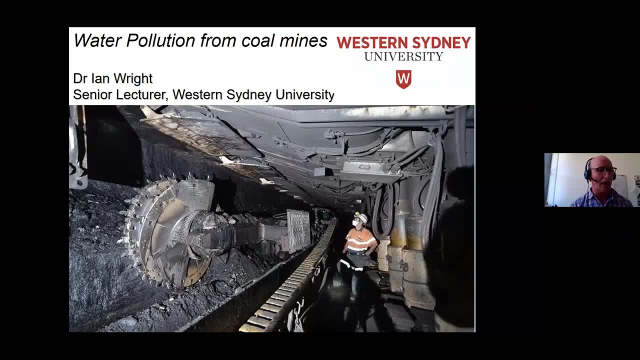 the map of the world. So I'm going to talk about coal mining. I've got a big interest in coal mining and it's been going for more than 20 years now. It's not the only thing I do. I'm a water scientist. 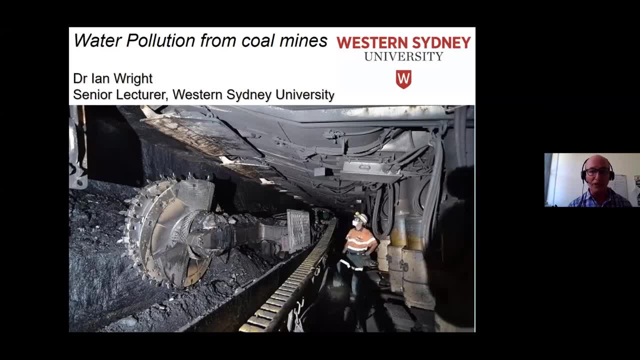 with a background in the water industry, I'm now an academic. I'm still a bit involved in the industry. but water and coal- people don't always think of it together, But there's a very, very close link. Here's a view of long wall coal mining which is completely revolutionising. 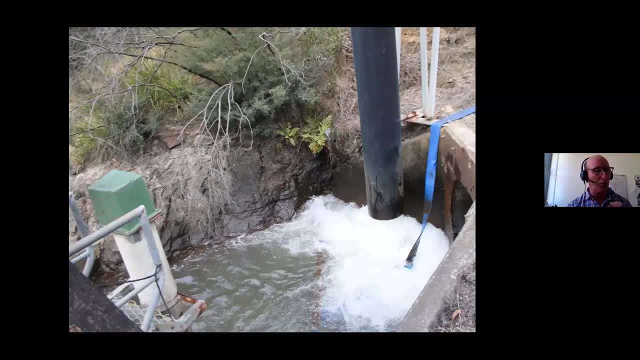 the way of underground coal mining, But it's water. Here is an outlet for one of the mines that I've studied. This is the Clarence coal mine and it might be counterintuitive to people but when you dig a big hole in the ground and mine coal and they dig huge holes, There's 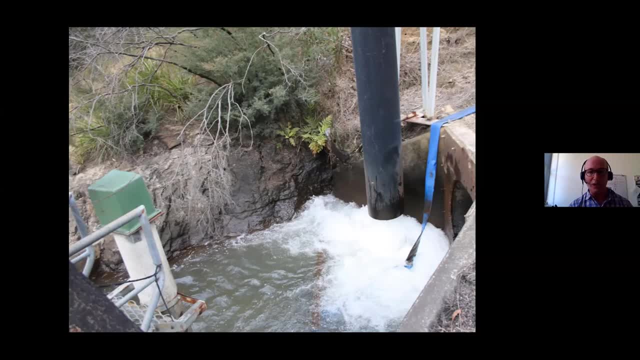 huge voids, whether they're roadways or long walls, but infiltration from groundwater seeps in and it's a huge area that's mined underneath and so you've got huge seepage And this is a discharge point. That's actually the licensed discharge point from a coal mine. 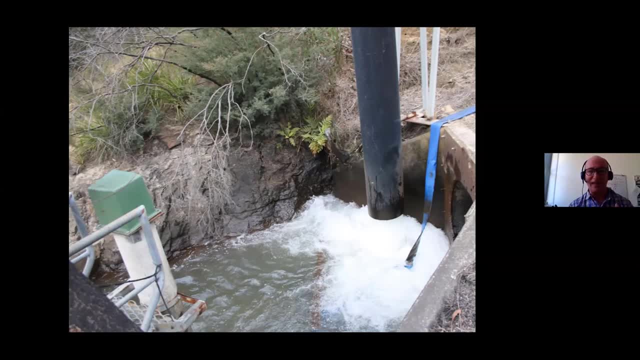 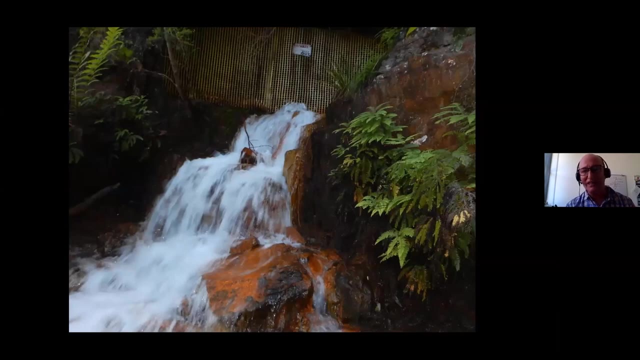 What's the impact, What are the issues associated with this? How is it monitored? What's the impact on the environment? How is it regulated? I'm going to talk about all those aspects, Cover it, not in a lot of detail, but here we go. So here for me is: this is why I do this work. 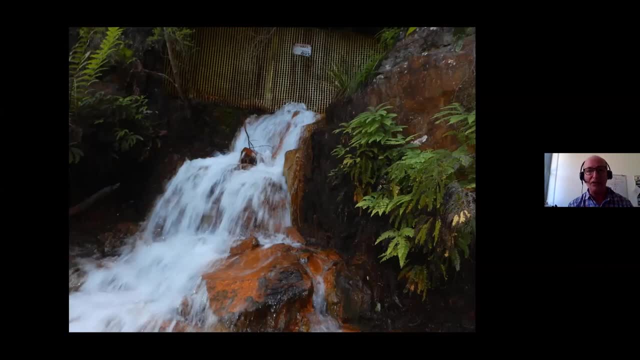 This is the first mine that I became concerned with. It's the Kenyon coal mine and this is a drainage adit. I last visited this probably about six months ago. I've been visiting it for on and off in different ways for 20 years. That mine shut 22 years ago, April 1997. the Kenyon. 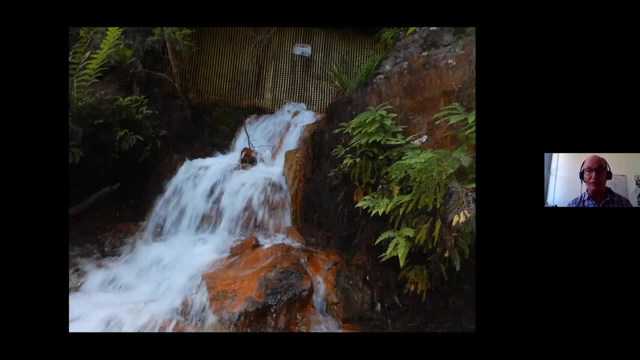 coal mine shut But water still roars out of it. There's two drainage adits. Look at those colours you see on the rocks. That's not natural. Why is the drainage still coming out? Because the coal mining has changed the layers of earth. that's cracked and water infiltrate in filters. but 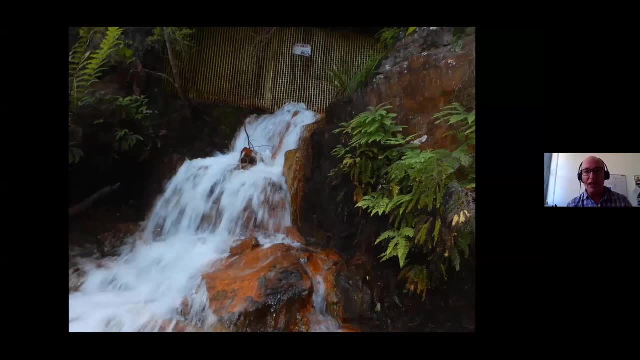 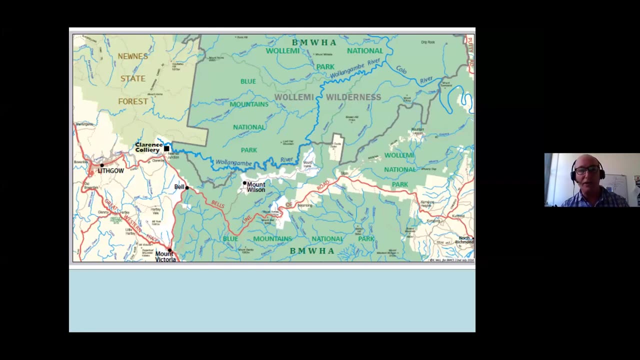 but it's probably also cracked streams and swamps above it, and now heaps of water continues to flow through. Where are we? Here is a map. We're in the Western Blue Mountains, so west of the Sydney CBD in Southeastern Australia. 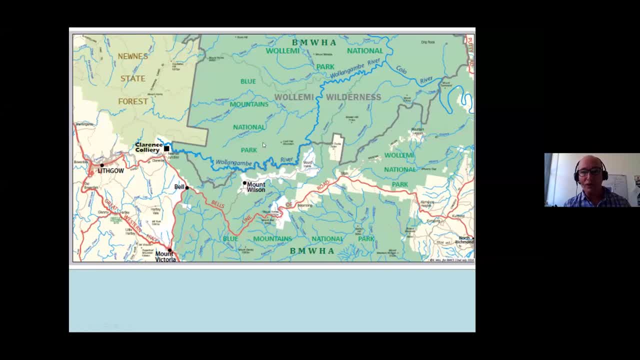 and this is the Blue Mountains National Park and the Wollemi Wilderness. It's also a declared wilderness area, It's a declared wild river and it basically ticks every box in terms of environmental significance. But you'll see this little red box appear. 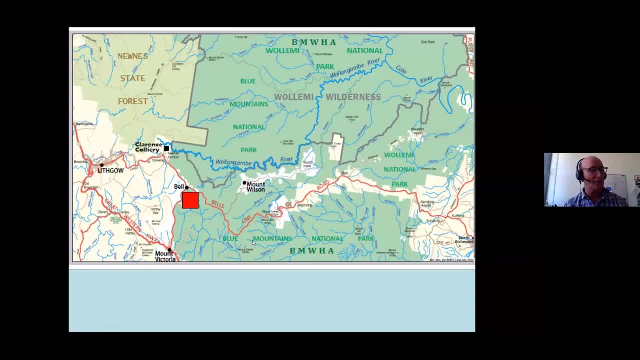 That is the workings of the old Canyon Coal Mine up at the top of the Grosse River. This was started 70, 80 years ago. If you wanted to cause an impact and put a coal mine, you'd put it there. National Park wasn't declared. 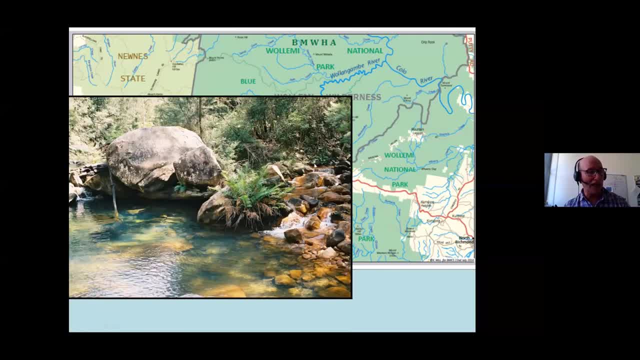 This is what it looks like today. So that's contamination that comes down. That's about a kilometre downstream from the mine, and then it hits the Grosse River. This is one of the most valuable and significant rivers in a conservation estate in Australia. 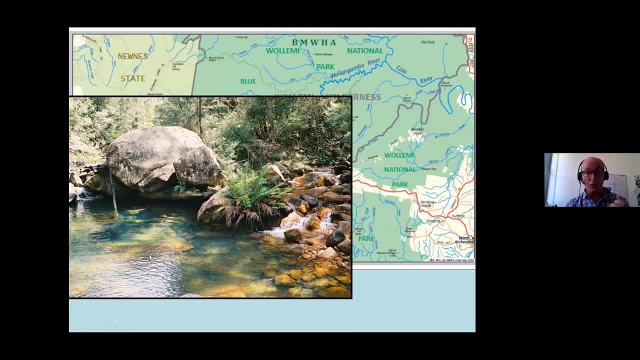 It can flow all its length from above 1,000 metres all the way down to the tidal area of the Hawkesbury Nepean. And look at those colours. I'll talk more about the metals that we see appearing in this stream. 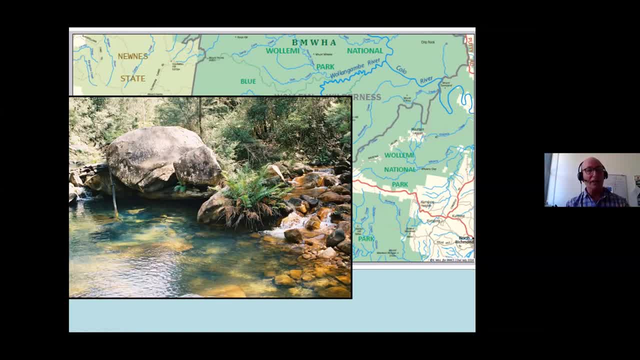 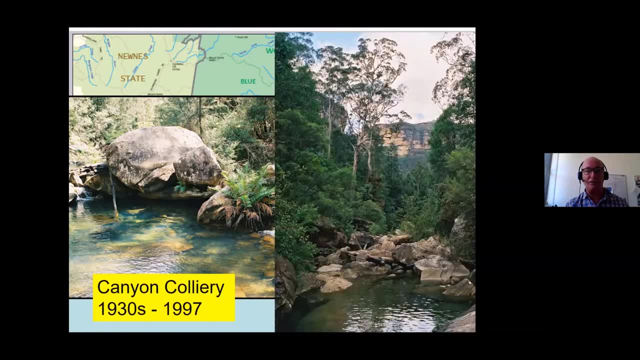 but we're in the middle of a high conservation value area. Mining's left but the impact remains, So it was called. the Canyon Colliery ran from the 1930s through to 1997.. And here is a view in the upper Grosse River. 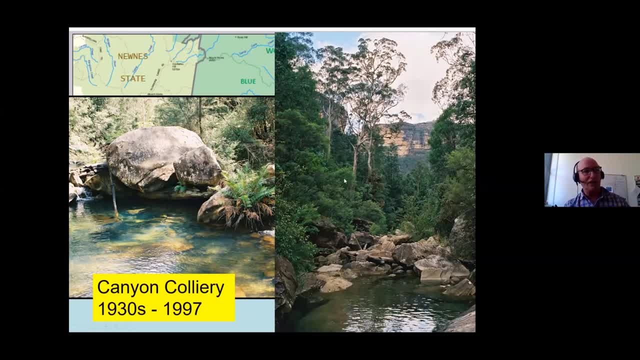 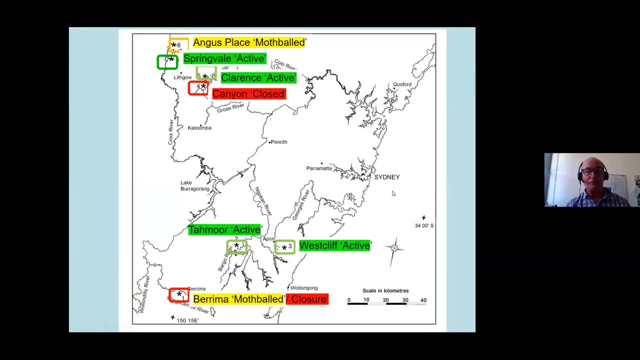 looking just above And where my icon is, there's actually a contamination comes from a stream and flows down into the Grosse River here. But this is just one of the mines I've been studying over the last 15 years. I've colour-coded them. 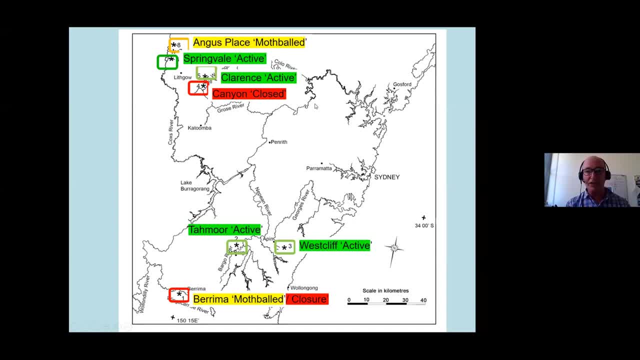 This is the Sydney Basin: Sydney, Parramatta, Penrith. This is sort of the Sydney metropolitan area- five million people underlying this. This is the Sydney Basin: Sydney, Parramatta, Penrith. This is sort of the Sydney metropolitan area- five million people. 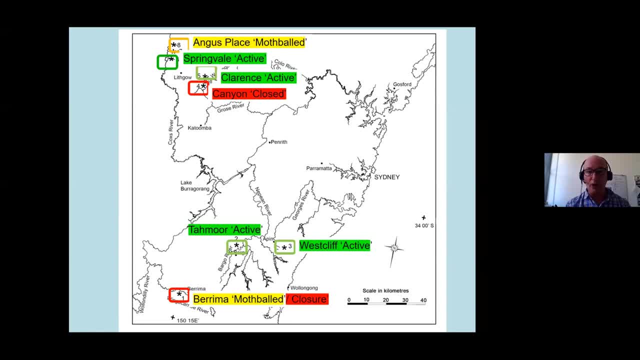 This is the Sydney Basin, Sydney, Parramatta, Penrith. It's an incredibly valuable coral resource. Some of these coal reserves are very low ash, very low sulphur, so they use for steel making. others are thermal coal. 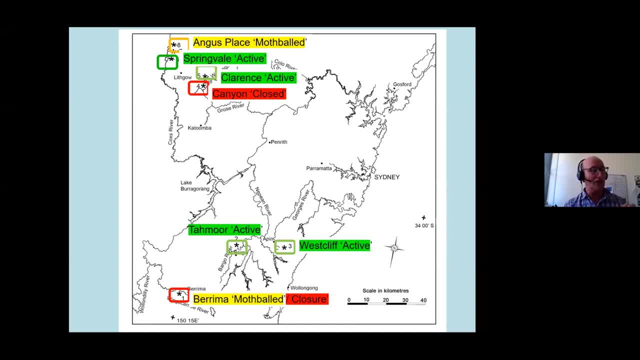 and this extends right above this area. Now I've colour-coded this: Red is closed. yellow is mothballed, or care and maintenance. green is active, so it's actively mined. The Canyon mine is closed. The archives of mine at the bottom is mothballed. 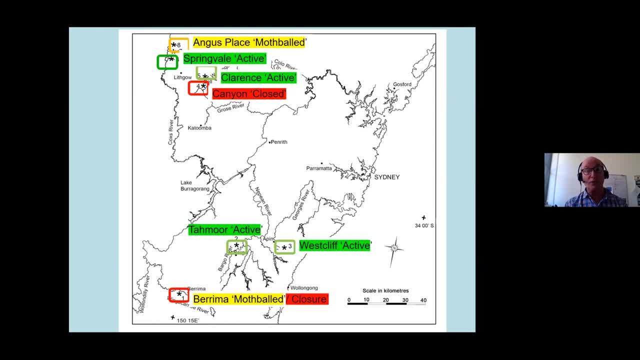 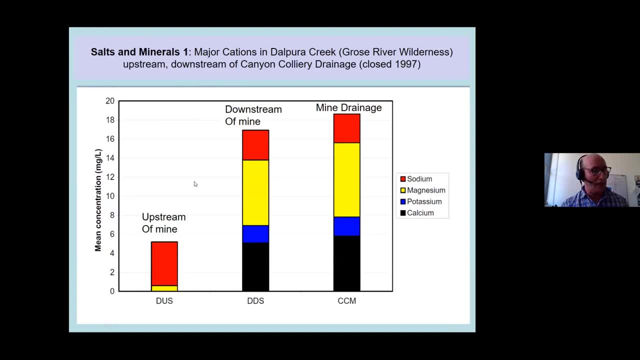 actually in the closure process, and Angus Place at the top is also mothballed. that's called care and maintenance, so it's ready to be opened. What are the impacts? I'm first going to talk about water chemistry and some pretty straightforward stuff. Major cations: sodium, magnesium, potassium, calcium. 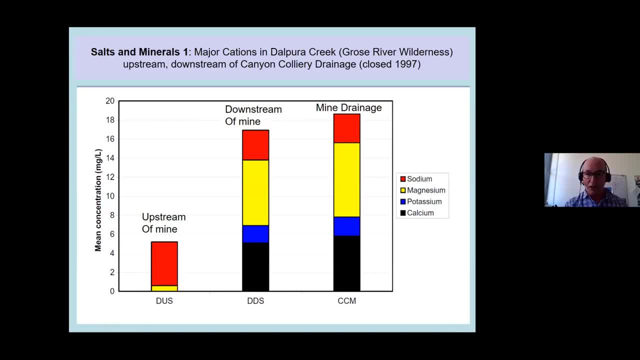 Upstream of the mine to the left, you'll see it's mostly in this bar graph: sodium, little bit of magnesium. This is the natural geochemistry of the streams in the Sydney Basin that's very clean. but then downstream of the mine and further to the right, the mine drainage. you see we've changed that sodium and a little. 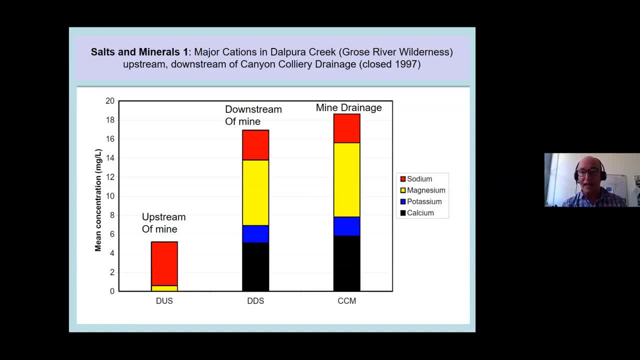 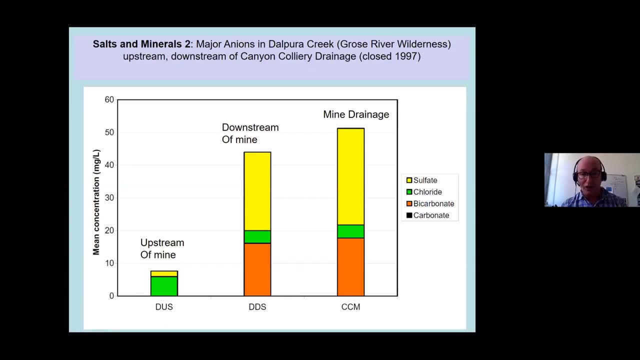 bit of magnesium. it's now magnesium, potassium, calcium. We've changed the ionic chemistry of the stream completely from the mine drainage. So that's the cations, the anions, in many ways, for me much more interesting. So it was chloride dominated upstream. 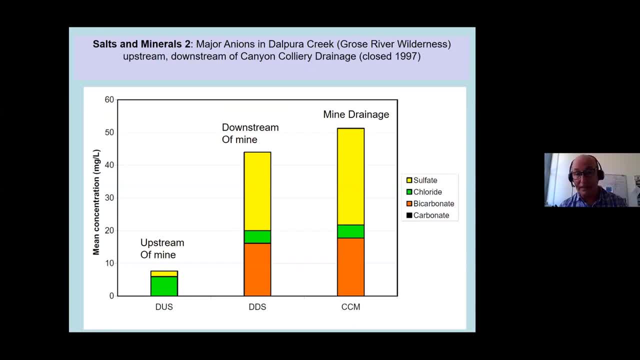 downstream sulphate. Sulphate to me in Sydney Basin is a real indicator. If you've got a sulphate dominated stream, there's a high likelihood that's associated with coal mining. So the sulphur mixed with oxygen and water in the mine and that creates sulphuric acid Gives some indication of those. 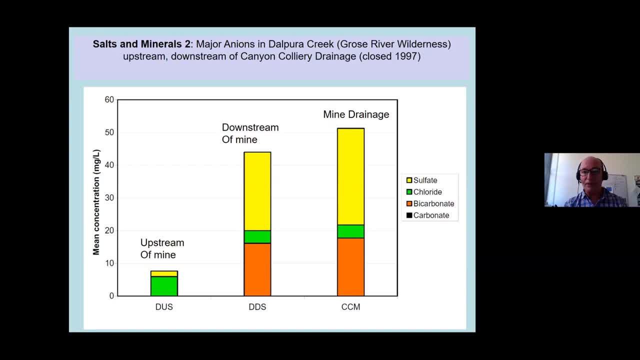 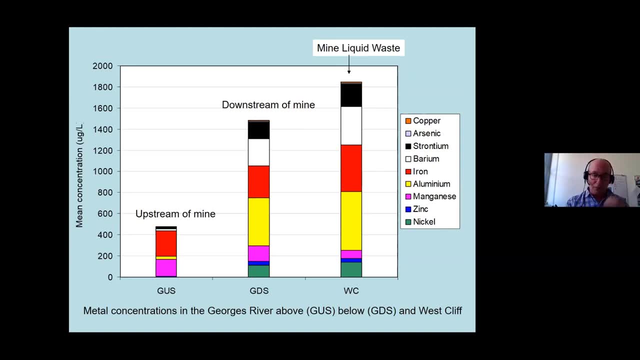 underground geochemical processes. We've also got carbonate and bicarbonate, and we're talking also about solder, Gaia and coal also. So, yeah, what's that do? It drops the pH. and I'm looking at another mine. this is the George's River. 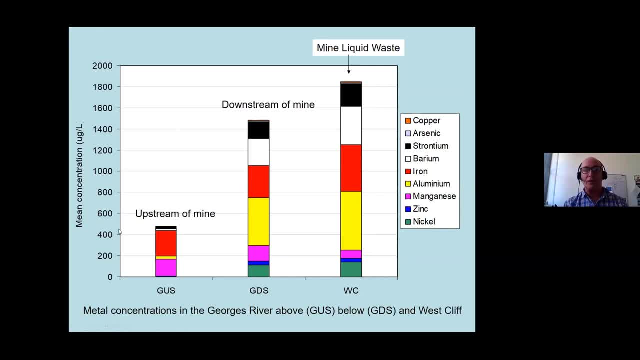 and the Westcliff mine is actively mined upstream. A snapshot of the major metals. So we see three in particular: iron, aluminium and manganese. that's the orange, the yellow and the purple or the magenta colour. That's Sydney sandstone. 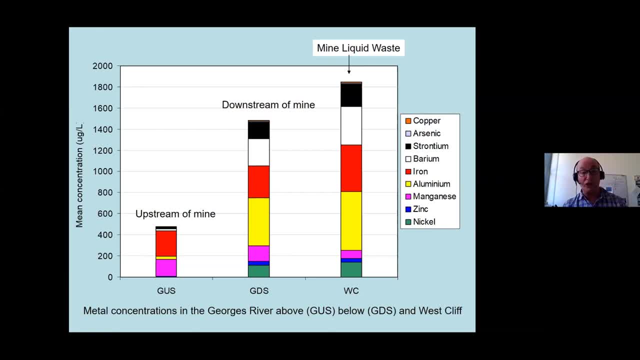 the typical ochre, orange and yellow colors, but when we look at the mine liquid waste, we've got a whole series of other things. pretty much everything we look for in a periodic table turns up. we've got copper, arsenic, strontium, barium, zinc and nickel, as well as the iron. 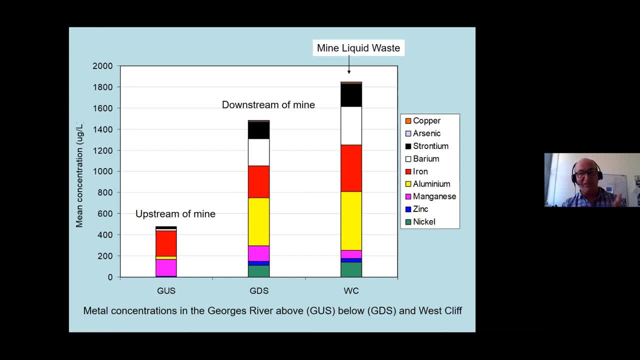 aluminium and manganese, for me straight away. strontium barium- that stands out. that's often associated with coal mines and the residue from coal mines in the sydney basin. but as an aquatic ecologist i'm looking at down the bottom: the blue and the green. zinc and nickel- they're the ones. 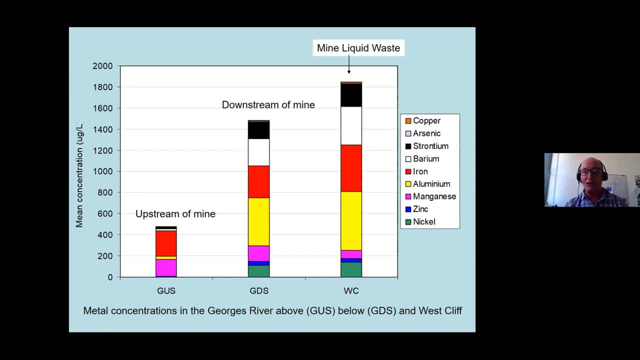 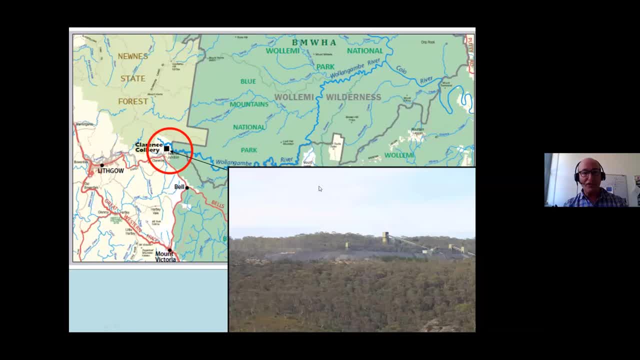 a lot of coal mines and we've got a lot of coal mines. we have the clarence colliery. i've circled that and i've pointed to the surface workings. so this mine is currently active. it's actually working under state forest but it's so close to the boundary and this in australia, is a very, very famous national park. it's also part of the blue mountains. 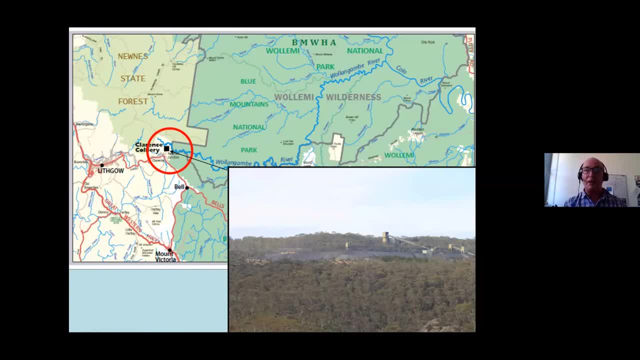 international park. it's also part of the blue mountains world heritage area and it has one of the living fossils that was only discovered about 20 years ago, called the wallet- myself leading an undisclosed world heritage area- and it has one of the living fossils. it was only discovered about 20 years. 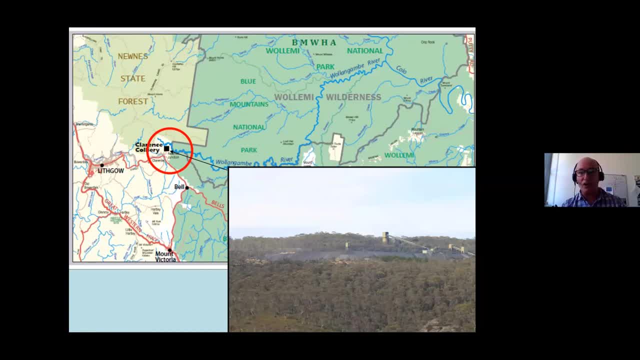 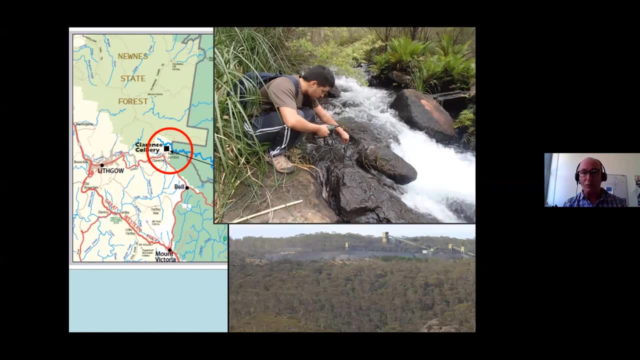 location somewhere in this national park. So what's this coal mine doing to it? Here's a view of a former student looking at the Wollongambi River just downstream of the discharge point from the Clarence coal mine. Already you can see the bottom of that stream. It's got a lot. it's very, very. 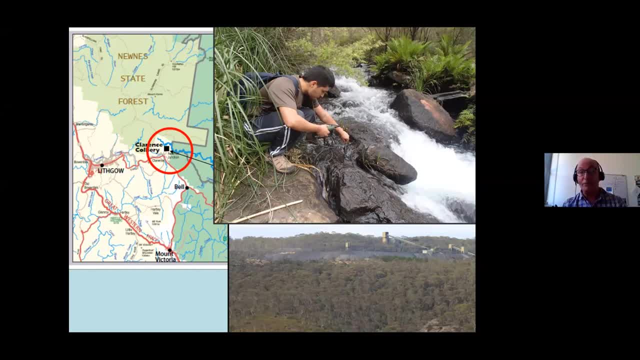 dark. The mine drainage makes up about 90% of the Wollongambi River, which actually flows into National Park and the World Heritage Area about 10 minutes of flow. It's about about a kilometre from the mine outlet. So zinc is one of. 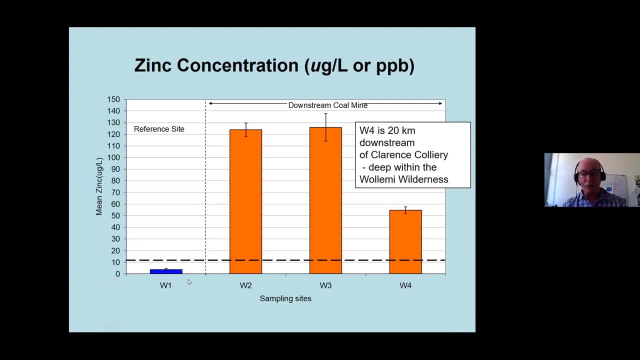 the things that concerns me, and so look upstream: W1, that is in the Wollongambi River, That's the average zinc level above the mine, and then W2 is below the mine discharge. W3 is about the point that it goes from State Forest to 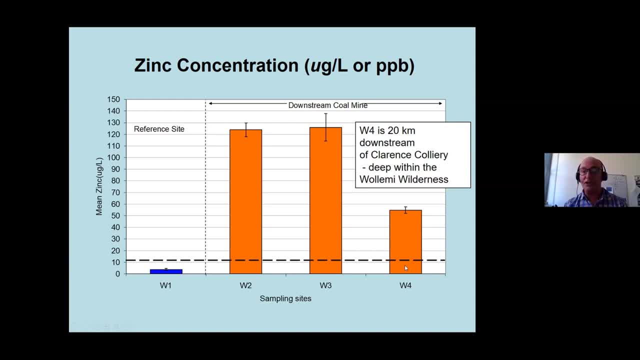 National Park W4 is about the point that it goes from State Forest to National Park. W4 is 20 kilometres downstream, So we're deep in the wilderness area, deep in a high conservation value area, really the highest you can get. It's World Heritage. 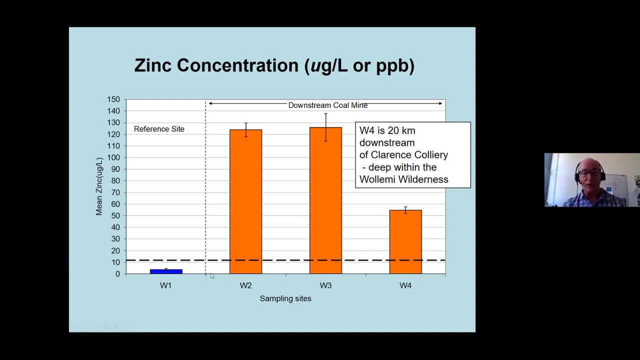 Look at the zinc level. Zinc and nickel are both pollutants here of concern. The dotted line is the Australian guideline. Above that dotted line it is stressful for an ecosystem. Look at that. 20 kilometres downstream It's still way above. That's originated from the coal mine. 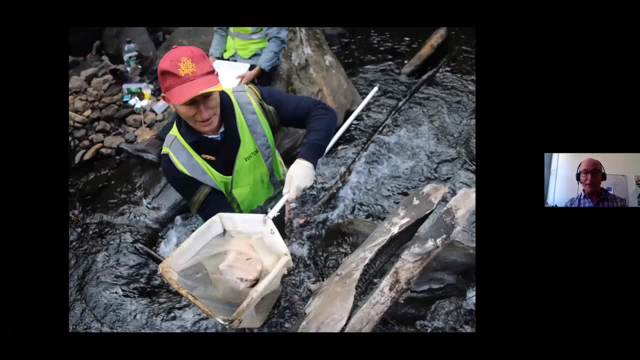 So here's a picture of me, Hello everyone. That's me jumping in a river. I'm the youngest of five kids. I was frequently called to as a kid: go jump in the river. Now I do it professionally. There I am. I'm using a hand net. I've 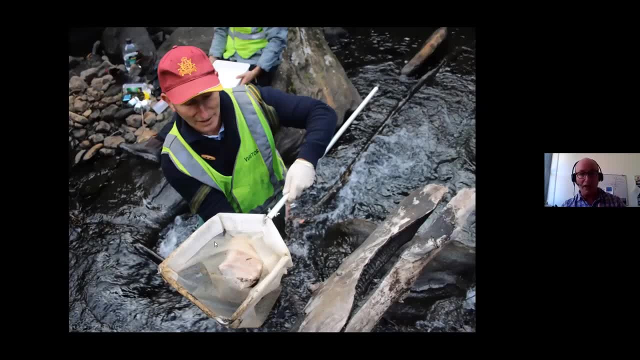 just put that down the bottom of the river. I've stirred up the sediment That is the Wollongambi River. I'm about to pass the contents over to my trusty assistant behind me, PhD student Nakia Belmont. Ah, G'day, Nakia. 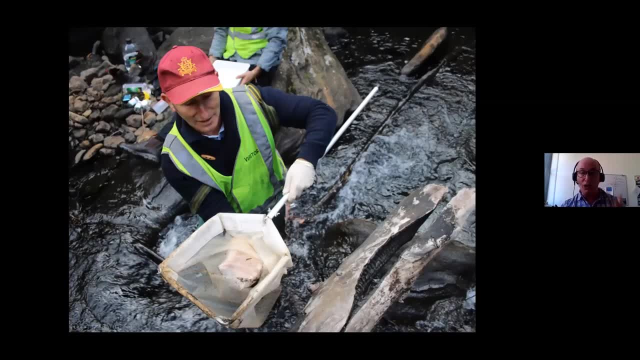 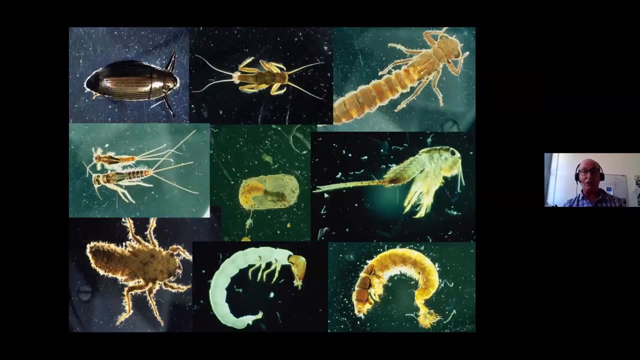 So I've got the contents of my net. The question I'm asking here is: what is my net 3, 2,, 3, 3.. here is: what impact is that coal mine discharge having to the ecosystem health of the river? I get my net contents and I look for animals like this, If anyone's. 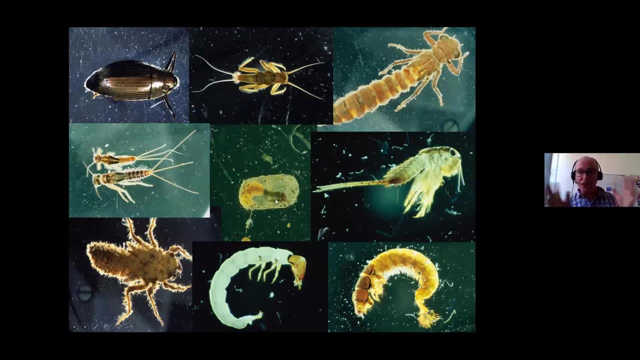 familiar with the Brady Bunch. I call this my Brady Bunch photo. this just gives you some idea of the kaleidoscope of animal life in the bottom of rivers in the Sydney Basin. Up the top right we've got a giant larvae of a dragonfly. 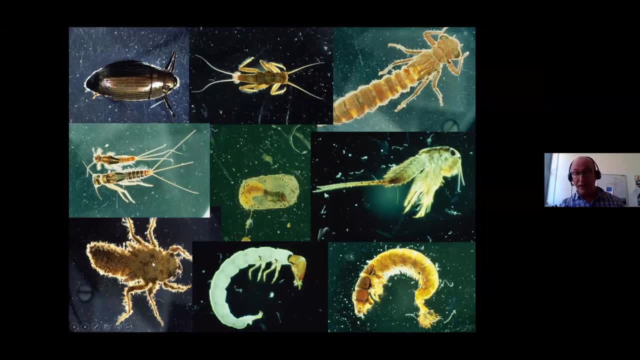 Bottom left. that's a different species of dragonfly. It's covered in silt and hares and that's a stealth predator. We've got beetles, stoneflies, mayflies, caddisflies, kaleidoscope of life. What impact is that discharge of the canyon? 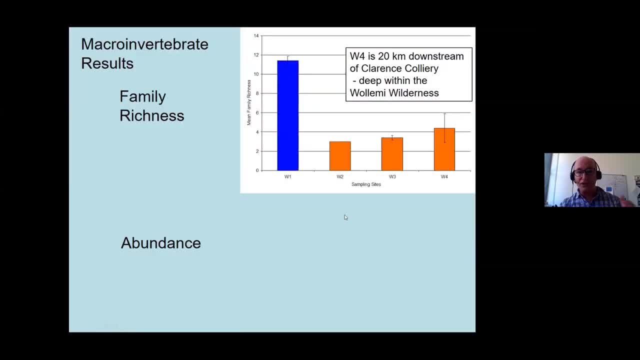 coal mine. having Looking at the family richness- so that's the number of different invertebrate families, W1,- we had an average of eleven and a half families Downstream. that dropped Down to about 320 kilometres downstream. It's just above four. So that's just. 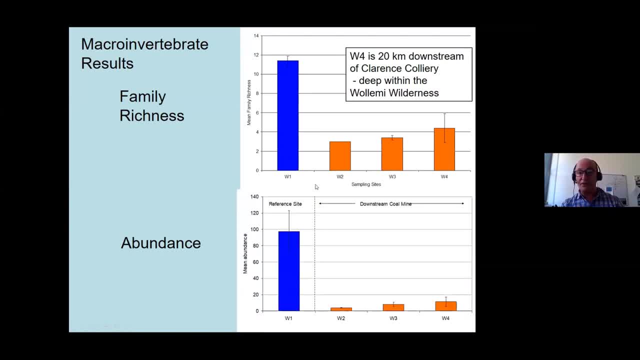 looking at the diversity, the number of different families, the abundance of animals that drop from a mean of just a below a hundred animals. in my net downstream It's about 90 per cent less W4, 20 kilometers. In conclusion, we're affecting the diversity of aquatic. 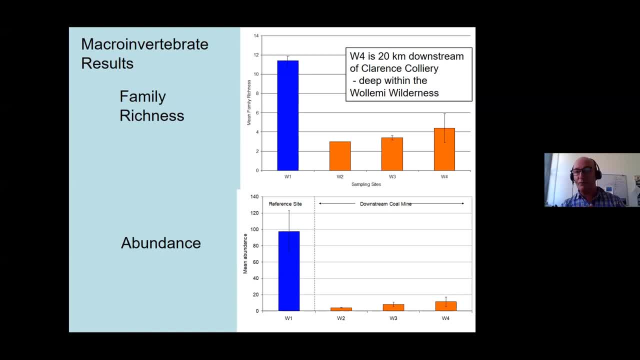 animals. we're affecting the abundance. Now remember these invertebrate animals. these are the fertilisers source for lizards, for birds. We've got platypus living in these waterways, unique to the Australian biodiversity. This coal mine is having an adverse, major adverse effect on the biodiversity of the 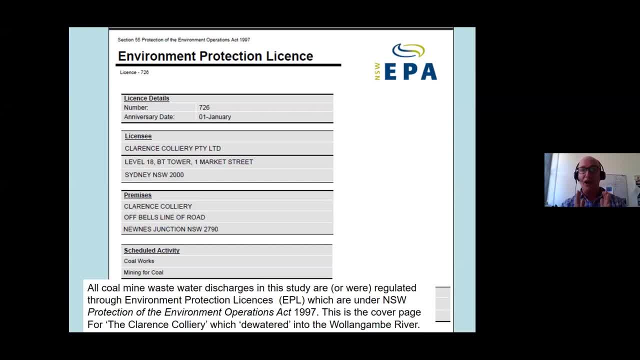 river. How do we regulate this? It helps if you've got a law degree As a scientist. I've had to get my science in and understand how the legislation works. In New South Wales the legislation is called the Protection of the Environment Operations Act. Here's a licence for that. mine, the Clarence 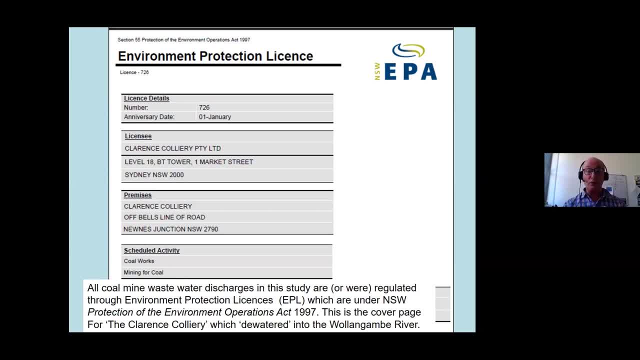 Coal Mine. It's about 25 pages and it's full of conditions. This is called an Environment Protection Licence, has a unique number- licence number 726, and that is how this is regulated. As a scientist, we have to get safe levels in here to literally achieve this: protect the environment. 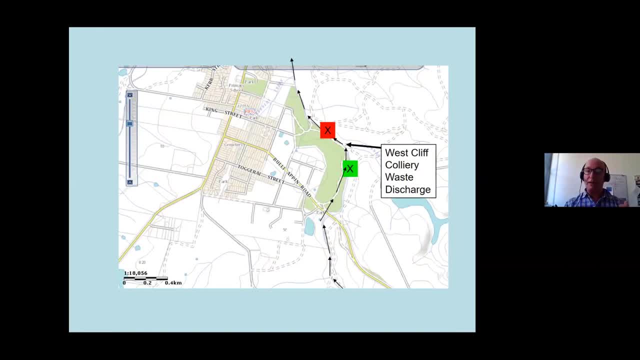 I'm going to display that now. demonstrate it through another coal mine. So we're now down on the Cumberland plain, closer to Sydney. This is a map view of Appin, and so green is upstream of a mine discharge and this is actually the Georges River. It's one of the big rivers that flows into the Sydney CBD. 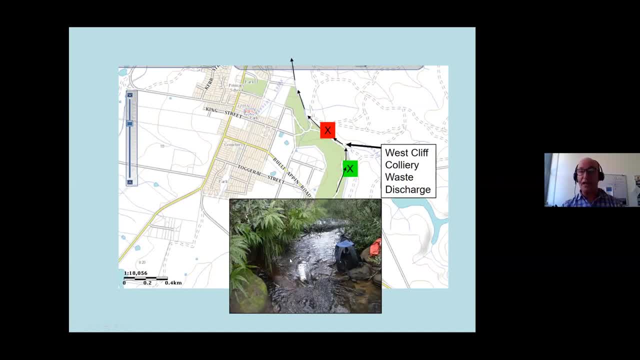 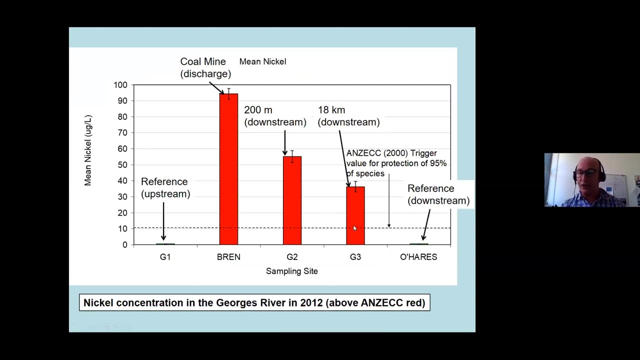 in a place called Botany Bay. That's upstream. this is taken on the same day and that's downstream. You can just see that turbidity. there's also more flow From the Westcliffe mine. that's the waste discharge, and here I'm looking at the nickel. I collected this data in 2012.. I 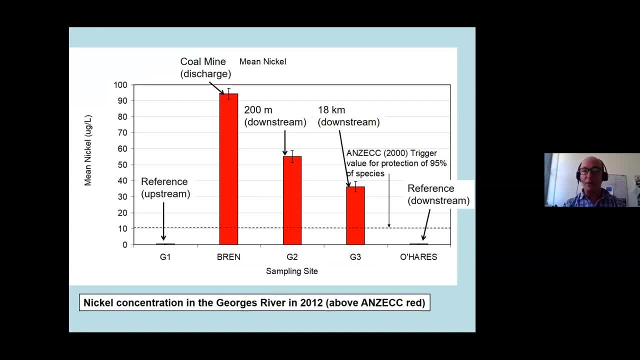 actually collected this for a court case. The mine at the time was owned by BHP and the local National Parks Association and the Macarthur Bushwalkers took BHP to court. They're a big miner. The mine's now owned by South 32,, which is Spud. Let's look at the nickel. here It is. 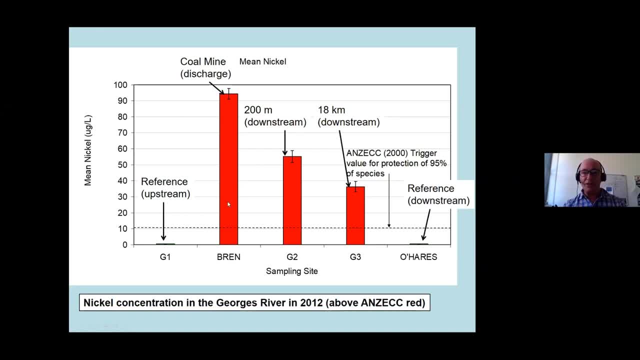 upstream, almost undetectable, Brennan's Creek is the tributary containing the coal mine waste, The dotted line, the safe level. Look at that level Again. 18 kilometres downstream, way above the guideline, We've got a reference creek downstream. Huge nickel levels, Unacceptable. 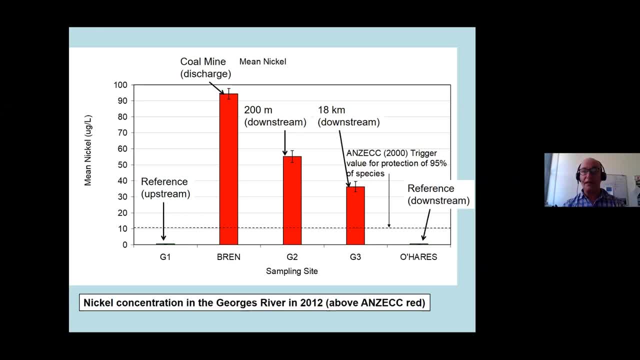 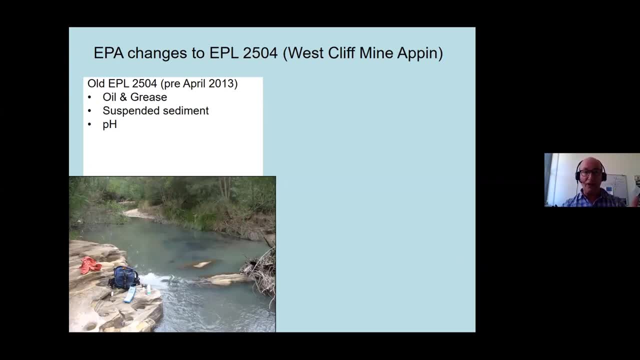 There was also an environmental ecological impact similar to the Canyon mine. So the conditions for discharge contained in that licence- the EPL Environment Protection Licence- that was number 2504 prior to the EPL, That's the EPL Environmental Protection Licence that was number 2504 prior to the EPL. 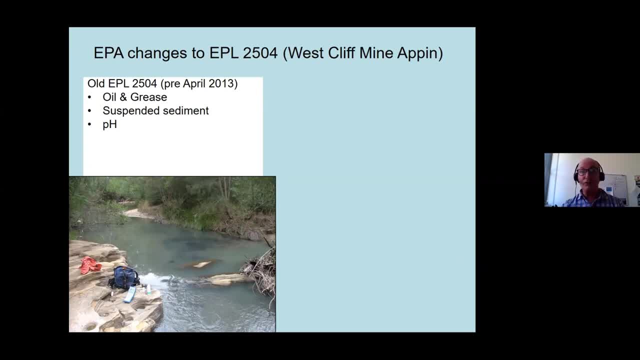 So the conditions for discharge contained in that licence, the EPL Environment Protection Licence, that was number 2504 prior to the EPL After April 2013,. there were three, Three: Oil and grease suspended sediment pH. That was all, Yet look what was coming out. Look at that turbidity. 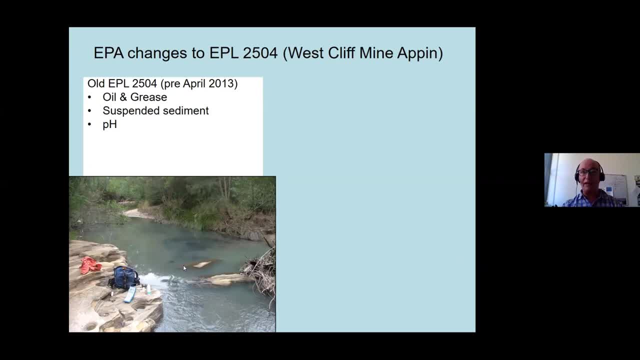 We didn't have conditions for any metals yet. they were coming out After April 2013,. these are the new conditions. We've actually got discharge limits for aluminium, arsenic, copper, nickel, lead and a whole series of others. How did that happen? We did the science. We were in a 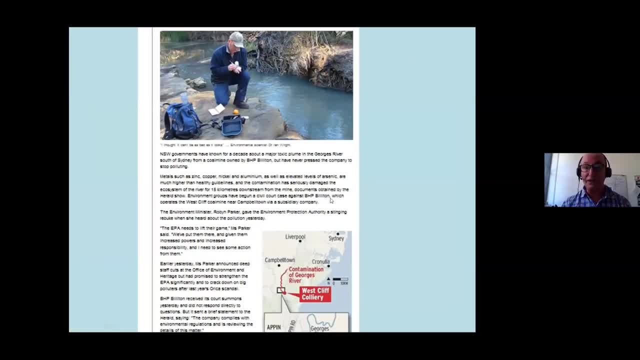 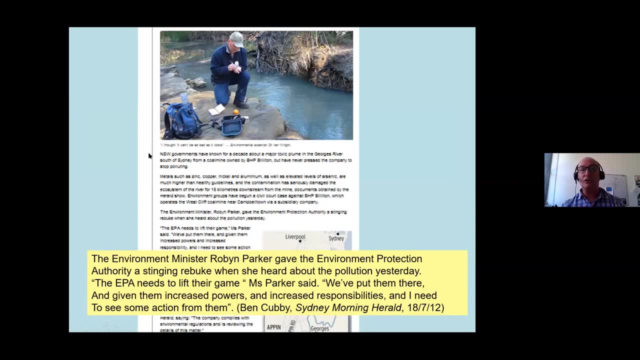 court case. This is what happened. Now you can't read this, so I'm just highlighting a couple of bits, but it's actually a picture of me. My sister said that she looked at the Sydney Morning Herald one morning and there was a picture of her brother. She said that wasn't a nice way for. 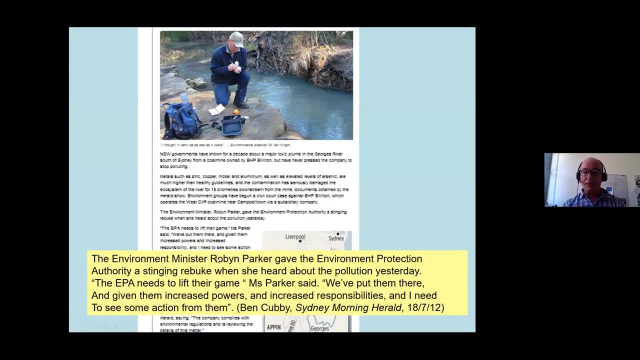 me to have breakfast, Anne. But here's a highlight: The Environment Minister, Robin Parker, gave the Environment Protection Authority a stinging rebuke when she heard about the pollution yesterday, Front page of one of Australia's top papers. basically, this got action. This was the Environment Minister of New South Wales. 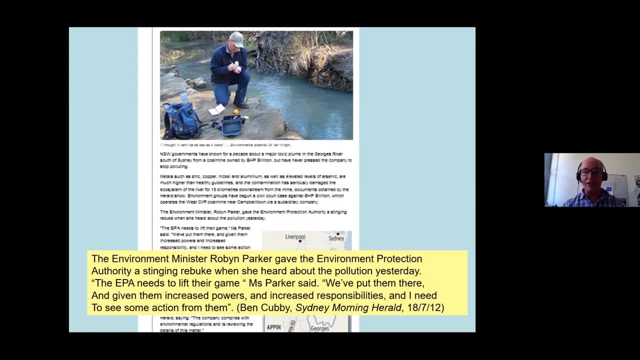 They encouraged the EPA and BHP to talk, now South32, and they improved their licence. So you need science, you need policy and law, but media helps and politicians. But what happens after a coal mine shuts? Here's another one. This is looking at the 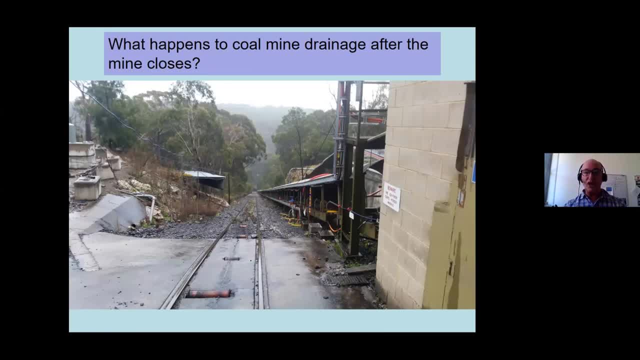 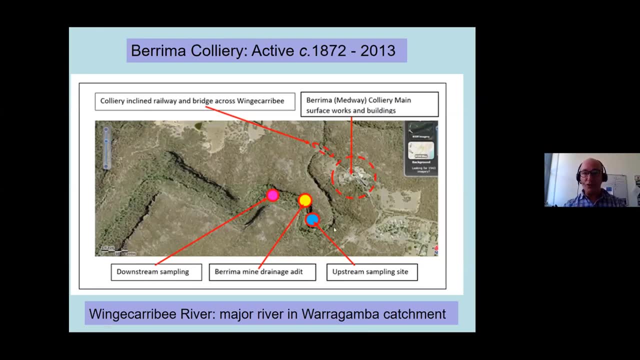 Berrima coal mine down the inclined railway down to the mine shaft. There's conveyor belt leading up. Here is a view. This was Australia's longest-running coal mine, from the 1870s, shut in 2013.. It's in the closure process And I'm going to show you some photos of what part. 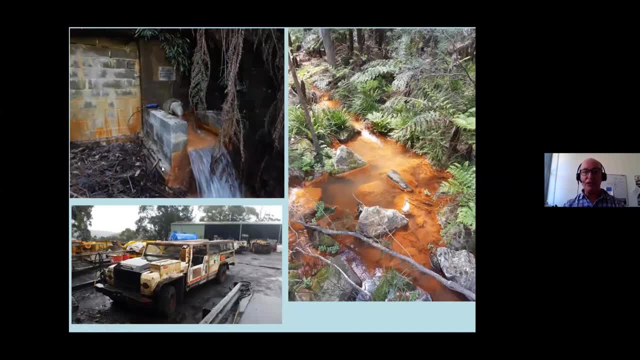 of this looked like after the coal mine shut. Here we have the drainage at it which was sealed, but only partially sealed, Basically, so people couldn't get in there. The drainage still came out. And look on the right, Look at that- ochre ferric discharge. 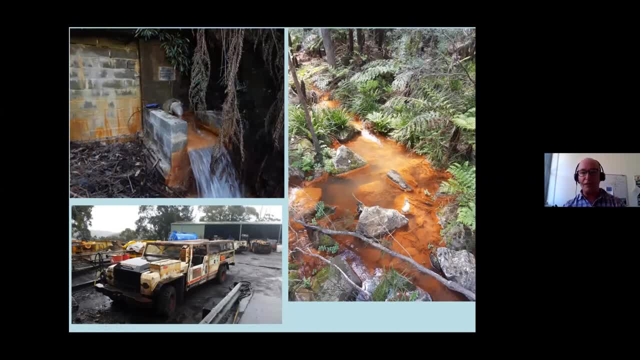 Metals oxidised. They then fell to the bottom of the stream. There was some machinery that was dispersed. This was owned by Boral, who have been good partners and have shared information with me through the closure process. We've got some data here On the left, the pH of the mine. 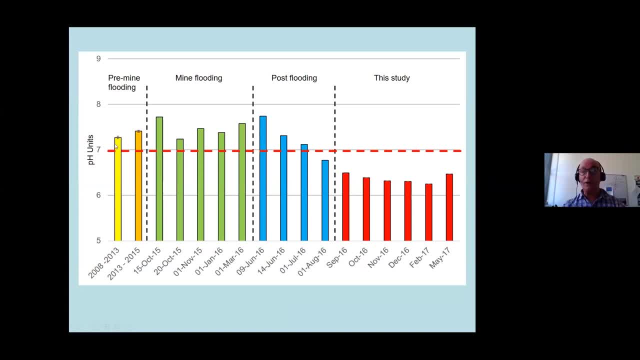 while it was operating, 28 to 2013,. it was mildly alkaline. They flooded about 15% of the mine. After the flooding, the pH dropped. So basically this mobilised sulphur, it went acidic and then that started to leach metals- Not huge negative pH. 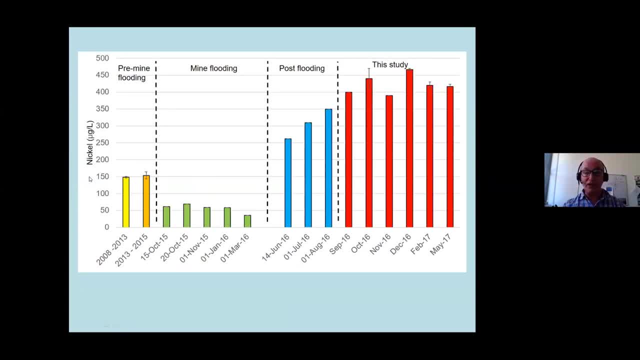 but it was mildly acidic. It's enough to make something like the nickel. Look at the nickel level: It was 150 micrograms. As it flooded it diluted, Then it shot up after the flooding because the pH had dropped and we had mild acid drainage and then very high level of nickel. 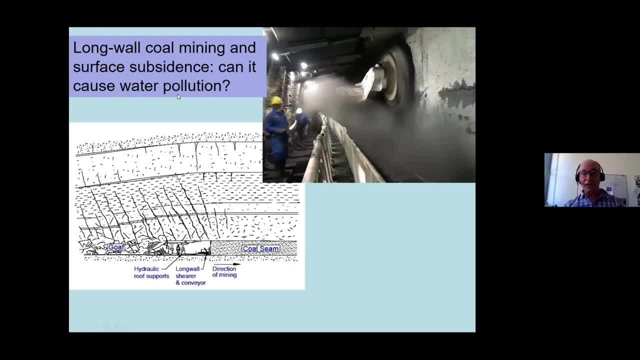 downstream of the mine. So that's what can happen After a coal mine shuts. again. getting back to long wall mining: Long wall mining: they take out the coal seam, Then we get fracturing of the land above and the strata. 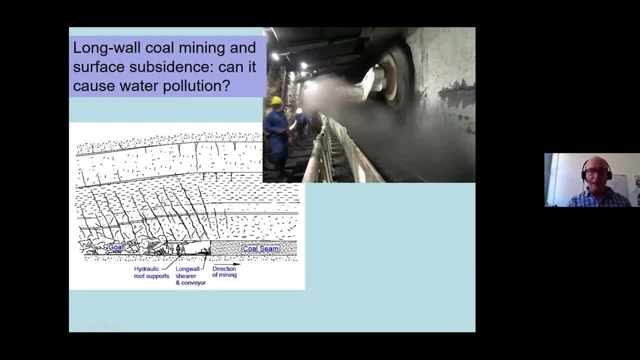 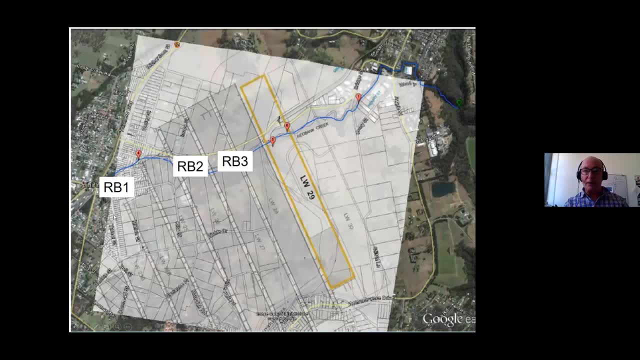 above. See all those big cracks. What can that do to a waterway? Let's have a look. Here is a study I did in the southwestern area of Sydney, in the Cumberland area. This is Redbank Creek. I've studied this creek for years and these are long wall passes, So the long wall is actually 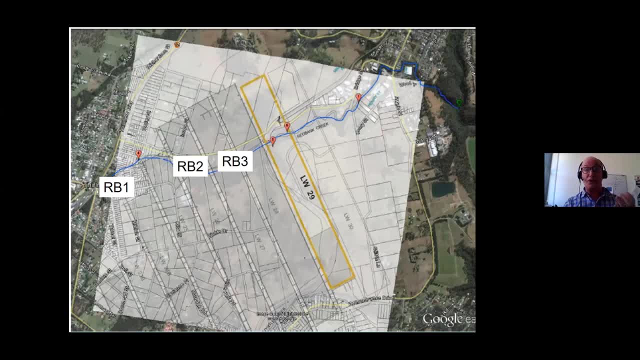 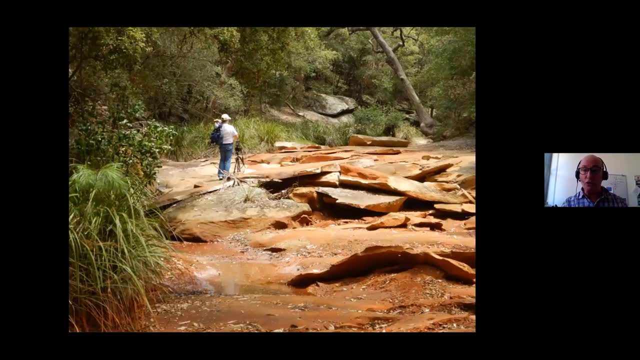 about 400 to 500 metres under the surface. What happens? What does it do to a creek? All kinds of stuff goes on. Check this out, Look at that creek. This creek has not been bombed. That is what they call abstinence. So as they took that layer of coal out, the whole landscape dropped by about a. 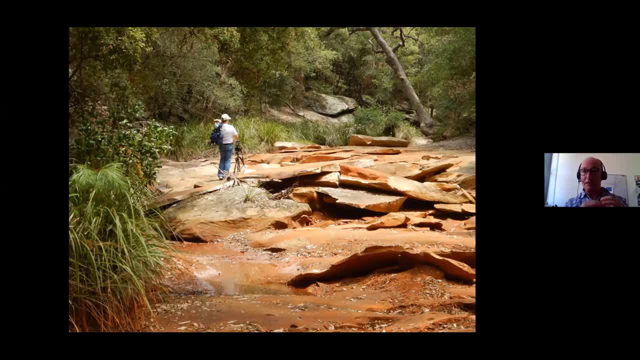 metre, but some areas didn't drop as much because there wasn't as much pressure above it, And that's often in a V-shaped valley. The creek is not as much pressure above it and that's often in a V-shaped valley. The creek is not as much pressure above it and that's often in a V-shaped valley, The creek. 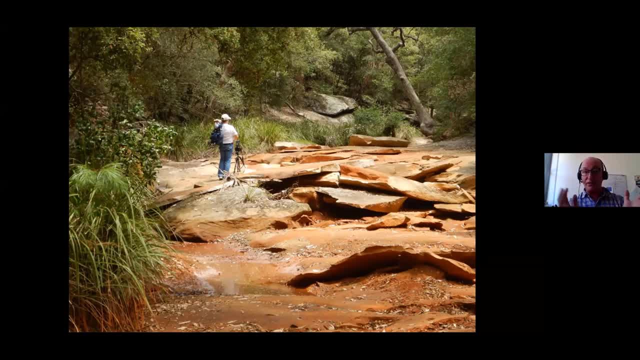 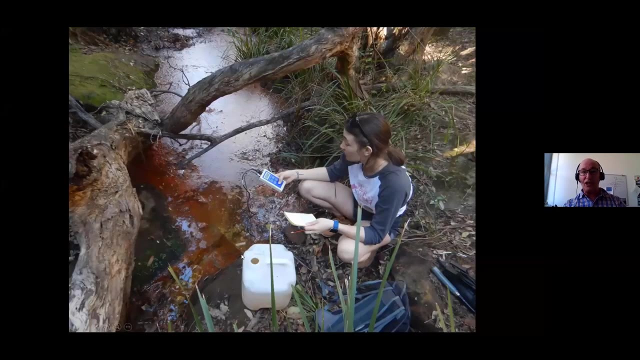 itself lifts up in relative to the land around it. It's called abstinence. Look at the cracking, the fracturing, the lifting, the warping, the twisting. Number one that doesn't hold water. well now, but you can see a bit of this ochre-like contamination And one of my last slides. 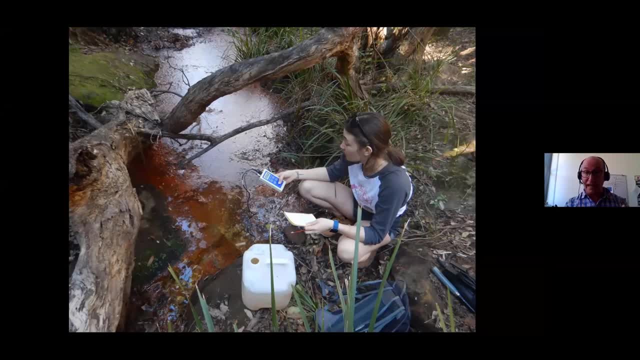 this shows water coming out. It's actually cracked an aquifer for a while And there I have a student gathering data. There was actually no oxygen in this water and it was oxidising on the surface and that was then stripping out the oxygen, oxidising metals, which then dropped to the 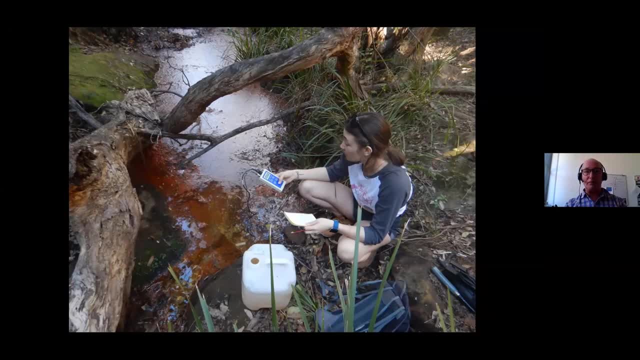 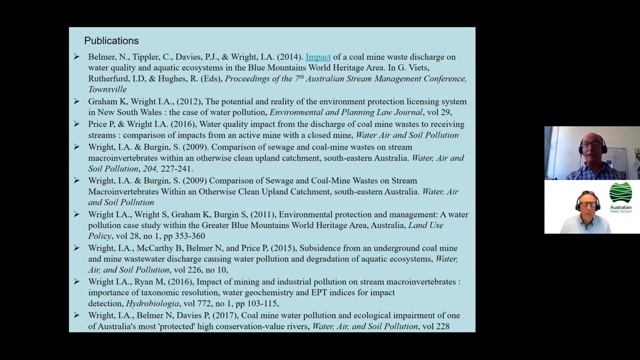 bottom. All kinds of impacts: high metals, low oxygen, high salt. It's complex, It has ecological impacts and that's coal mining in the Sydney Basin. I've got lots of publications. I've given some here, but I'm happy to have questions. Trevor, how was that? 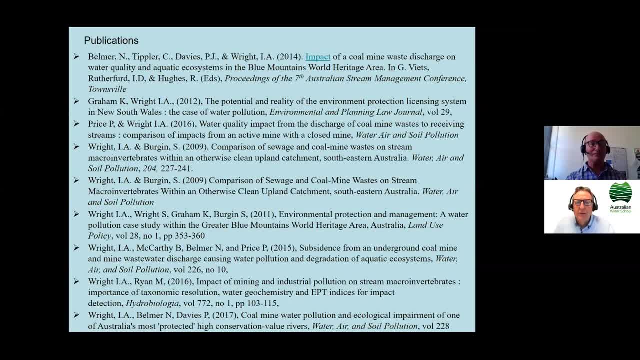 It was great, It was good. I've got lots of questions. I'm happy to have questions, Trevor. how was that? It was great, It was good. I found it to be something you could follow. well and very clear. I said earlier in the 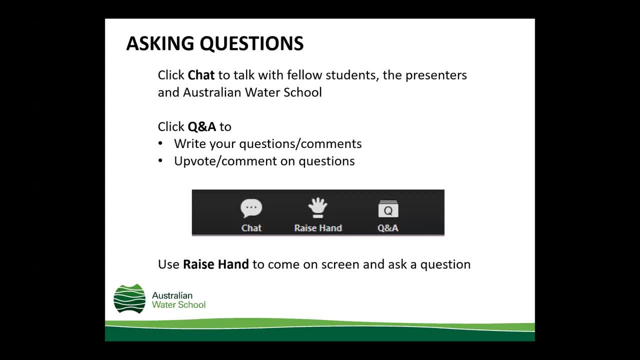 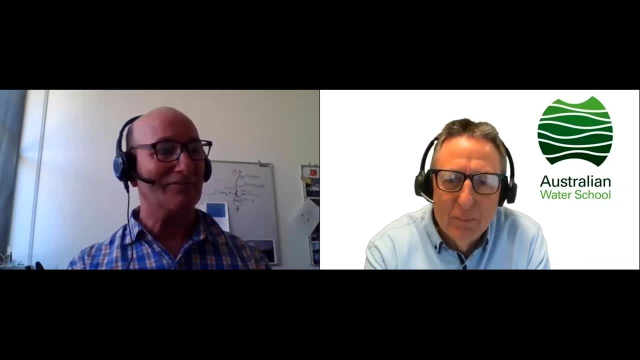 chat line. brilliant, clear presentation And I can see the questions are starting to come through. Fantastic. You've done a lot of work on all this and had a lot of people involved, And I love your quote: go jump in the lake or go jump in the river. 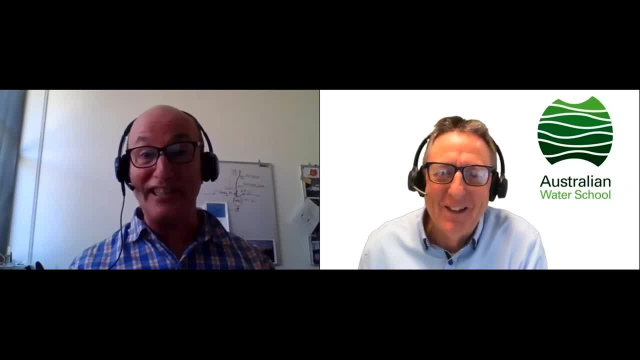 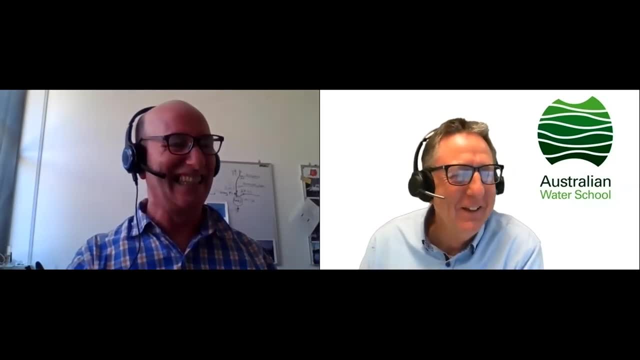 which is exactly what you're doing for a job. It's great, I get paid for it. now It's great, It's my revenge. You get paid for doing what you've got hit by the last of five kids. I know that feeling. Why don't we get started with these? 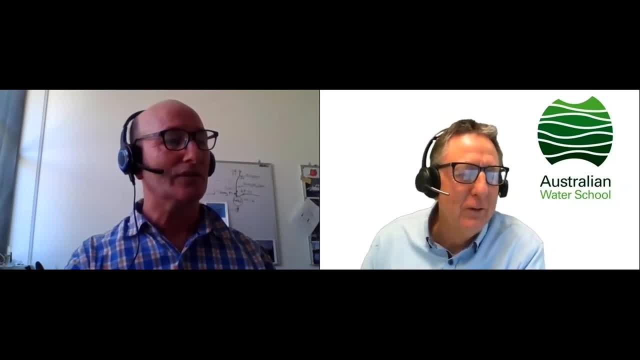 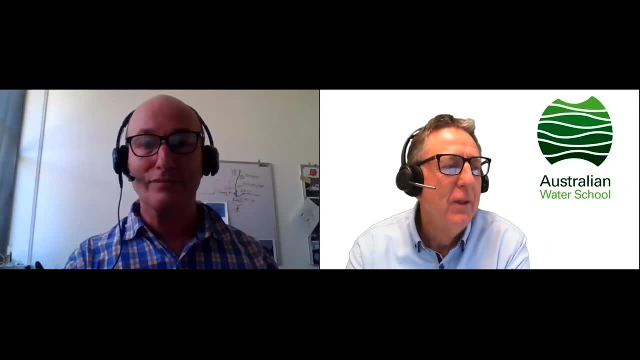 questions And everyone. thank you, You've started putting in questions and discussion. That's really great. Keep them coming. That'd be fantastic, But Pat Ridley has asked: maybe it would be good, Ian, if you hit your Q&A icon so you can just read along that with me. 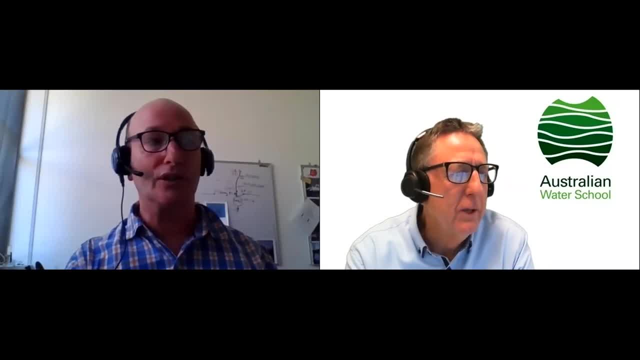 Oh, yes, See it there. Yes, I do. The top one there has now been uploaded and there's a few more questions coming in, So let's keep the answers reasonably brief. But here we go. How are legacy issues managed after mine? 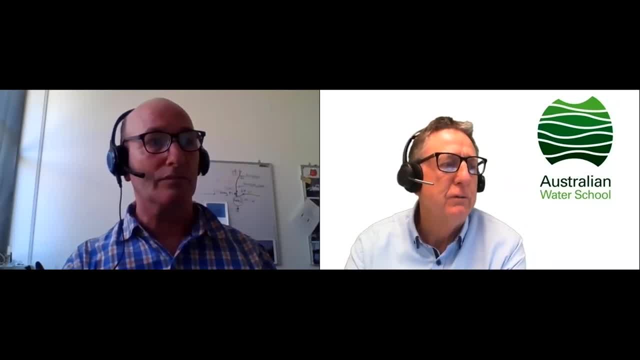 closure. Many mines expose acid sulphate soils. Mining companies leave after mine closure and leave contaminated mine voids. How is this managed? Oh, that's a great Thank you. Thank you, Pat. That's a great question, Probably. how long has it been a string? 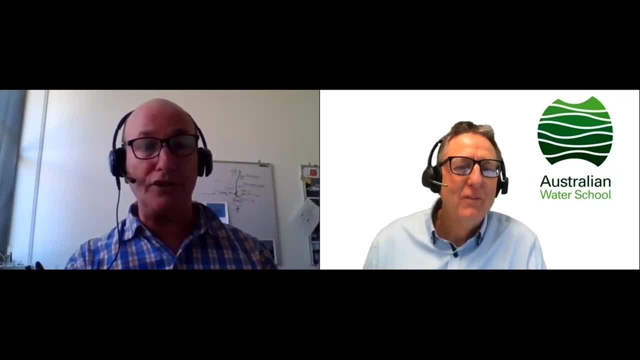 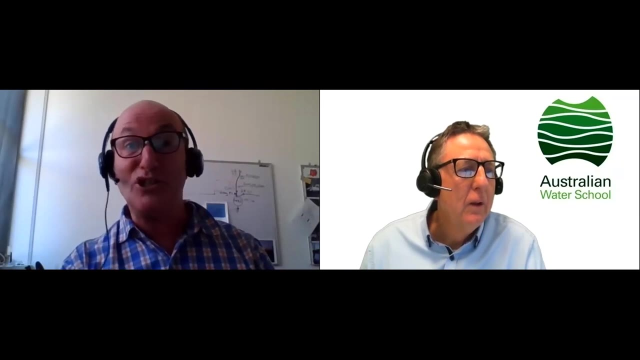 Absolutely And we really have the full extreme of the two ends. The Canyon coal mine- that miner has walked away. Industry regard that as a disaster, both the regulators, consultants and the miner- And that impact is left for future generations. When I'm teaching, 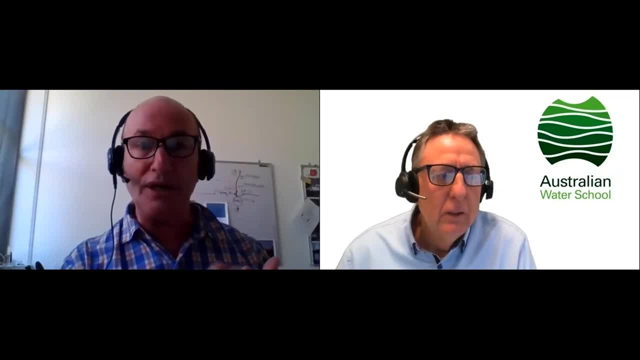 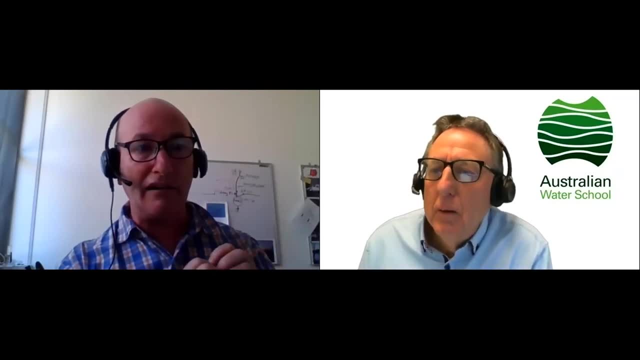 students I say you're going to have to deal with that. We're not. But then look at the Berrima mine Boral own it. They haven't walked away. They've worked with me, with the regulators, and they are actually sealing that. They've installed a treatment system. 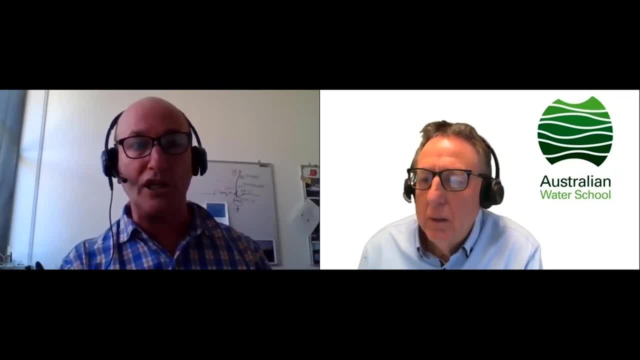 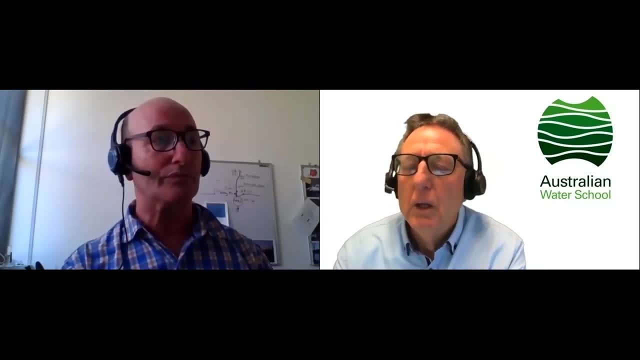 They've now sealed up the mine And I think Boral are establishing a new, a new benchmark, So I'm hoping that's encouraging the rest of industry not to leave a legacy issue. Thanks, That's really good question to now come and think fast, So we'll keep them moving. 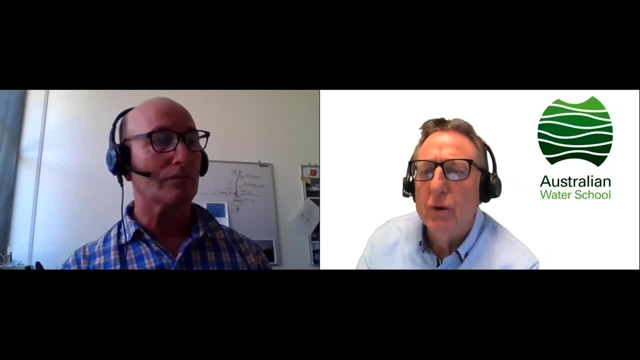 One here quite pertinent from David Harris and quite important: What are the key methods to radiate legacy contamination issues? And thanks, David, for your question. Great to hear from you and your high experience- long experience- in the area of water. What are the key methods to remediate legacy contamination issues and effects to surface water? 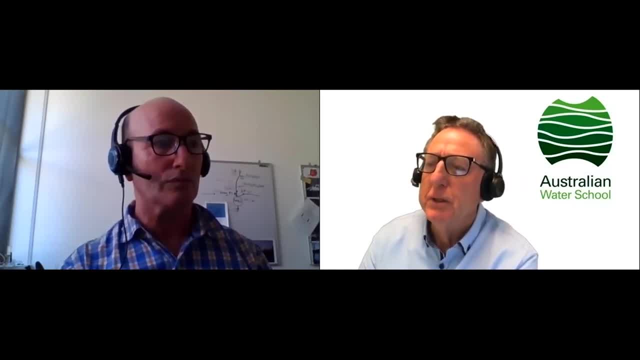 quality. Can soft engineering approaches be adopted to improve post-closure water quality on receiving waterways? This is a pretty key question. This takes time here, but it's a pretty deep question. Thanks, David. Look, that's a beauty. Look, I've got to say 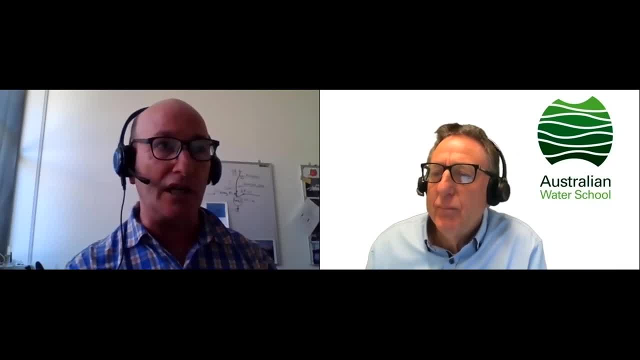 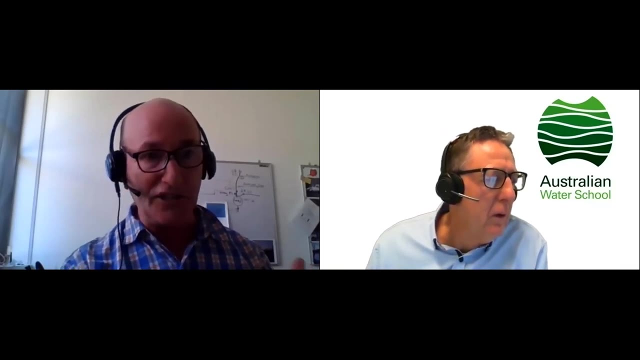 I've seen more answers to this really in the literature And I've seen a lot come particularly from the US, But the greatest literature I've seen is actually from the United Kingdom And because they lost so much of their coal mining industry and coal mines shut down in the 60s, 70s, 80s and 90s, I think there. might only be a couple of mines around. Honestly, many mines are not remediated at all. It's actually rare to have a full remediation. Look for underground coal mines. it's a bit different when you've got long wall mines. 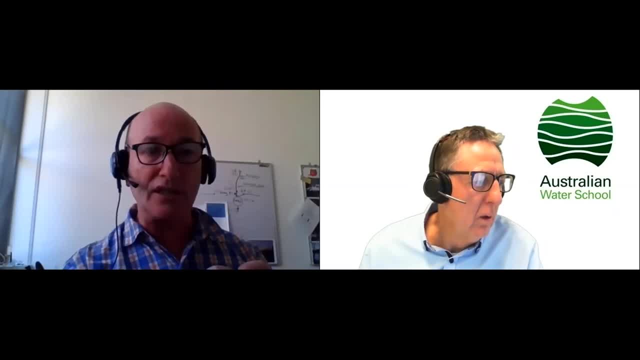 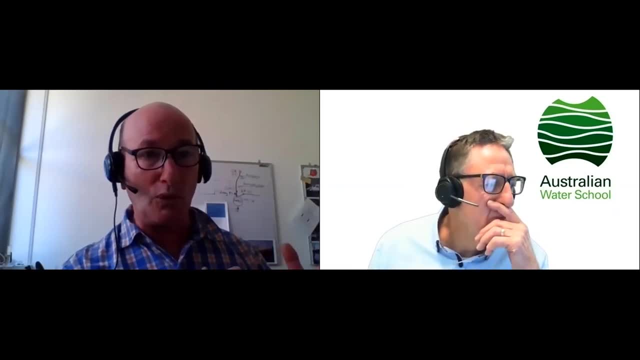 You've got long wall mining and you've got major disturbance, subsidence and fracturing. This is an area that's not well dealt with And I think a lot of the mines that are affecting waterways with fracturing aren't holding water well. 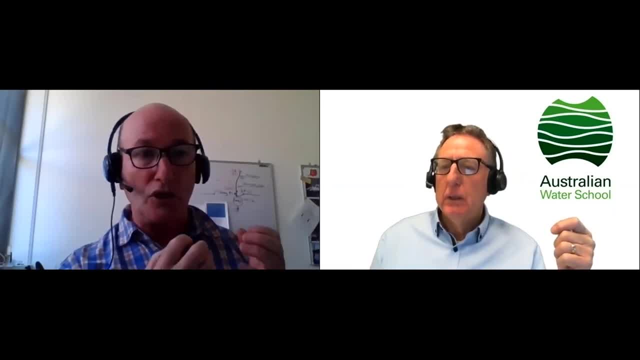 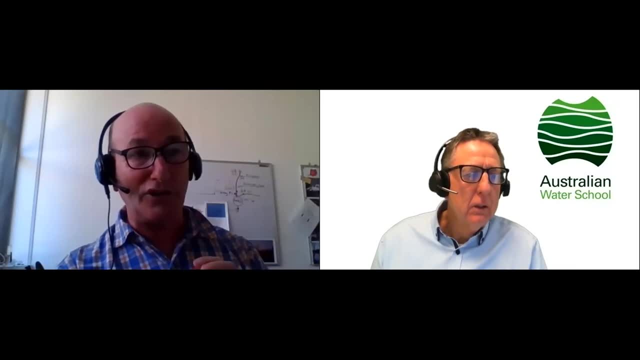 The mining industry and consultants are trying to glue them up, cement them up, grout them up, But a lot of the creeks still lose water. We've very dry continent. We've got a drought in Australia at the moment and that's a huge problem. 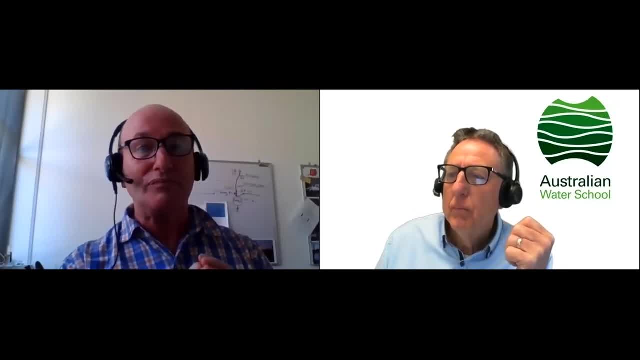 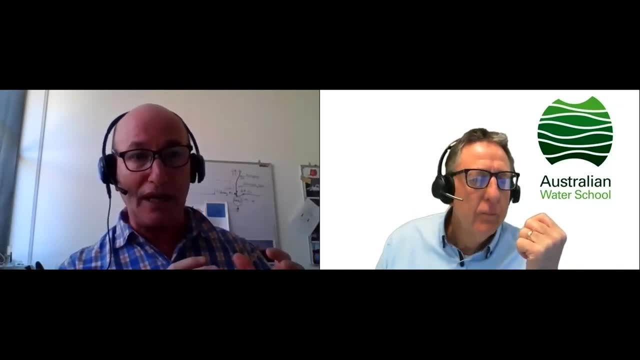 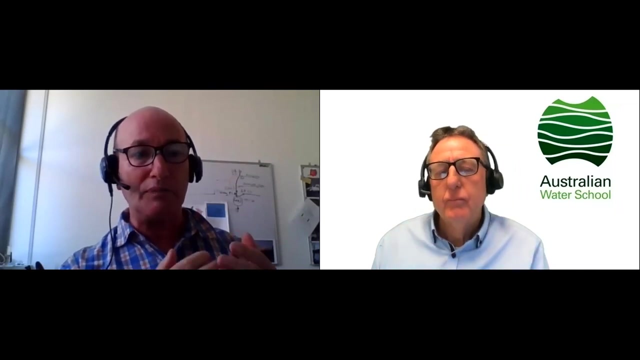 Soft engineering, yes, And I'm thinking particularly now about open-cut coal mines and reworking the disturbed areas, working with topsoil fertilisation and revegetating holding, preventing spoil heaps from being eroded and also controlling drainage and controlling the mobilisation of sulphur and acid mine drainage. 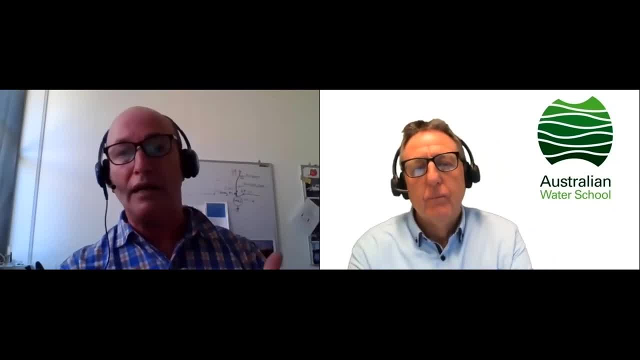 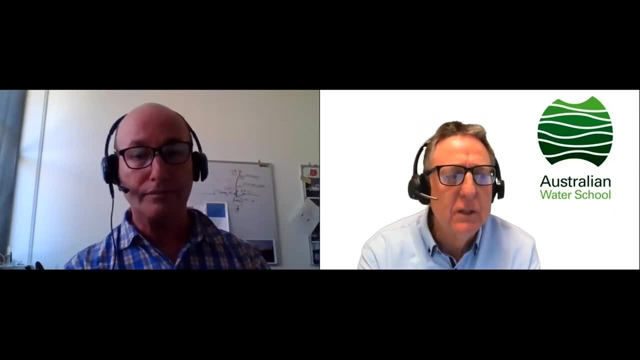 And yes, soft engineering has a big role. It's a complex area. I hope that covers that. Fantastic, Any follow-up to that, David, by all means. The other thing is: can we put on the chat line here? maybe my colleague Joel could put it up? 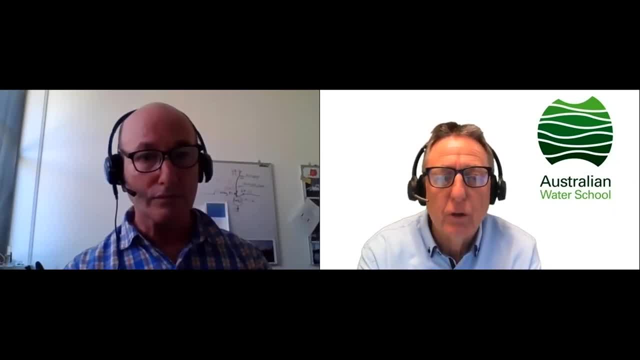 if you can recommend a website or a document that listeners, attendees, should go to. Is there anything in particular you could think of off the top of your head right now? Joel would certainly be able to put it up. You mentioned the UK. Yes, yes, They've got some incredible, incredible literature. 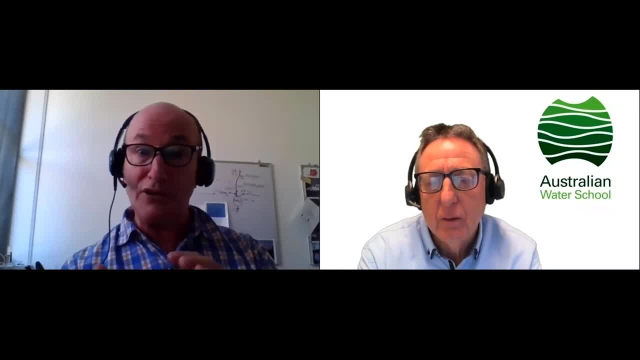 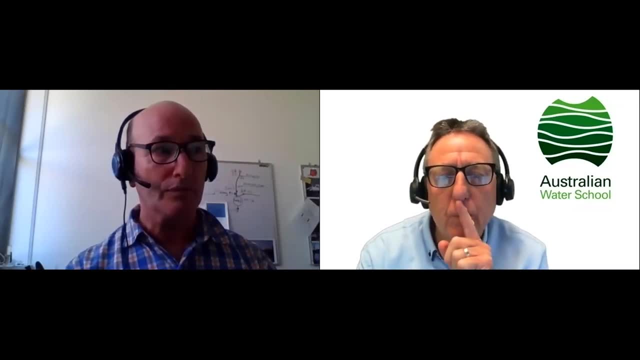 And they've also got a whole litany of problems and also successes. So I've really been quite impressed by the literature coming out. We can do it on the fly. Is there something we can look up right now and put it up for people to look at? 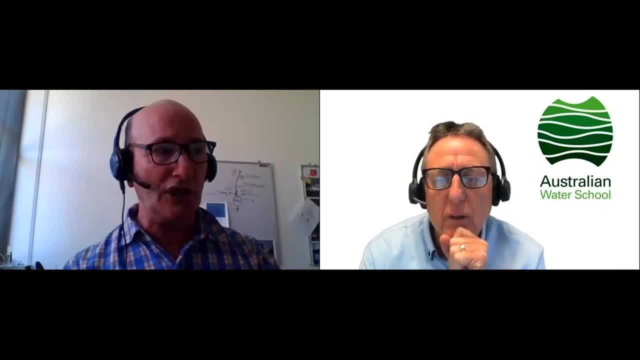 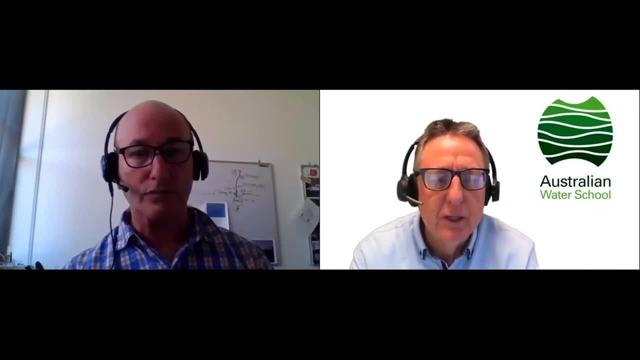 A website? Nothing I can think of off the top of my head. I'm sorry. That's all right. We'll send it out. when we send out the email to you, We'll send it out to all the registrants attendees. after the standby. 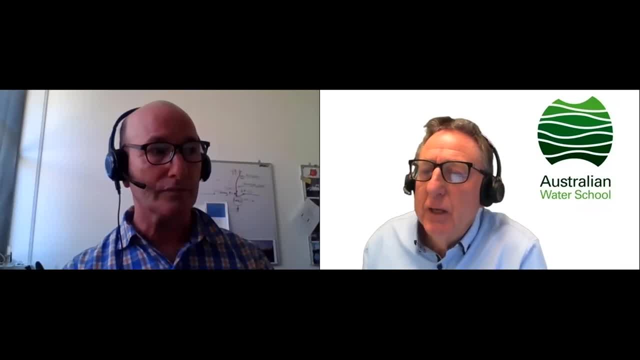 They're good references to have. All right, let's go to the next one. Thanks, David again. Carolyn Champion, amazing presentation. The question is: is there a way to re-stratify a mine after closing to improve stability and prevent water release containing contaminants? 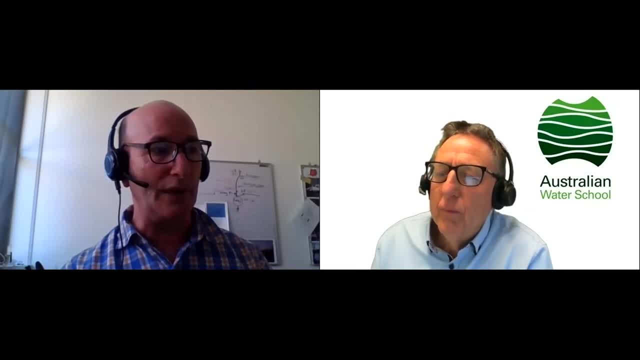 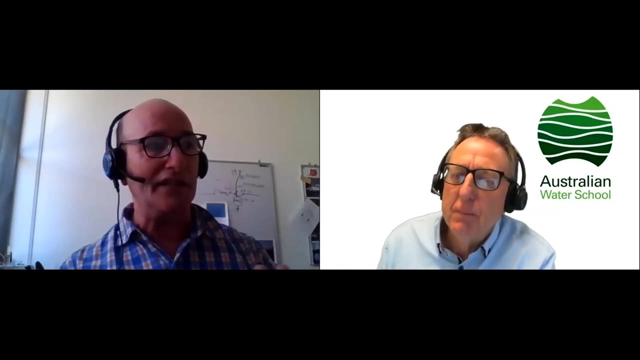 Oh, thank you. Thank you, Carolyn, Great, great question. Now I'm not sure of the term stratify, Trevor, perhaps you could help me. What does that mean? No, I couldn't, I couldn't. The main thing she's after is to improve the stability and prevent water release containing contaminants. 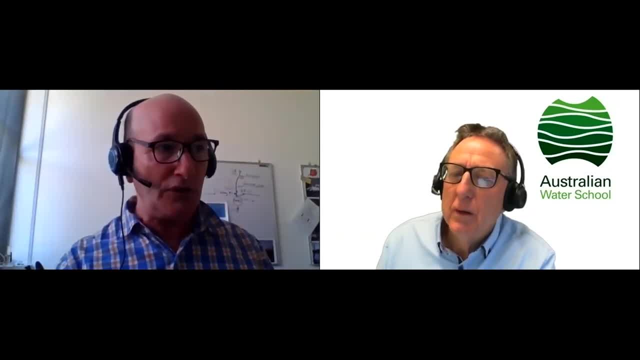 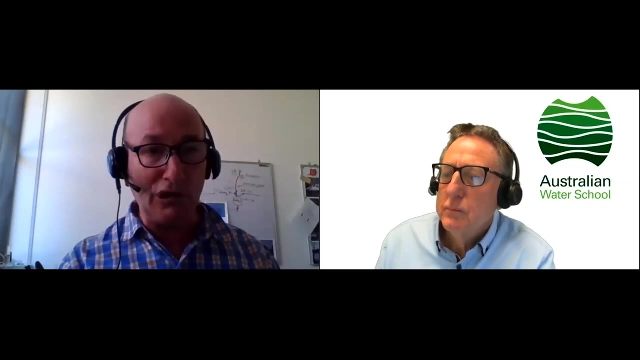 Yes, No, I get that. I didn't go into a lot of detail with the Berrimah mine. Berrimah mine's a great example. Ah, here we go, Layers, Layers. Thank you, Carolyn. So the Berrimah mine was the first example I know of in Australia. 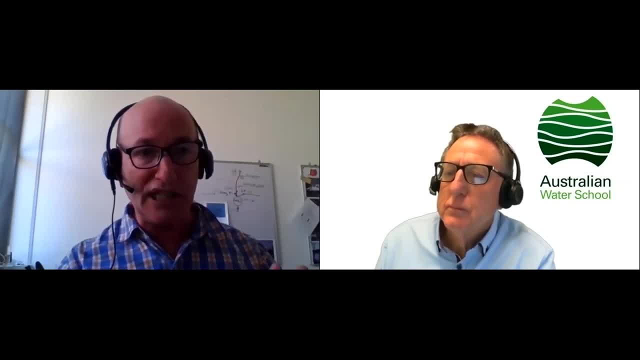 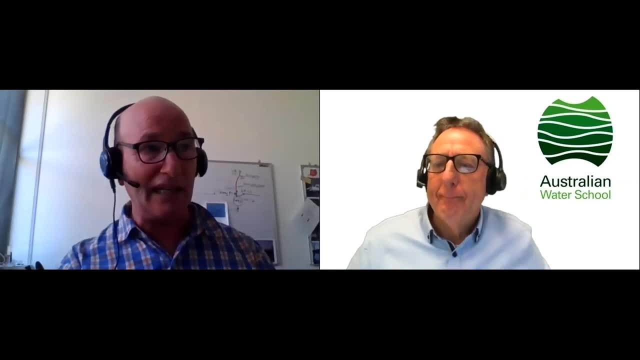 I'm happy to give Bora a rap for this. So the Berrimah mine was shut. They were in the process of sealing everything up And they were starting to flood the mine 15%. They went back in. They opened it up. 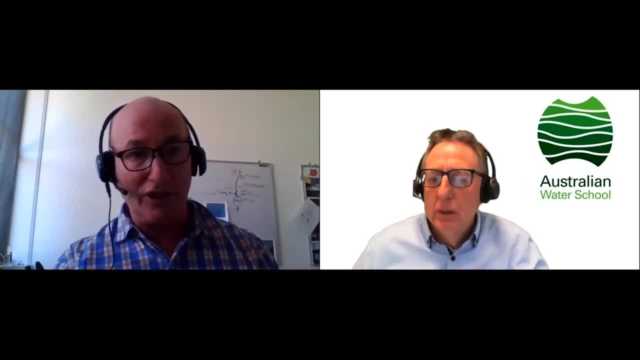 So they had to keep it ventilated- you know, keep air going- And they had to dewater it So you know you can't go underground if it's underwater And they, for a while they actually installed a limestone trench to lift pH. 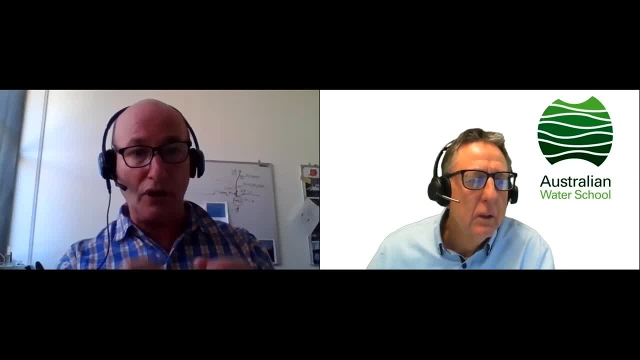 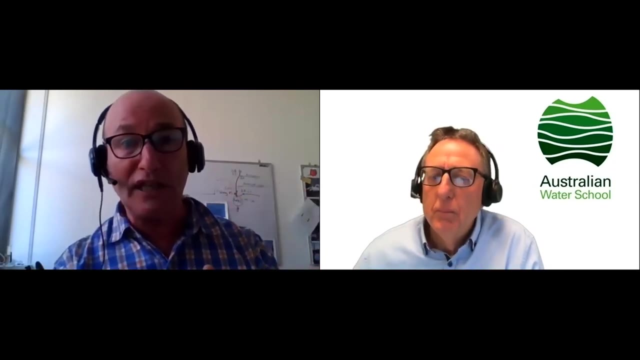 And it also allowed, you know, sedimentation. So the metals went out of solution, So sedimented and accumulated. Then they installed bulkheads And they're attempting to seal the mine and basically seal all that contamination in. Now we're holding our breath a bit to see what happens. 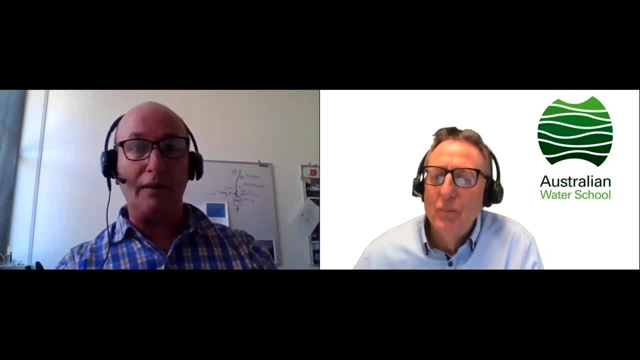 But at the moment the mine drainage discharge is trickling. It's not roaring out. It was roaring out at 2.6 megalitres, Olympics, women all day. The level of pollutants have stopped And we're holding our breath. 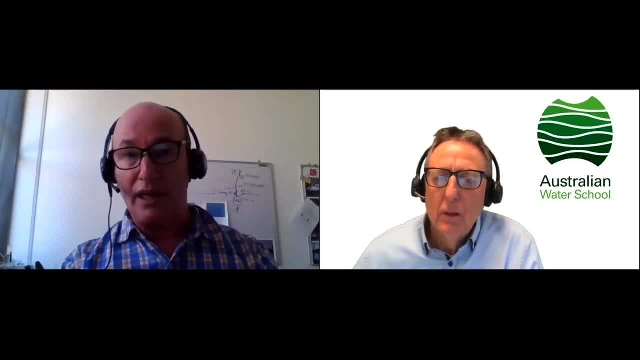 It holds Now. United Kingdom literature has shown that sometimes they call this rebounding. That is, the mine floods the workings And that pressure, that hydraulic pressure, can actually cause physical damage And it's actually blown holes out And the mine drainage has come out explosively. 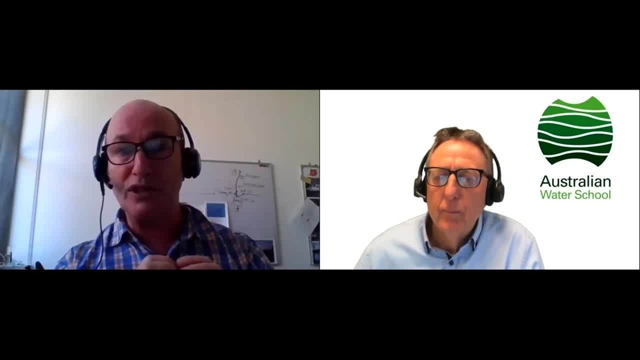 It's caused damage to civil engineering, you know, bridges, roads, buildings, et cetera, And also the pollution that comes with it. So I'm hoping this holds The Berry McColl mine, The shovel mine At one point. 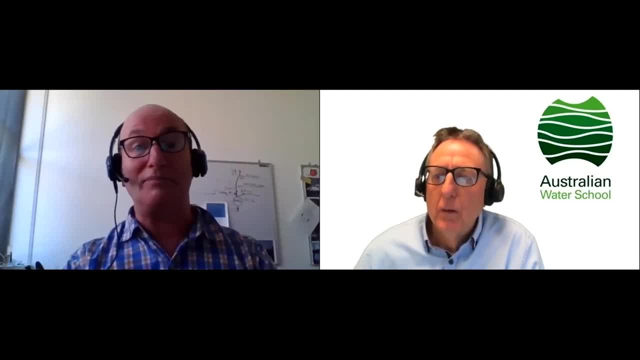 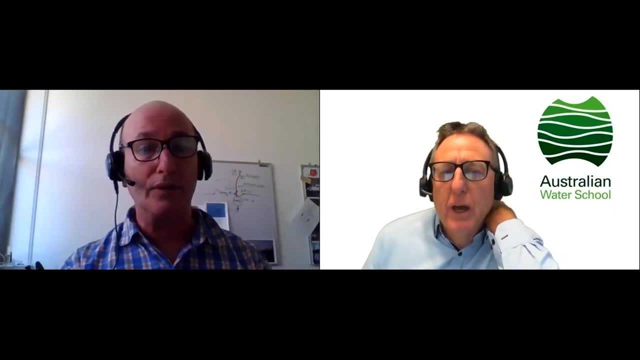 But it was mechanized in the 1930s. So yeah, I'm going to report back on that. So patchy, so far It's not absolutely clear. That's a fair comment, But bouquets to the company giving it a go. 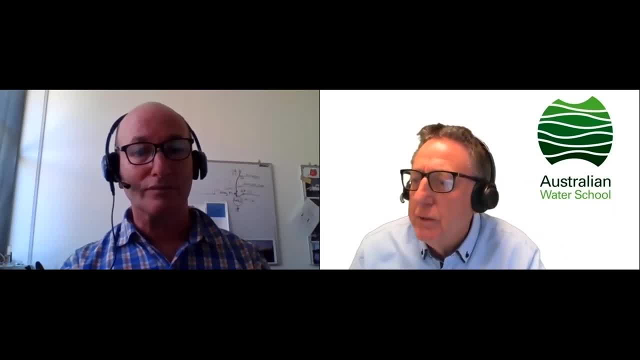 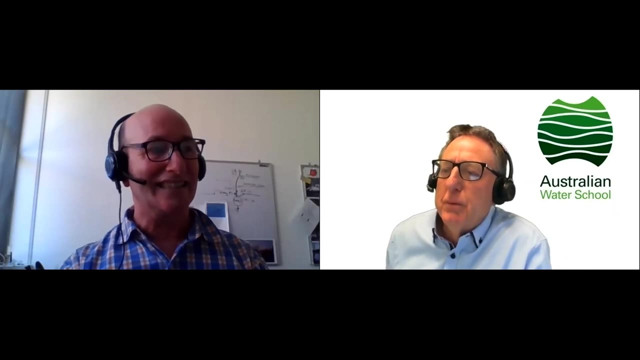 Absolutely Sure thing. There's a lot more questions coming, So we might have to do these faster answers, But let's go. I'm surprised to see that selenium and nitrate are not key contaminants of concern for these sites, Particularly compared to metallurgical coal sites in North America. 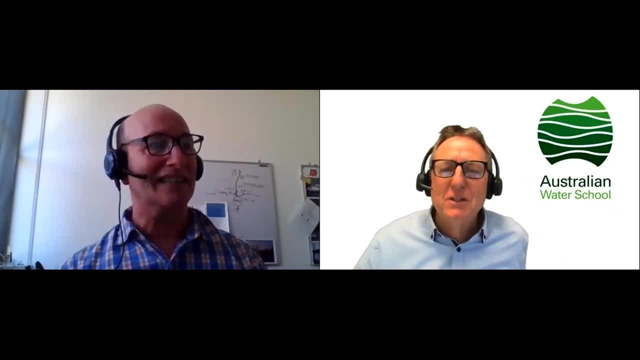 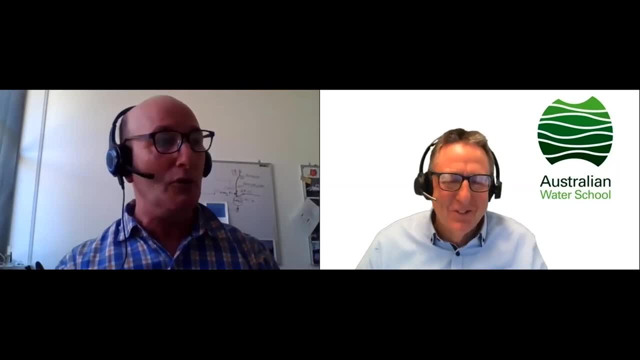 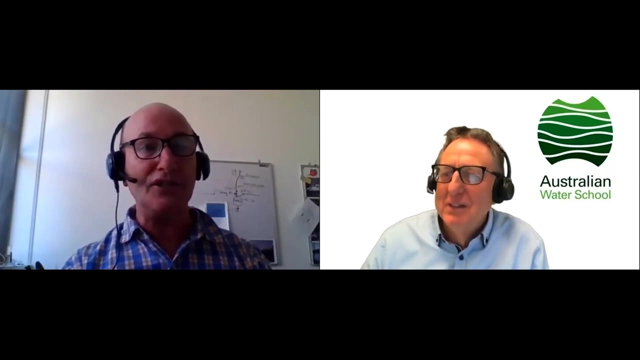 Are these deposits simply low in selenium and nitrogen parameters? I love that question. I'm learning from my audience now, Trevor. I love these questions. Good thing, We do test for selenium And every single one we go to, So we've been studying seven. 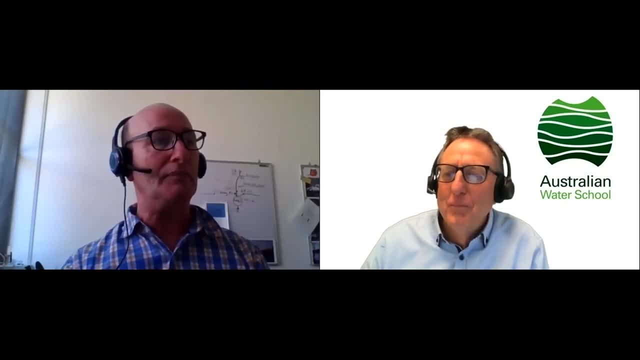 Every one has a different kind of periodic table Few common elements. Some of them have really high levels. I've only recently started looking at nitrate. It is always high. Honestly, I had just been missing it. I'd also been seeing plant growth and algae in particular, flourishing downstream. 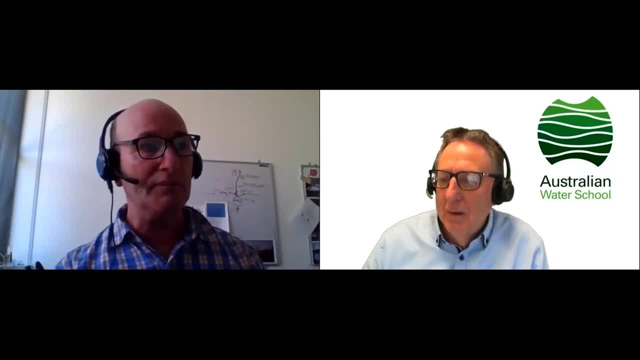 So, to be honest, I'm going to add that in. We're adding that in now to our studies, So I think that's a great reminder. Thank you, Julie Martinson says I think this is an important issue internationally and in Australia. 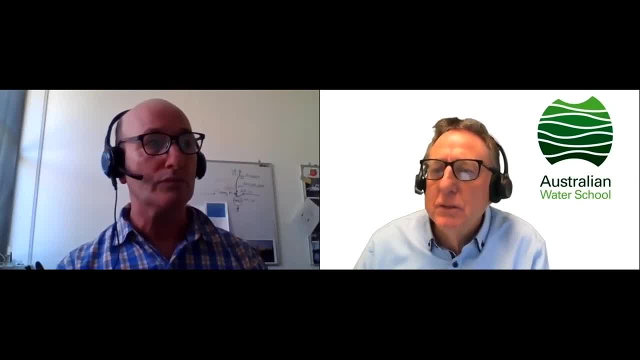 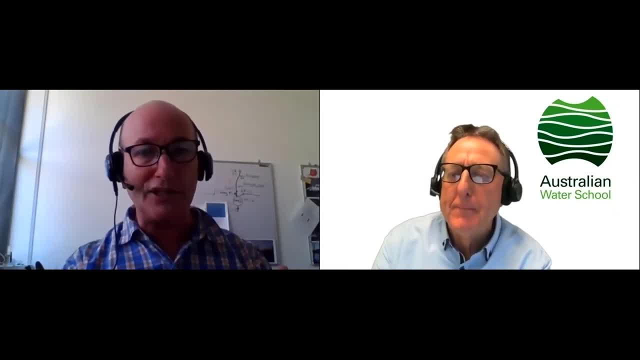 Thank you, Simon. You know something funny we're seeing. We're actually seeing a lot of the coal products actually appearing in urban areas And we think the link is one of the byproducts of coal mining, and the power industry in Australia burns coal. 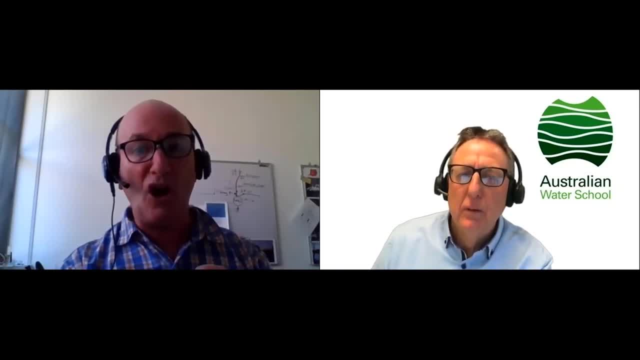 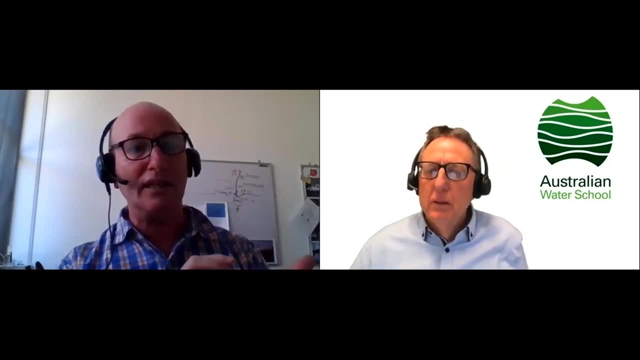 Fly ash is often used in making concrete. It's a major component And when the concrete leaches- which all concrete does- we start to see, you know, particularly barium and strontium indicators for me. So yeah, it's common across industry, but also in urban areas as well. 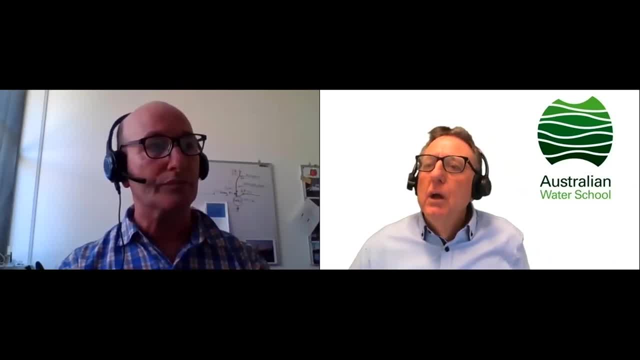 And there might be a common link back to coal. Next one, Kirsten Braun says: has there been a change in downstream sampling sites at the active mine sites since the licence conditions were changed? Perhaps the licence conditions were changed to include metals in 2013.. 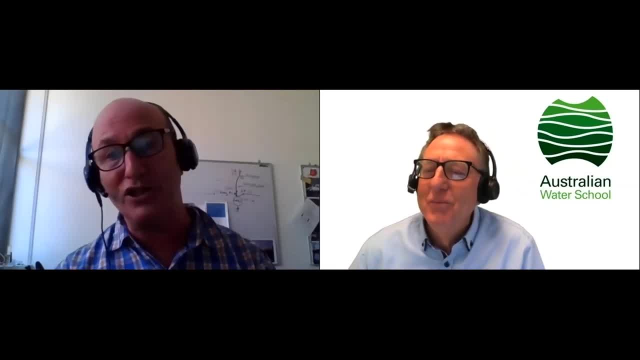 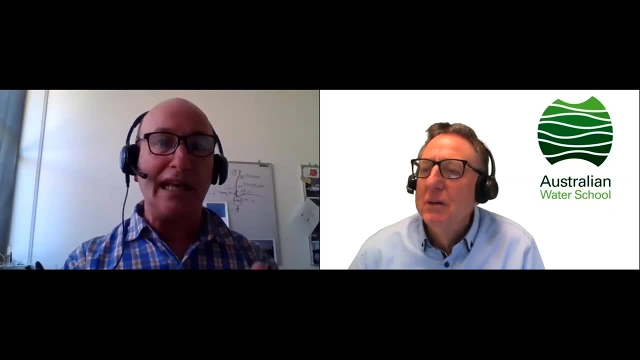 Oh, thank you. Thank you, Kirsten, That's a great question. I've actually got a master's student studying the Georges River and looking at that mine, And the answer is yes, it has improved. However, the EPA- the regulatory authority here- had given quite generous discharge limits. 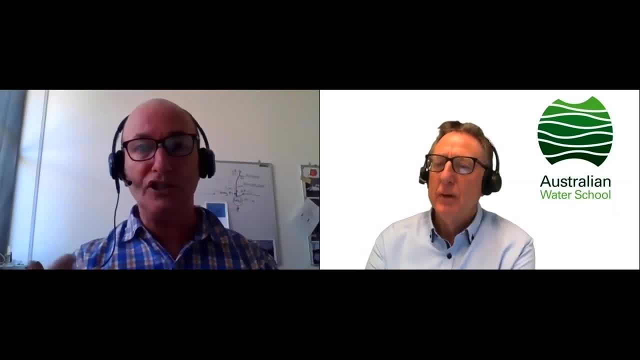 So they were quite high levels. In a way, you could say that they were, you know, legitimising the pollution. But also we're in a severe drought At the moment And in fact, that river has stopped flowing from time to time. 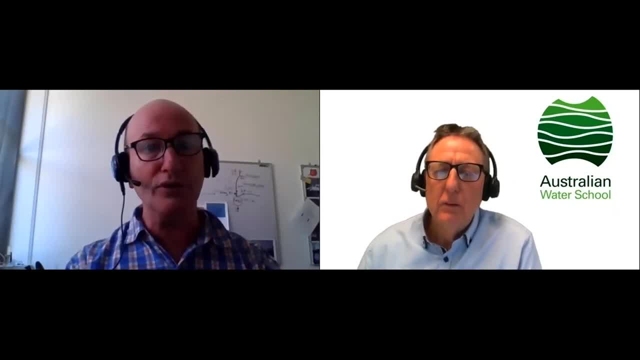 So dilution has dropped, So we've seen some things improve. Some things have got worse, But that's probably more due to climate. But yeah, great question, Thank you, Moey Tiong has asked. thank you for your passionate presentation. 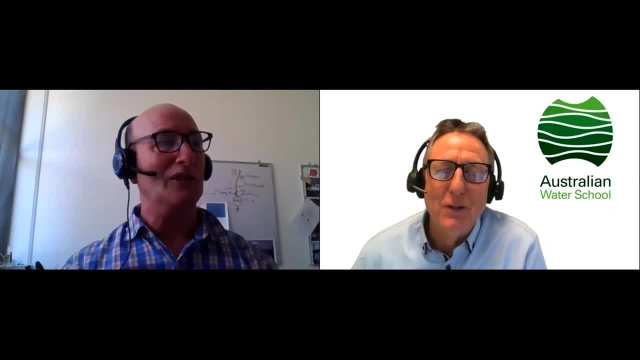 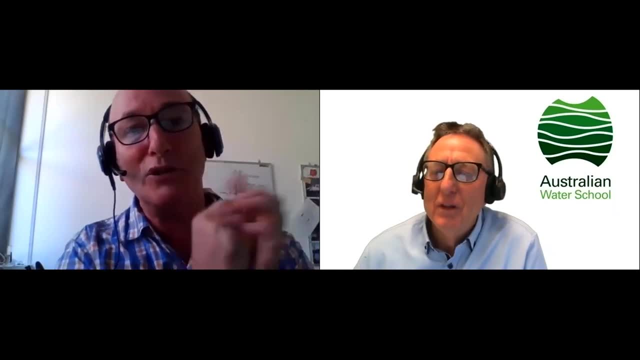 Ian, is there a risk to Sydney's drinking water supplies? Thanks for the comment, Moey. Very much, And yes, there is Two of the mines in that, Three of the mines in that actually go into water catchment. 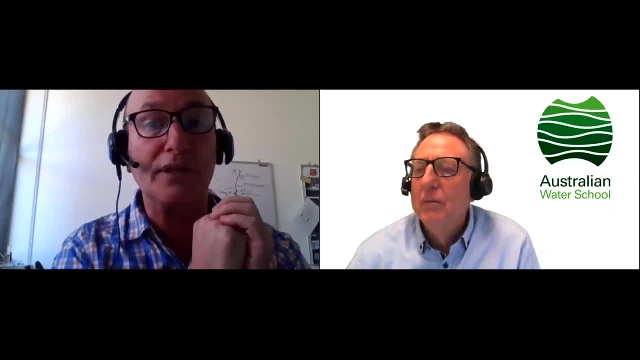 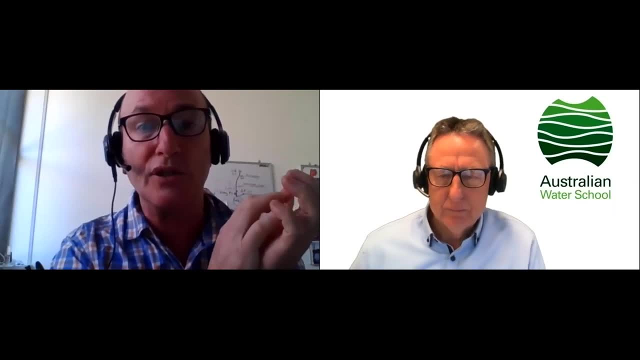 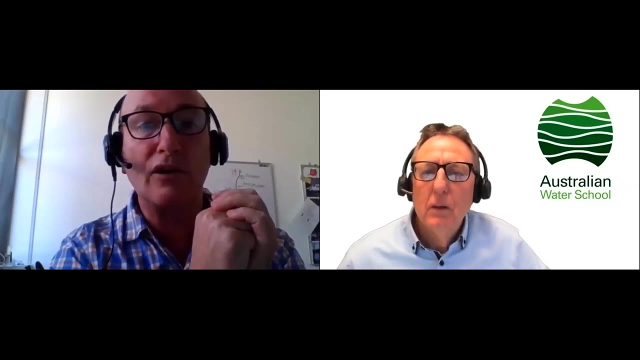 Lake Barragarang Warragamba Dam, our biggest water storage in Sydney, And some of the media I've been involved in last week. There is actually an accumulation of contaminated sediments from mining- probably long-wall mining- in two of our oldest storages, Cataract and Cordo. 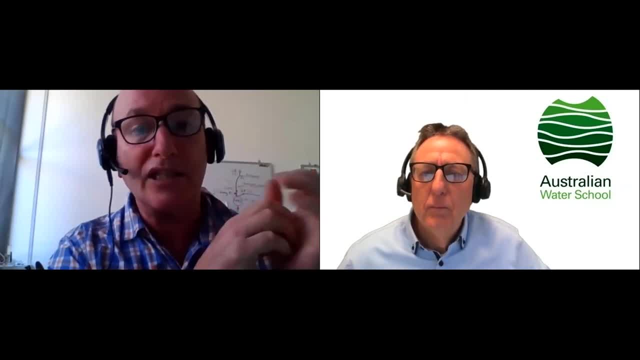 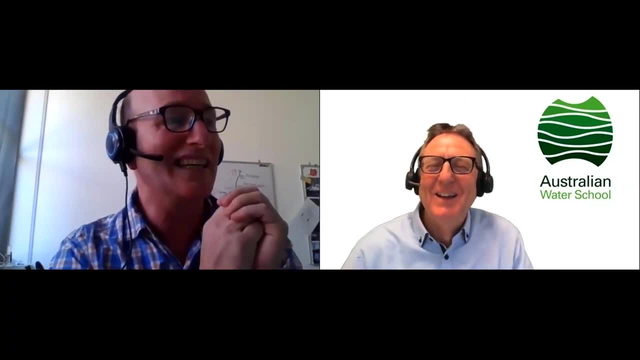 So, yes, it is accumulating in our water supply. It's not adversely affecting drinking water quality. In many ways, people are tougher than aquatic life. Well said, Well said Nicholas Cone has said. a lot of water quality assessment appears to relate to surface flow. 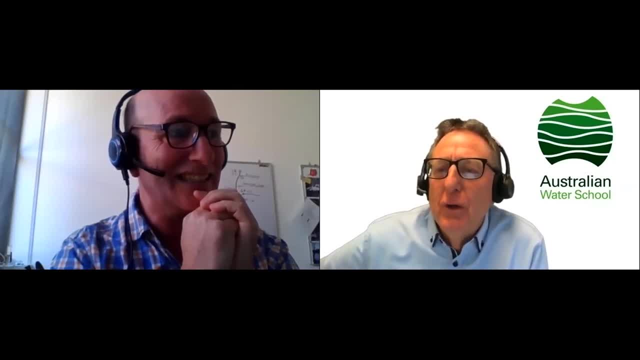 Do we know what impacts on the subsurface water and is this as critical? Might be able to take that, Ian, with the next one by Pang Catch Great talk, Ian. Yes, Have you found any impact on groundwater or aqua downstream and also impact on streams and wetlands near the mine? 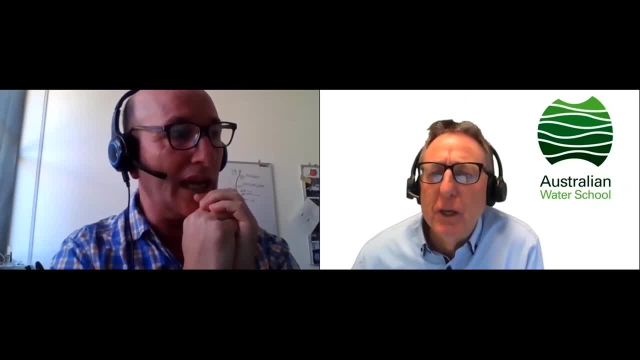 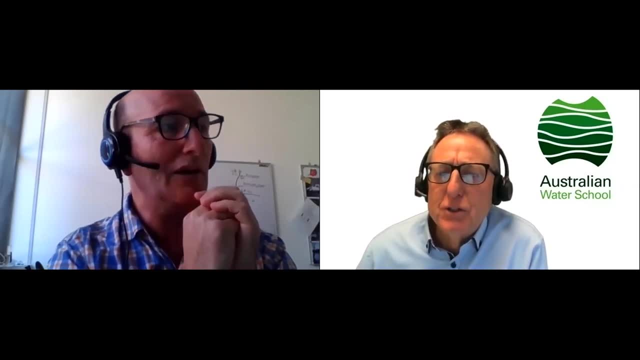 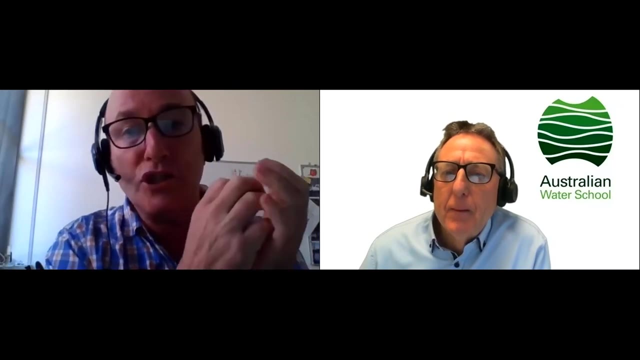 Spring is near the mine, he says: Fantastic, Fantastic, Fantastic, Fantastic, Fantastic, Fantastic. Thanks, Nicholas and Pang Catch. I don't tend, I'm not a, you know, a hydrogeochemist. I don't go underground. 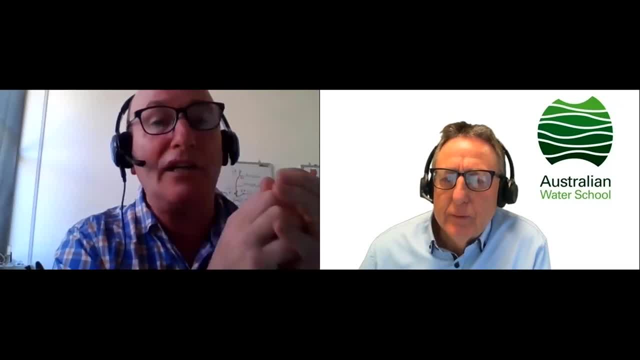 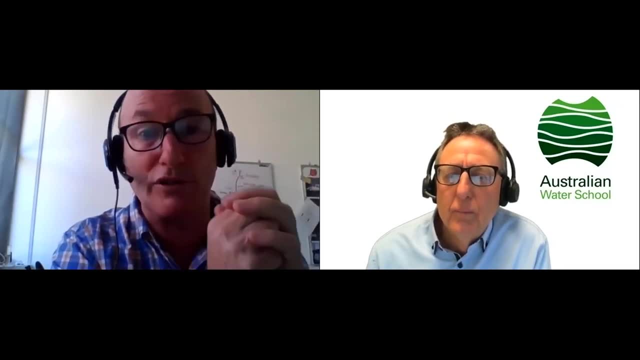 I wait till things come to the surface. Without a doubt, there are impacts on groundwater. Groundwater aquifers are really important. in Australia, Most of our water is actually groundwater. There is definitely impacts down there. We see it when the water surfaces. 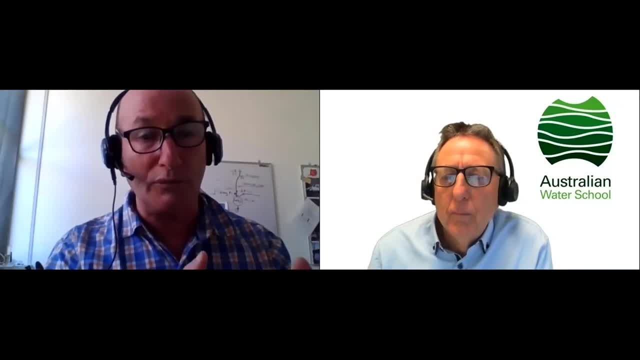 So like the very last image I had, that was a cracked aquifer that was contaminated By the fracturing. Yes, absolutely, there are impacts in the groundwater In terms of wetlands. I haven't studied many wetlands downstream. 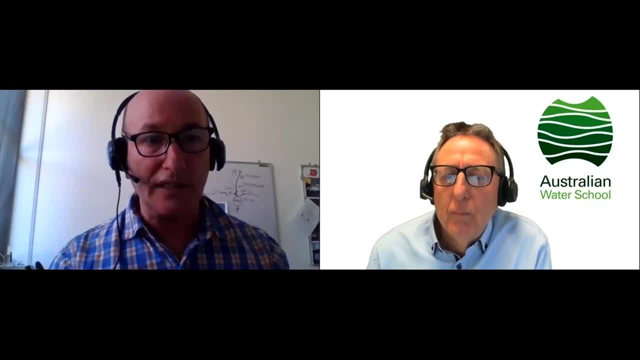 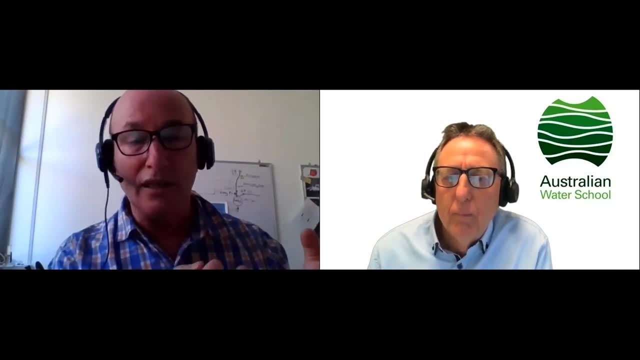 But often wetlands above the mine have been cracked and then drained, And then we've had- And some of these are very high conservation value- wetlands in the Blue Mountains And we've often lost plants and fauna. Great questions, Thank you. 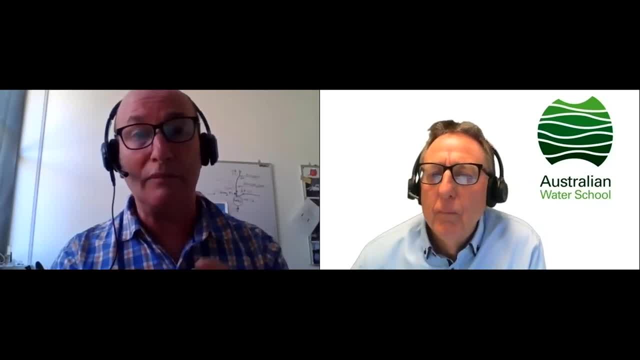 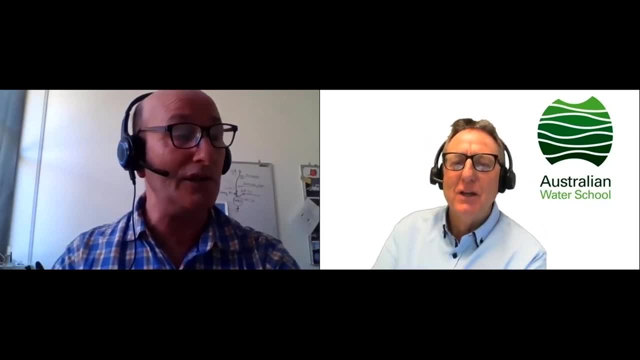 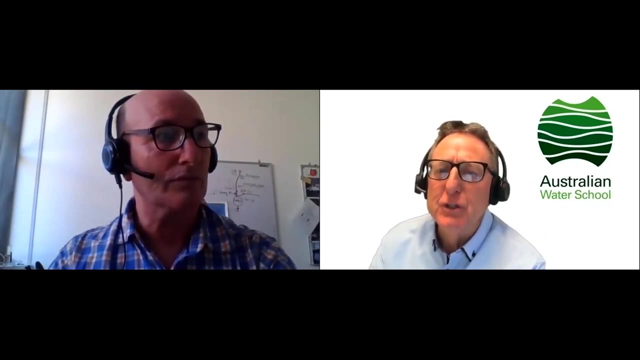 We're getting some probing questions here. Here we are. It's good. I know that there's been a lot of talk about you know. you know it's good. I know EPA New South Wales focuses on water quality. What do you think the Water Regulation Agency in New South Wales can do in the future? 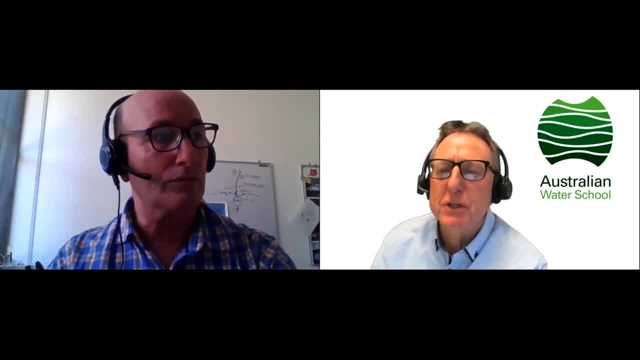 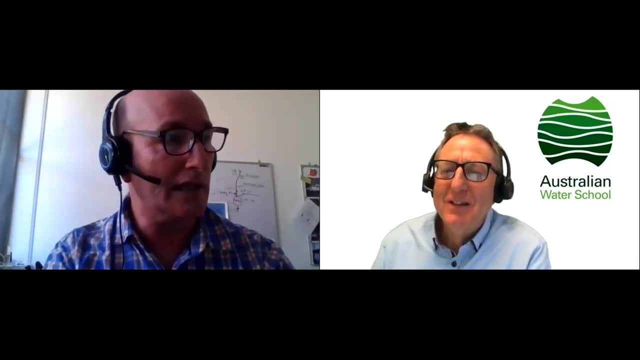 to provide more support for water resource management. I've worked really closely with the EPA And- look, we probably weren't friends to begin with. I never got Christmas cards or anything, But I've got an open dialogue now. I share with them the research. 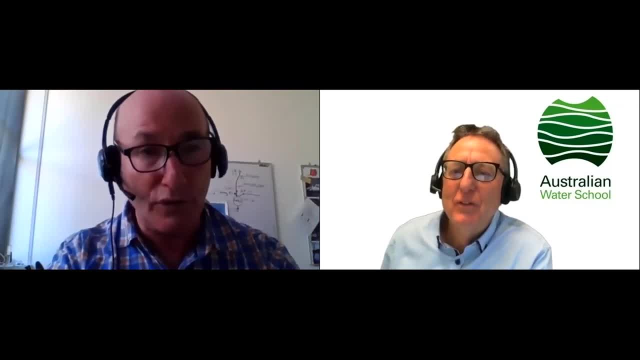 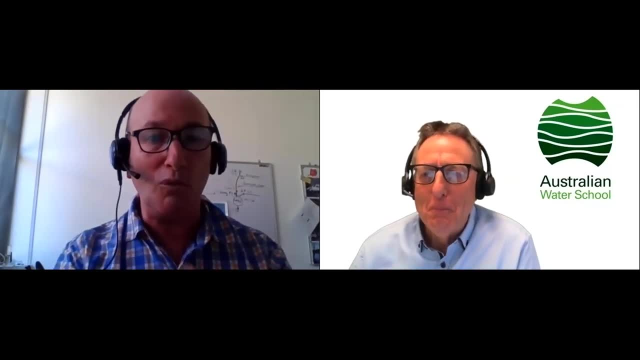 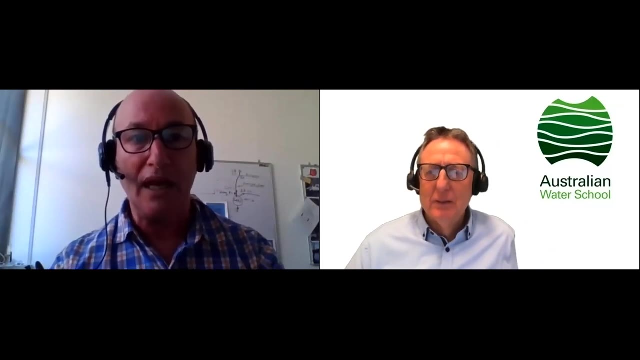 They have changed. I did feel for a while like a one person EPA with my students But to be honest, we're changing the way they regulate. in New South Wales There was no doubt that industry- the coalmine industry- had a lot of political support here. 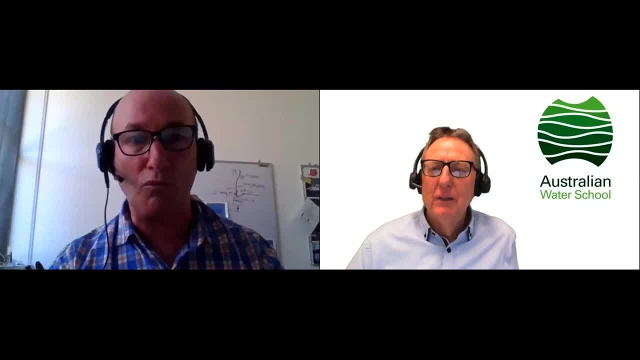 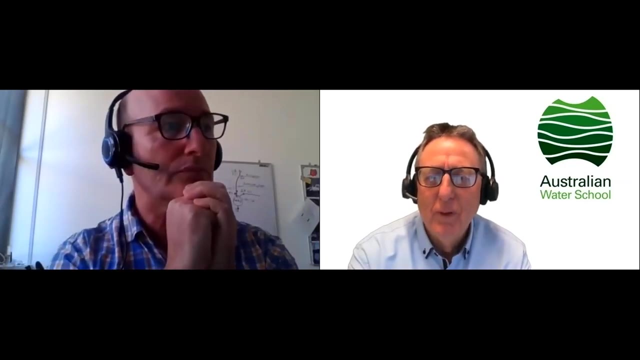 And they regarded any money spent on cleaning up the drainage as a waste of good profit. So we're sort of attacking that culture by highlighting these problems and the EPA, with the media, with the politicians- we're all learning together. There's a huge interest here today. 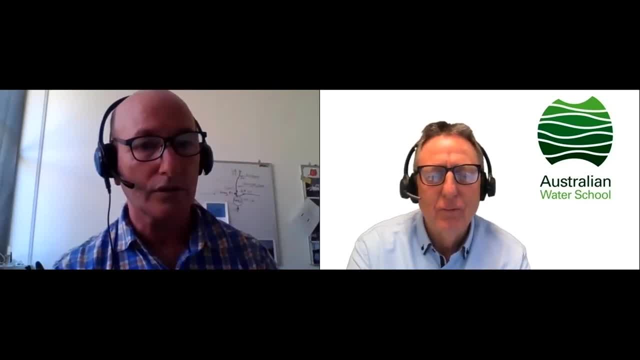 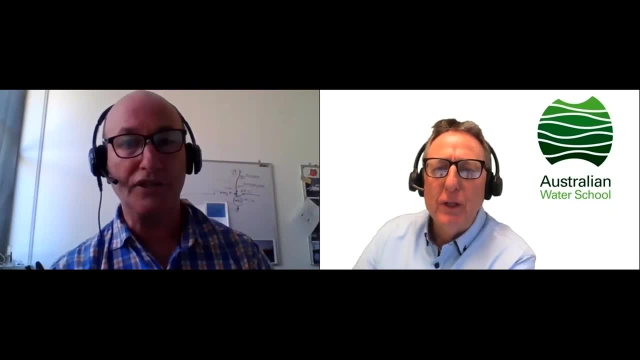 That's for sure, And probably a lot more in the recording. after this webinar is over, We'll put it up on the web and there'll be a lot more interest from there. We'll track that as well. Julia Emery has said. 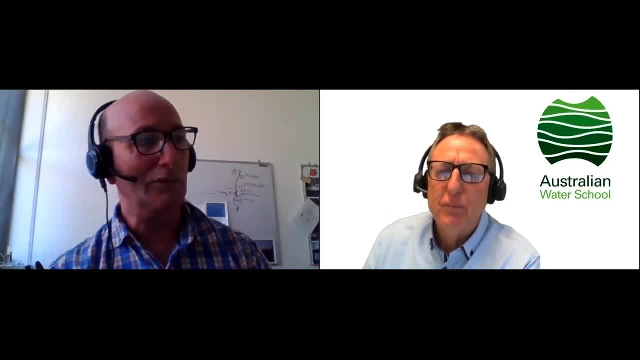 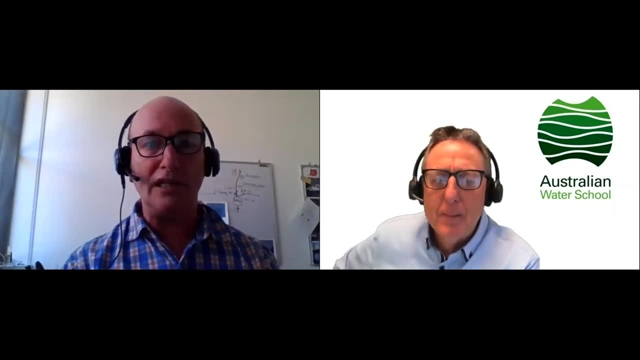 have you found a significant increase in salt loads downstream from discharge points in your research? We're getting great questions here, Trevor, I really appreciate this. Thank you for that, Julie. I think we're getting a lot of questions about salt levels. I often measure that as electrical conductivity. But yes, all coalmine discharges here increase, dissolve anions and cations And sometimes we get an increase of up to 20 times in the salt. And part of that is because some of the geology of Sydney. used to be under the ocean, So there's very, very high salt levels down there. But it's also when you break down and look at what's in that salt- like a calcium bicarbonate salt- that comes out. So, yeah, really good question. 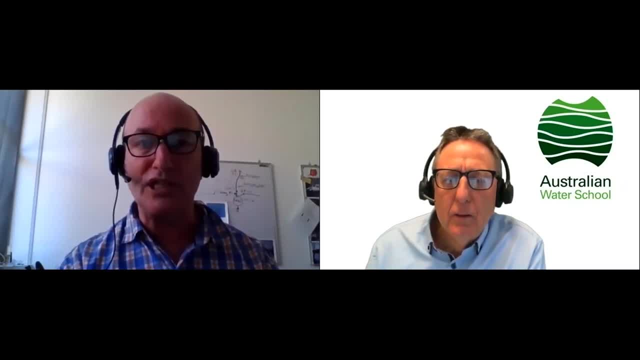 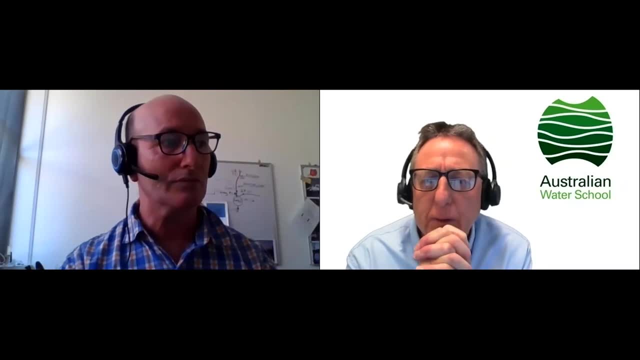 But yes, we do have mild to moderate salinisation associated with this. Another question here about groundwater. I'll take it while it comes, although it's down a bit. Brian Keogh has said: thanks, Ian. with cracking in streams, disappearing the surface water, 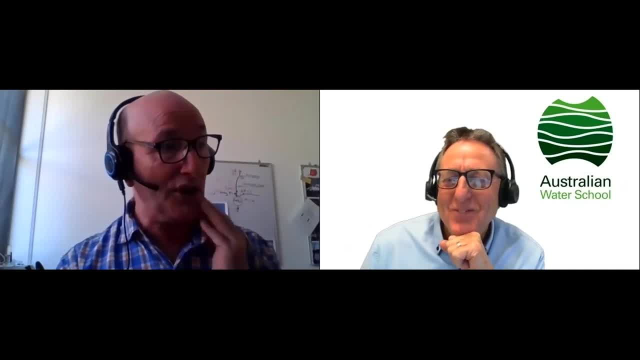 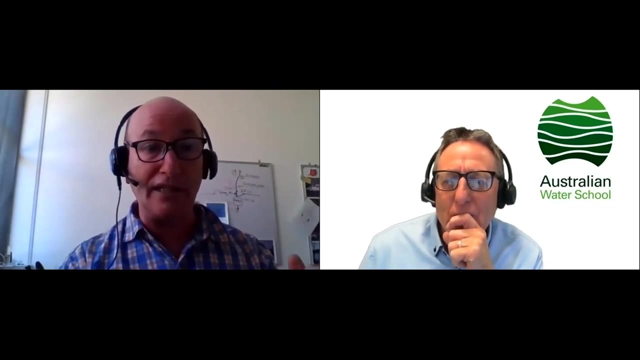 is there an increase in accessible groundwater? Oh, good question, Isn't it? Great question? I'm not sure of the answer, but this is really a point of contention. There are quite a few coalmines that we know that they're cracking aquifers and they're draining. 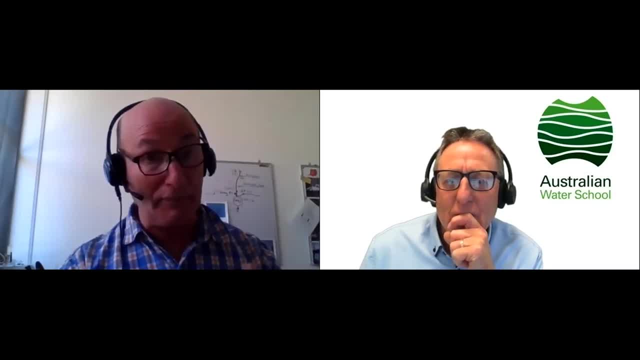 groundwater. It's a bit hard to tell what's happening, but I'll tell you what. they're generating a massive volume of wastewater and that's possibly where the groundwater is going And one of the biggest points of contention for a lot of people. 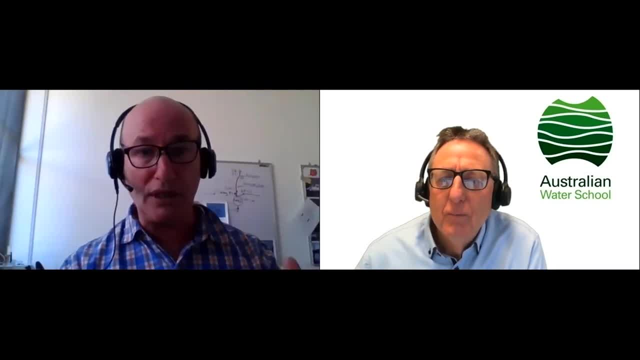 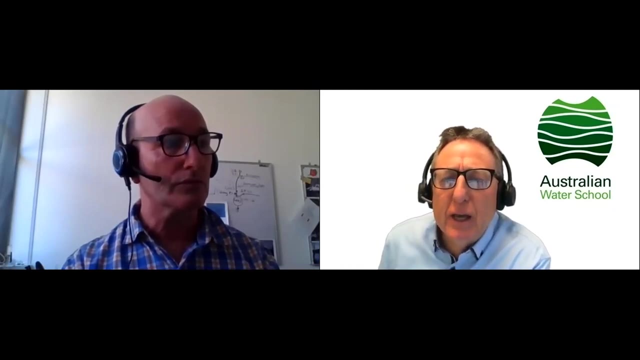 surrounding the coalmines is that they have dropped the level of groundwater and they can't. they either have to dig a deeper bore or they just lose access to groundwater. But yeah, great point, Thank you. David has asked: do you think there's an opportunity for government agencies? 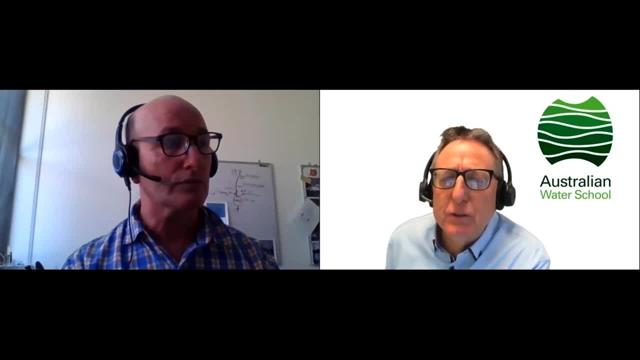 academics and private companies to interact and share information to improve performance and breadth of environmental monitoring. Are there any forums or groups that can be set up to encourage a digital world platform for water quality? I think that's one of the guts of the issue here. 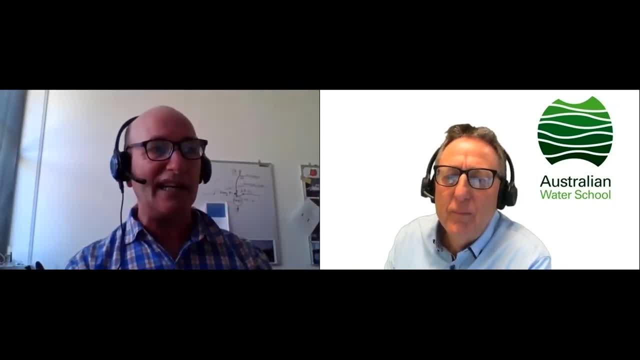 Yeah, thank you, David. That's really, really good At the moment. I'd say it's rather disjoint in terms of the government agencies And it's probably you know. for example, the mining industry here is supported by the you know for government. 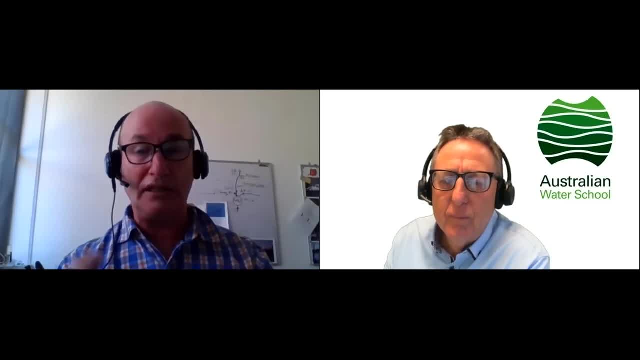 it provides employment, investment royalties And they'll do anything to encourage that. But they need to balance that with the environmental impact. So I'd say at the moment it's still a bit difficult for government and even I can actually see that the government agencies 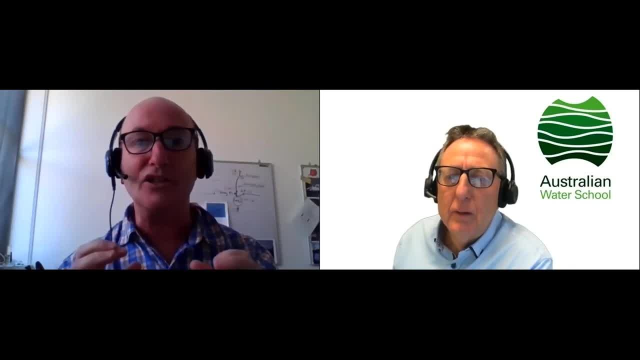 there's a bit of a fight on their hands, But probably leading. that is community concern. And it's probably community concern with the burning of coal and the impact on the atmosphere. In some ways water gets forgotten. But look, I do see in all of my research. 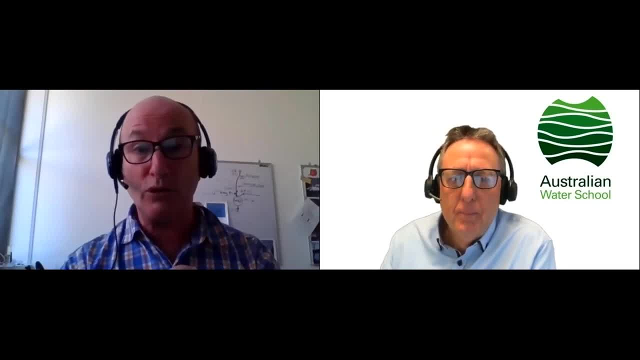 I actually link with local groups, I talk with stakeholders. Plus I talk to the mining industry And I think we all realise that we have to work together. We have to be open and honest about these issues, Not anti-coal mining, but if there's an issue. 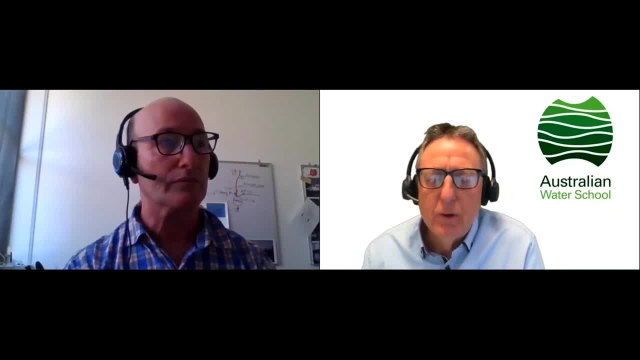 let's be open and honest about it and see steps taken to manage that. That's the moderate, progressive view that we need to have, Not just black and white. I mean, it'd be easy to do black and white, Anyway, let's go on. 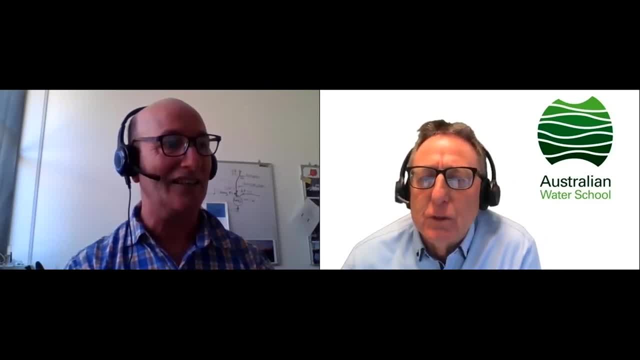 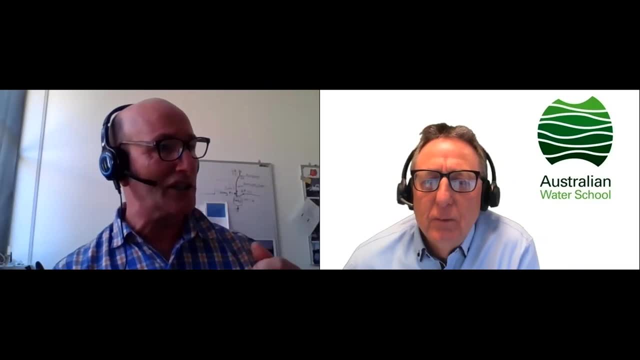 Camilla Scott, we've still got 15 minutes to go here. Let's keep this going. Camilla Scott, how do you go about remediating the affected creeks with coal mine sludge? I'm not sure about this one. 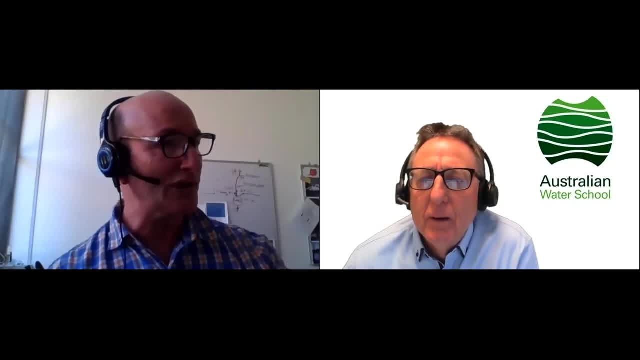 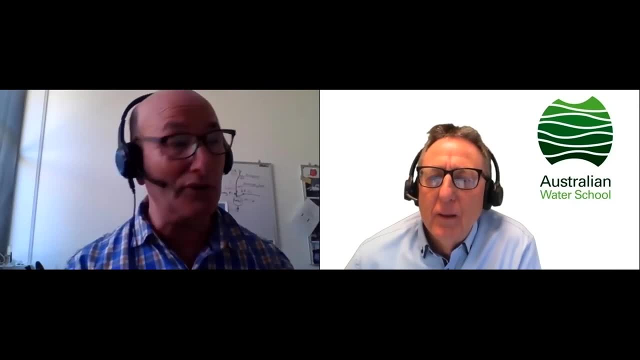 I might need your help, Trevor, Using the coal mine sludge or the creeks that have been affected by the coal. No, the second Great example. It's really difficult. Great question, Camilla, When I was working on the Clarence coal mine. 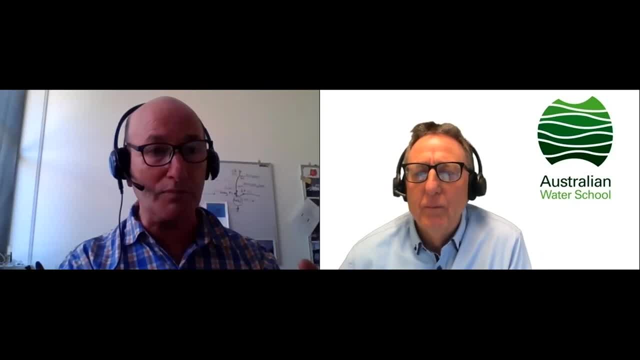 they actually lost their. They actually had a giant spill of their coal washings. In fact, a whole lot of coal mine sludge entered the river. Short answer: they were fined a couple of million dollars, but they spent a fortune. They sent poor people. 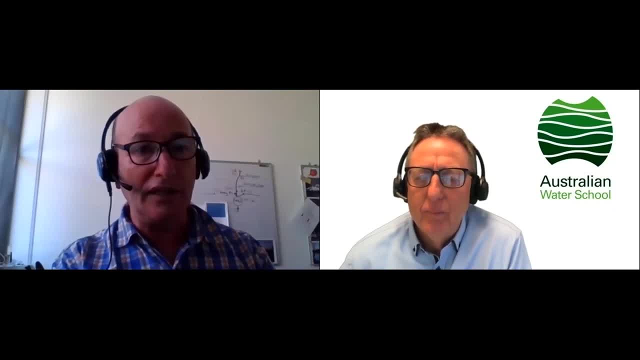 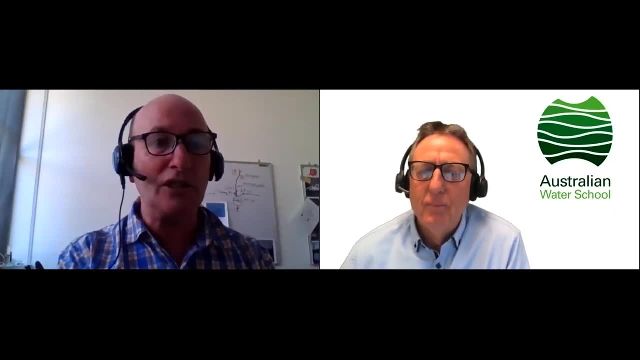 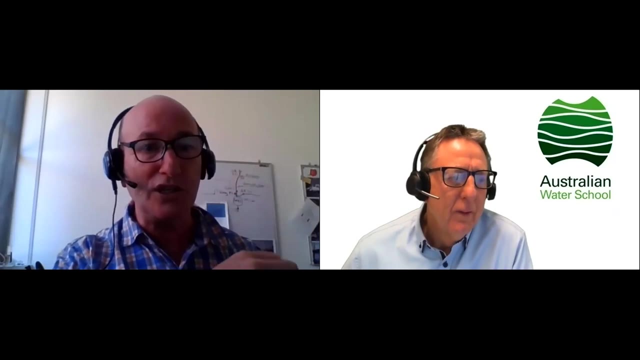 into that freezing cold mountain river and they used a sucking device to suck out as much of that contaminated sediment. The sediment contains so much more of the pollutants it tends to get mobilised and re literally diffused into the water quality. It's difficult once it gets in there. 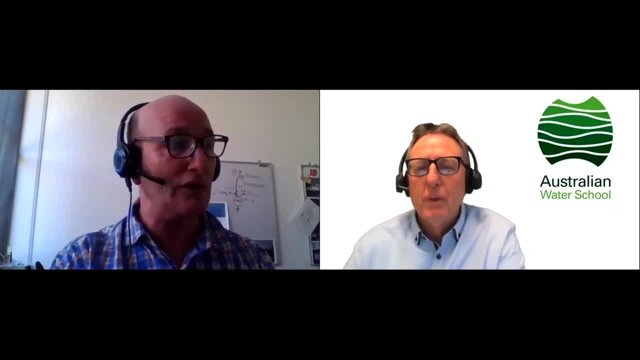 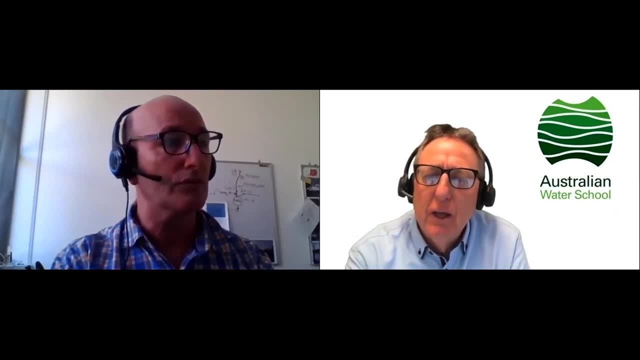 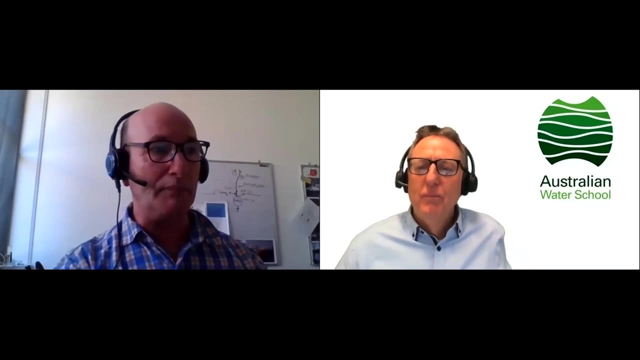 And sometimes it's just too late to get in there. Yep, Great question, thank you. Rafael has asked how can we differentiate metal discharge contribution from the local geology from those from activity of coal mining? Oh, good question, Rafael. 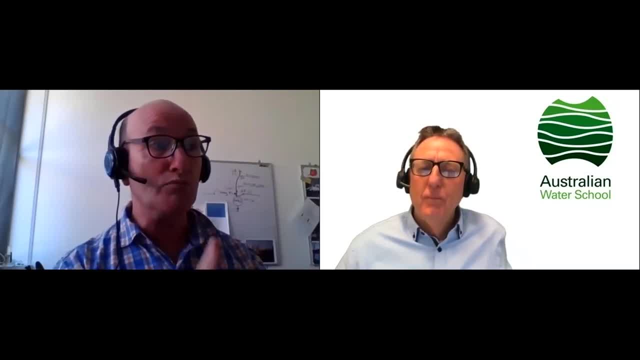 That's why I always use upstream reference site And when I can, when it's available, I'll use more than one upstream. So I'd really learn what are the natural level of metals. I always see iron, manganese and aluminium. 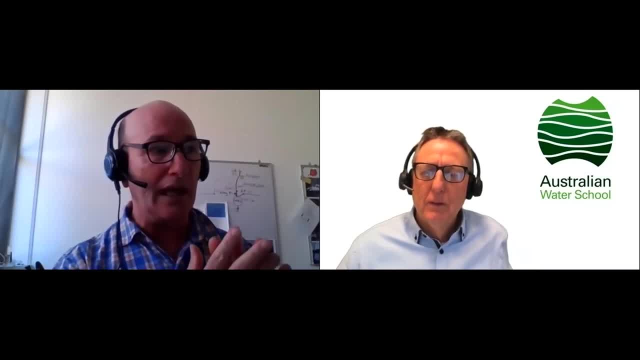 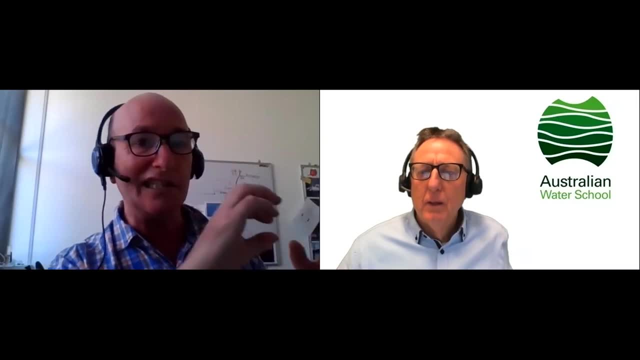 They're key metallic elements of the Sydney geology And once you know the background- and you really do need to know the background level of metals- you can then see the signature of the mines. So it's like a triangulation. You have the background. 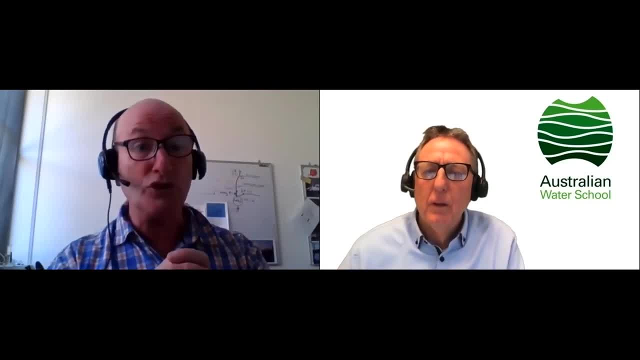 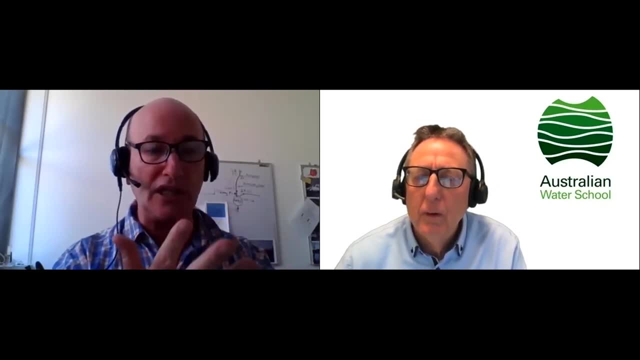 you're then looking at what's coming out of the mine. then you look at what's downstream, And it enables you to quantify how much of that metal is in the mine. So things like barium, strontium, lithium, titanium, zinc and nickel. 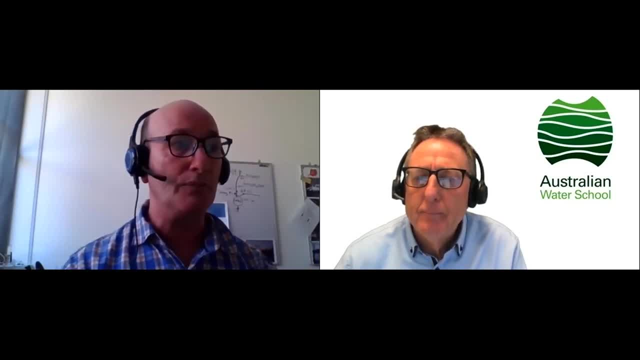 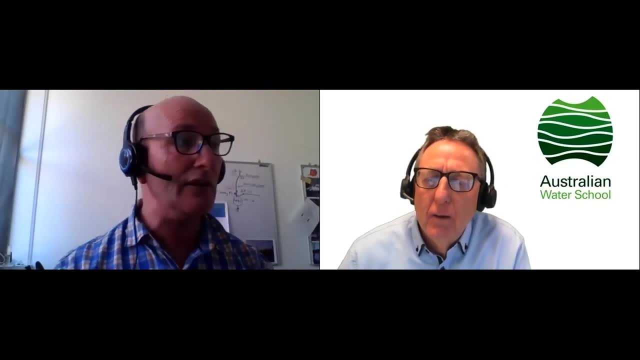 and a whole lot of others. even uranium and arsenic stand out. Great question, thank you. Claudia has asked: have you done any measurements of metals accumulation in plants? Yes, thank you, Claudia. thank you, I've got an experiment running 20 metres from me. 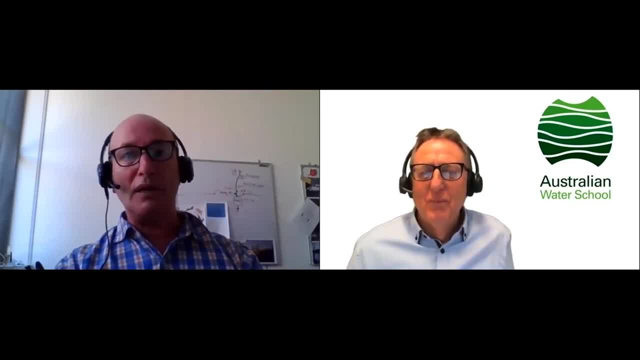 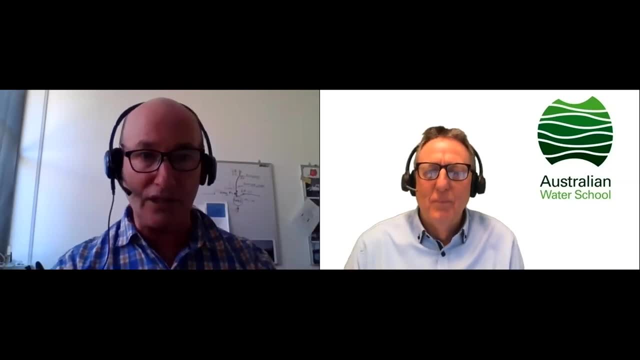 I've got a master's student. We are doing exactly that, Thank you, thank you. thank you, Claudia, Because one of the questions is: what about stuff? But what about plant life? That's the basis of the food chain. 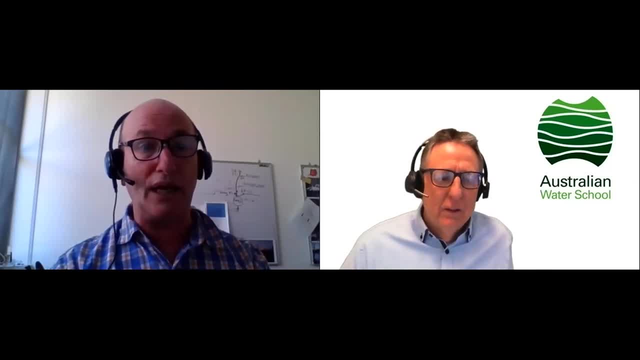 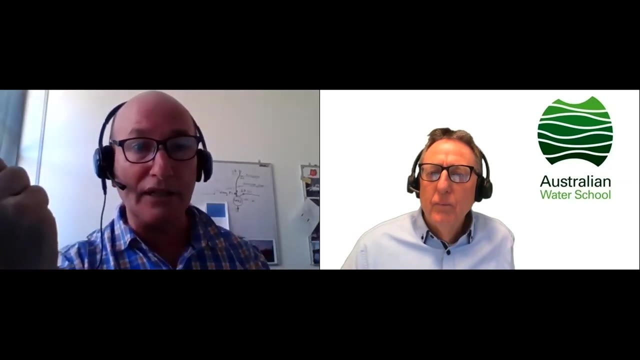 And we are finding. yes, some of the metals are actually moving into plants And we're trying to work out where they're going and how. But the roots seem to filter out some of the metals, But we are seeing bioaccumulation in the plants. 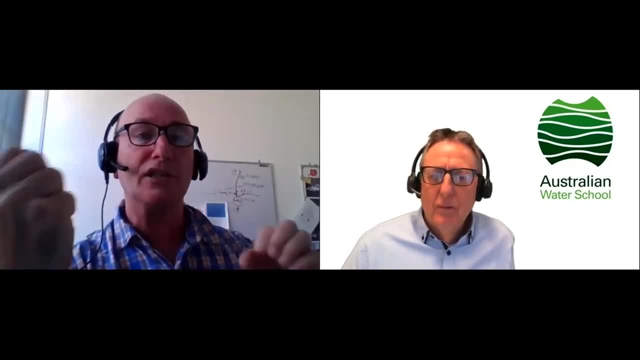 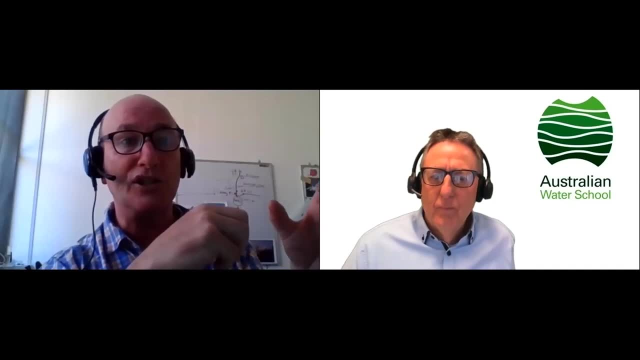 We've also done studies of my Brady Bunch photo of invertebrates, Top left predatory beetle. It's a predator. It's a couple of steps up the food chain And we've seen bioaccumulation of metals in those beetles downstream of mines. 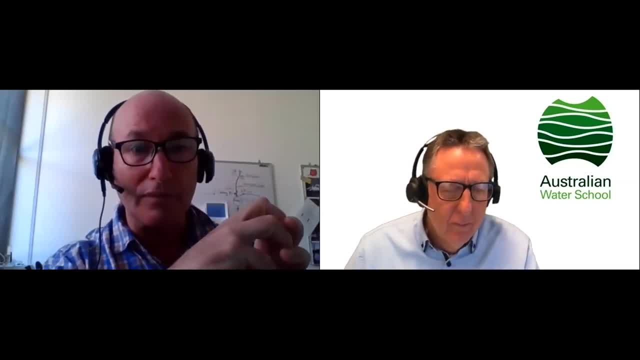 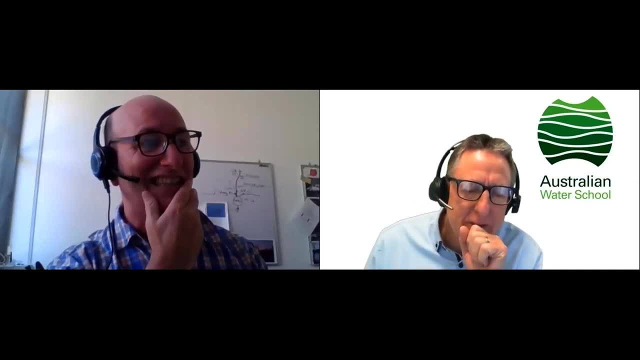 that don't. we can't even detect them in the water, And so that's biomagnification. Great question, thank you. I love that slide of your Brady Bunch. It just shows you the sheer breadth of animal life, And then the graphs showing how much. 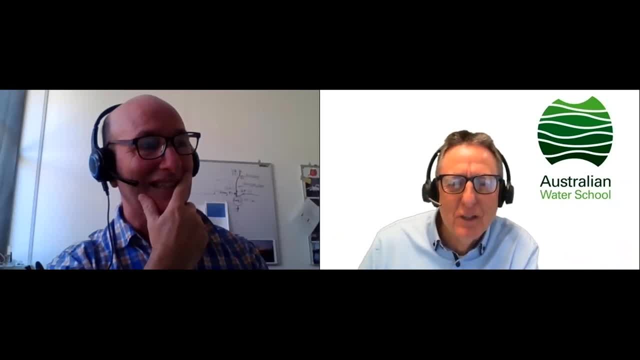 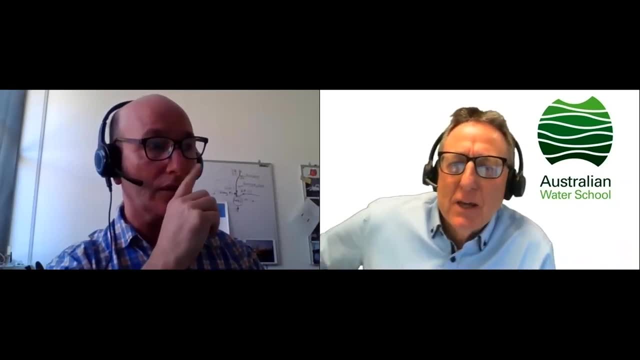 they've been reduced by downstream. They've got to be saying something to us, Even though we don't know the full effects, but we do know they've been produced hugely. Thanks, Trevor. Sanjay says. other than the macroinvertebrate. 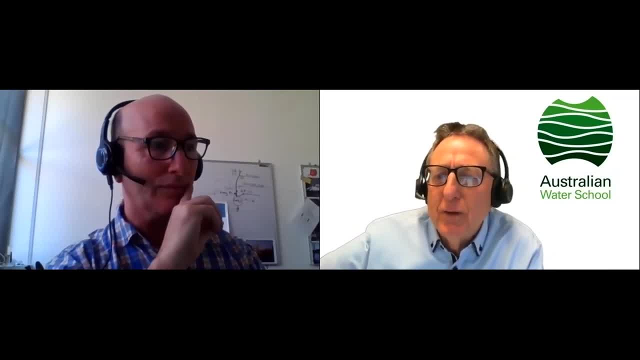 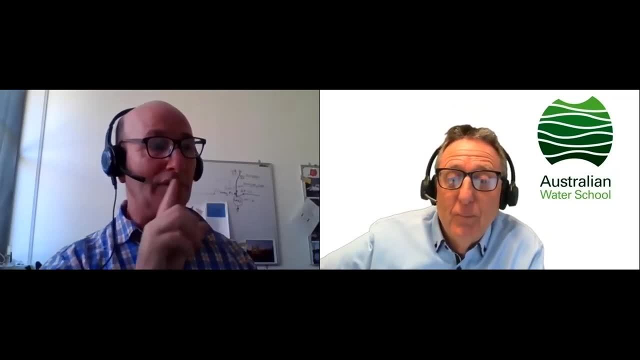 community index. do you recommend any other methods to measure the effects on aquatic life, Like: is there a point downstream where rivers actually recover? Trevor, I'm loving these questions. They're fantastic. Thank you, Sanjay. Yes, yes, yes. 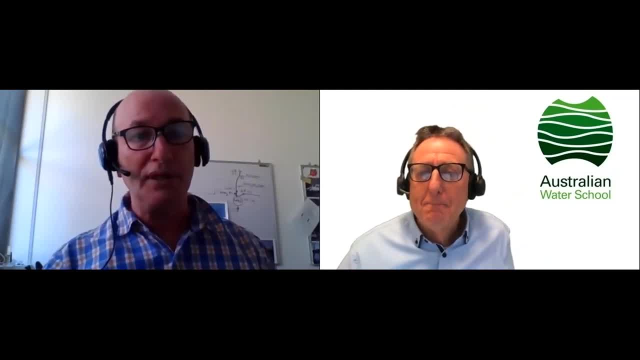 I do invertebrates because it's cheap, it's easy, I've got the skills, I can train my students. But there are so many other things I would look at. It really depends on what your river is. I would love, for example, to look at. 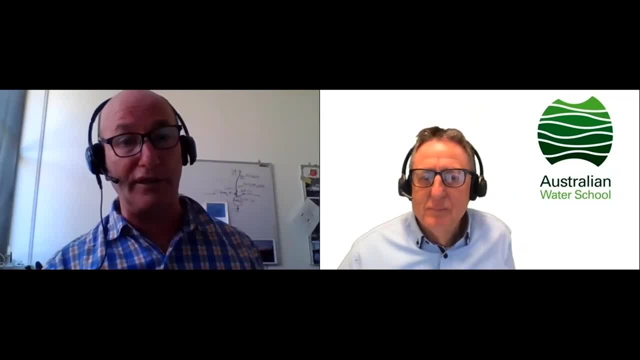 platypus, Or if it was a major fishing river, absolutely I'd be looking at fish and looking at fish larvae Depends. pardon me, you've got to get approval to use different things, But algal diatoms are one of the best. 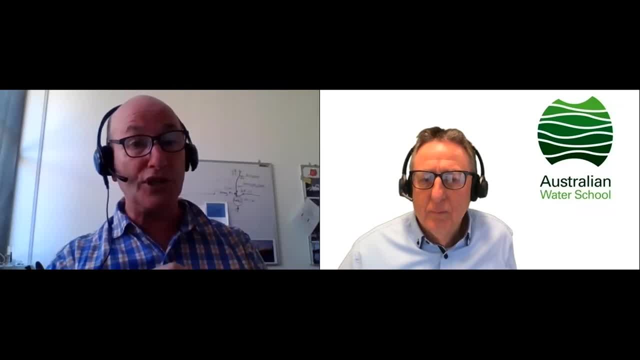 We've been doing that. we haven't published much of that yet. Algal diatoms: we've been doing that for a long time. Algal cells right at the base of the food chain, mega diverse, strongly affected. You can even use riparian plants. 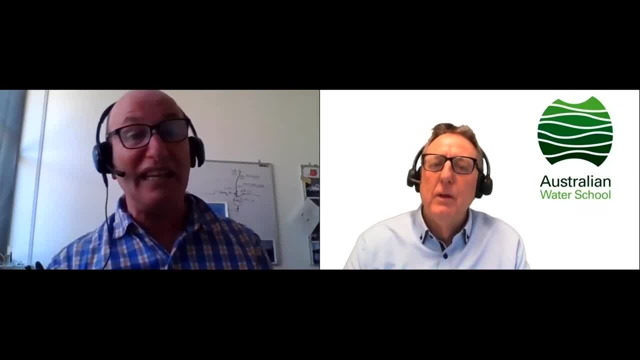 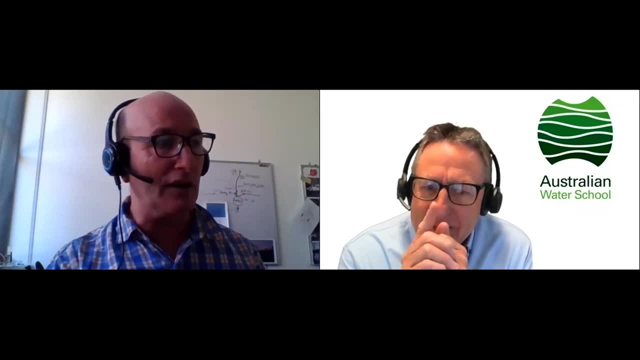 living in the bank or in the channel. So yes, you can. There's a lot of literature out there. I would like to have a go at the second part. That's the twist. The second part is the twist in the tail. 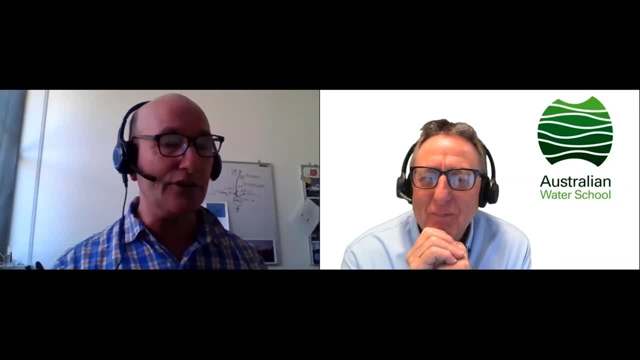 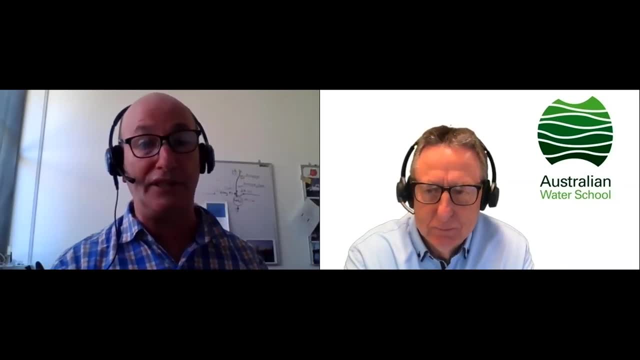 It is. Is there a point downstream where the rivers recover Again? thank you, Sanjay. We picked for two of those rivers. we picked 22 Ks downstream and 18 Ks downstream. We picked that. we thought surely. 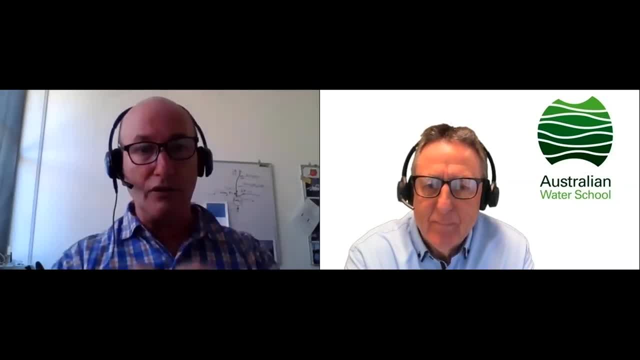 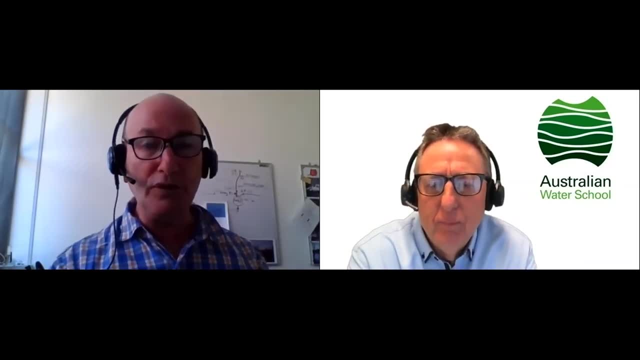 the effects will be over by here. A lot of the metals oxidise, fall into sediment and really leave the water column. How far 22?? 22 and 18. Both of them were way beyond the guidelines at that level. 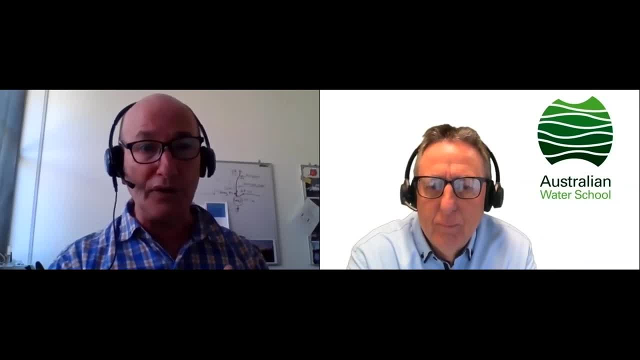 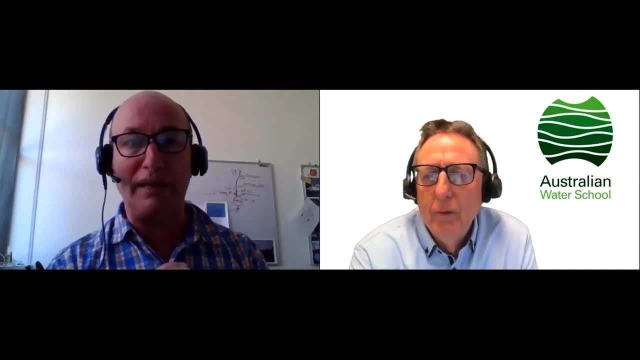 And at 22, that was the Wollongambie- we still found the invertebrates were hammered. It was still having like a 60% degradation of the ecosystem, depending on what metrics we used, And in both of those it was just inaccessible. 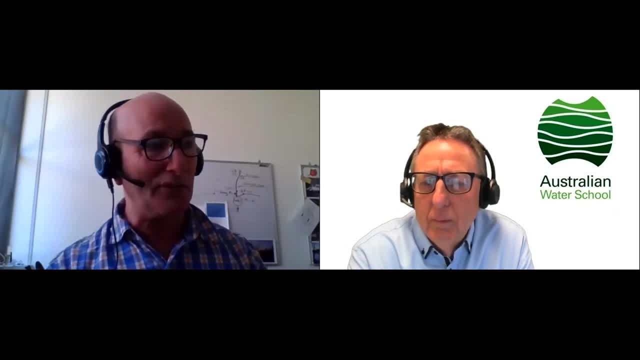 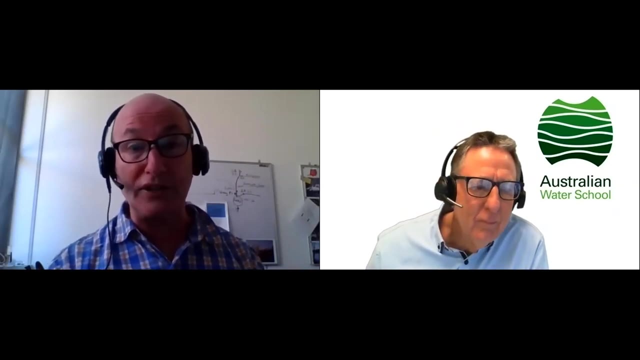 and too difficult to access. But yes, I'd like to find a point downstream where the rivers recover. That's saying that I would say for many mines it's likely they recover in possibly even a shorter distance. For some of them we just did an upstream-downstream. 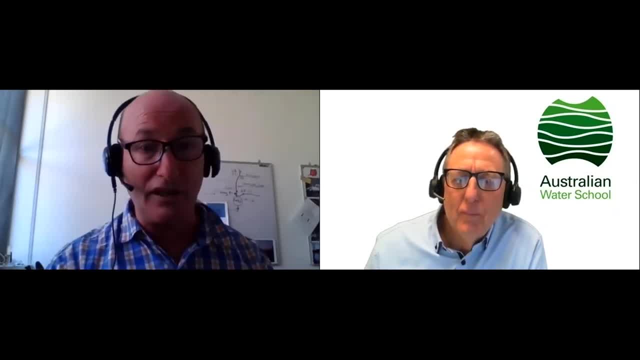 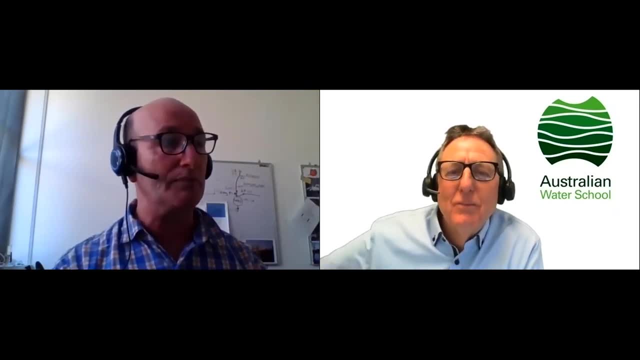 comparison based on a limited budget, availability of labour And I've got to say we've had co-operative students that can carry heavy packs in difficult locations. But great question, Fantastic discussion, everyone. I think we might make this the last one or two questions though. Carolyn Champion. 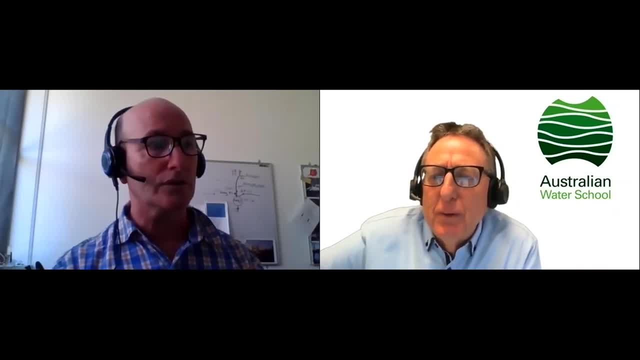 in the UK, they taught in 2007 that succession planting can trap and hold tailings in place. In 2012,, there was research in Canada showing that certain plants were able to bioremediate bioaccumulate copper in order to remove it. Yeah, 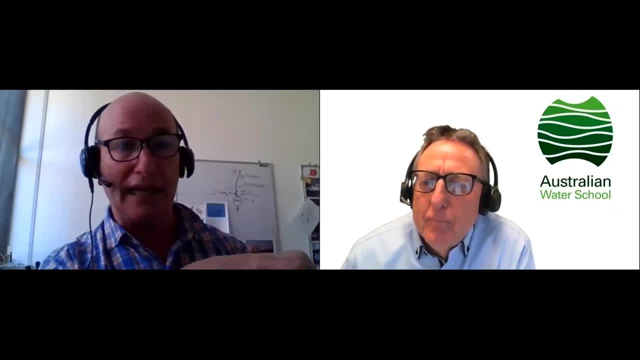 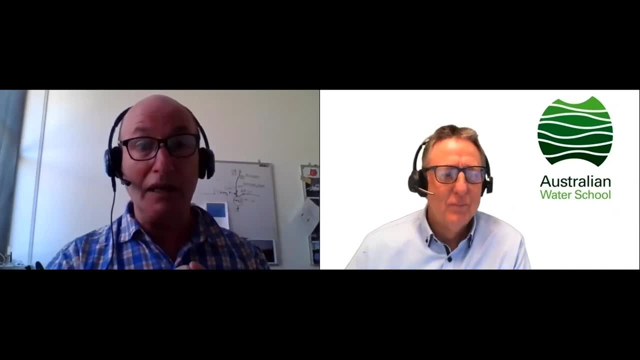 great point, And that's one of the reasons we're looking at plants. we're actually using willows And we're studying willows. There are pest species here, but they're also easy to grow. But we're doing it with a view to 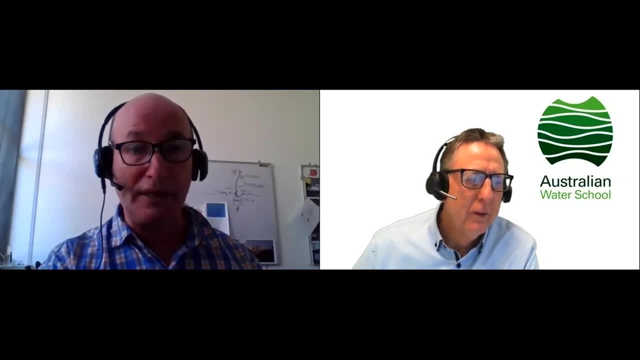 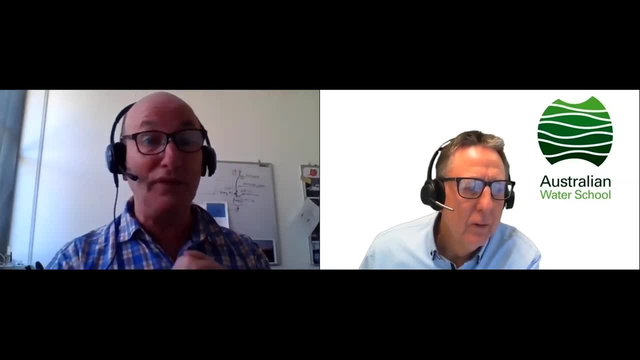 potentially using them for bioremediation or phytoremediation if you like. So the idea of growing them and then perhaps catching that material and putting it probably in landfill. It's very, very hard once you put these contaminants out there. how? 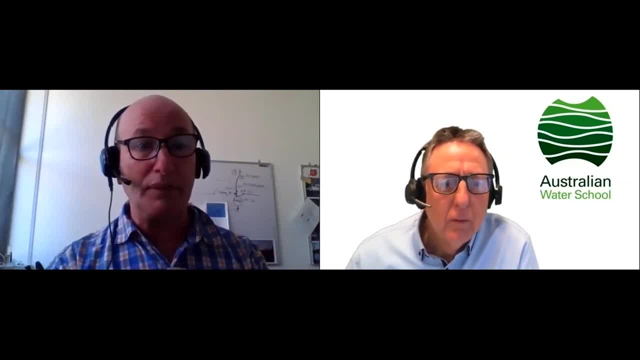 you actually stop that effect further downstream. But yeah, look, that's a really good point And we are looking at that as a potential management technique to reduce the impact of contamination. Let's make this the last question from Julia. then, Julia Emery, Have you found an increase in? 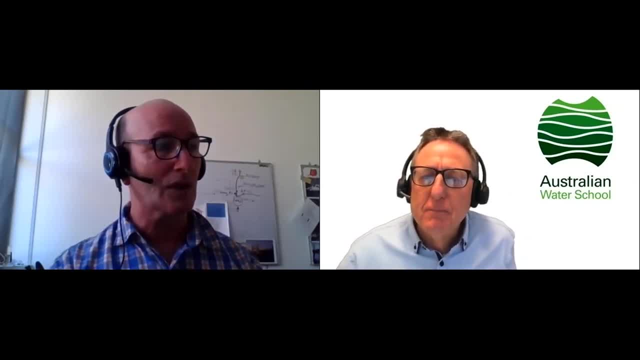 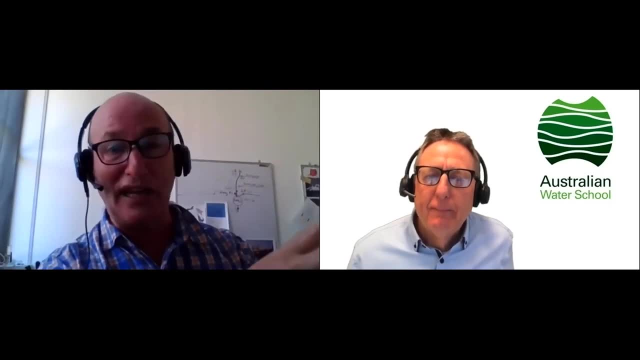 algal blooms downstream from discharge points And, if so, what types? That's a really good question to finish on, Trevor, And a really good, really really good question. In fact, we're working on that now. It's one of the reasons we've started. 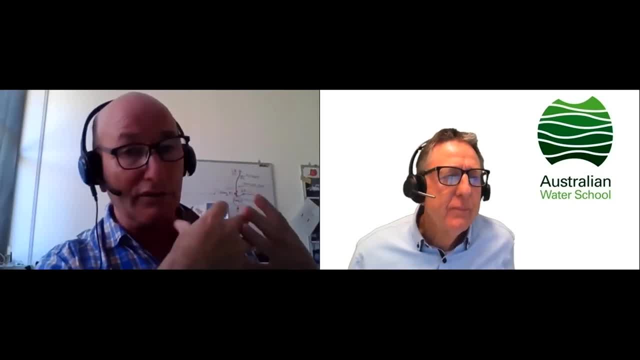 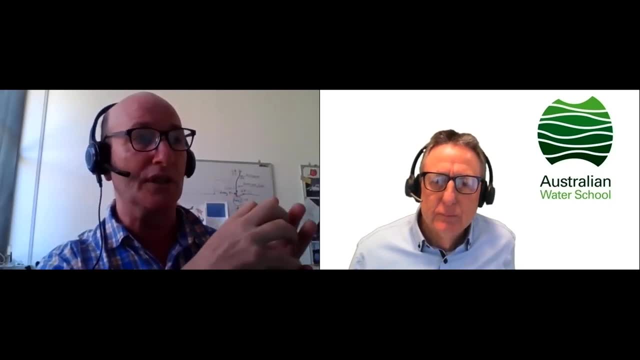 looking at algal blooms, But I have in the very low flow conditions we have in Australia at the moment. in the very low flow conditions I have seen filamentous algal blooms downstream And I've also seen algae in the water column. 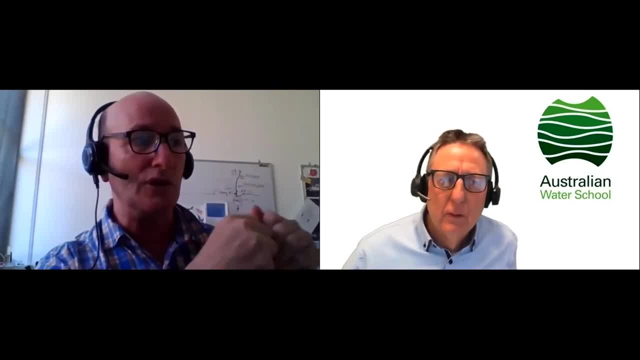 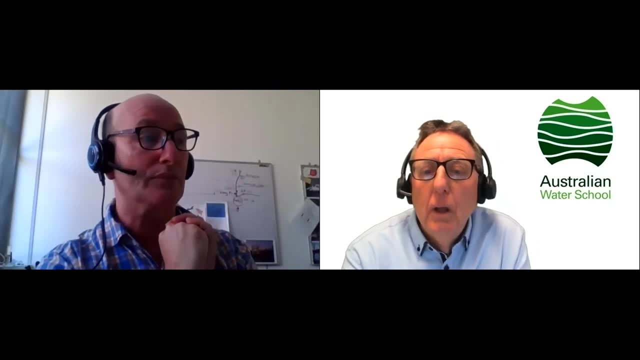 So we are working on exactly that, Julia. I've seen it. I haven't got it documented, But that's future research. Great point, Thank you. Just want to close, Ian, before we close, just say these two things. 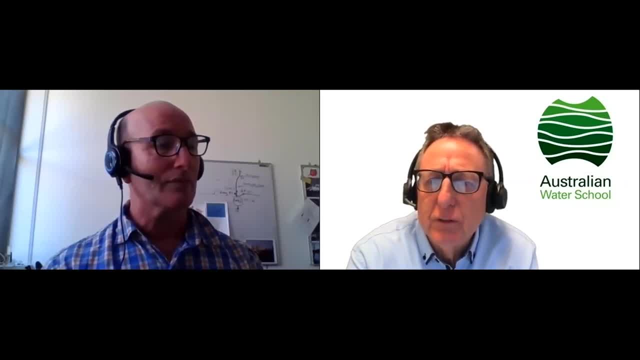 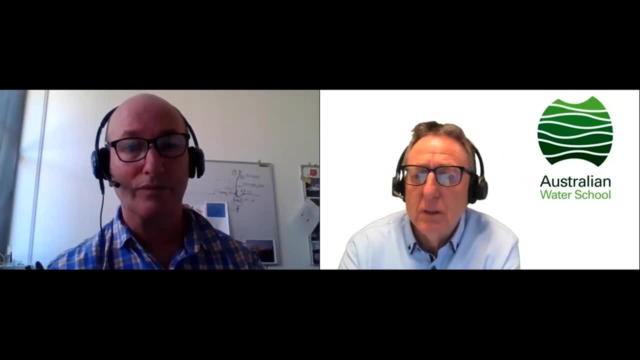 Thanks, Ian. Very informative and a lot of information is highly transferable to other industries to right model conditions. Yeah, that's important, Julia says. thanks, Ian, Great presentation Also Johannes de Beer. thank you for your comment, Great. 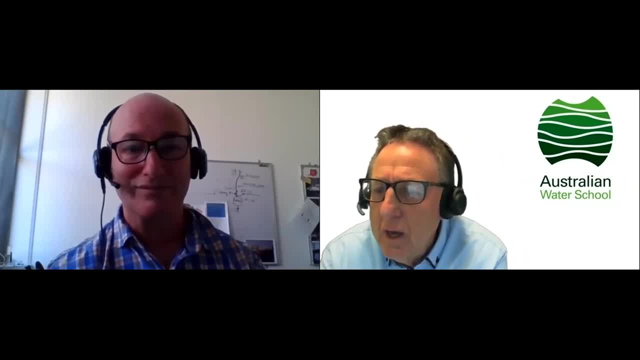 to meet you last week at the groundwater conference, Johannes. Thank you, Ian, for a great presentation. Thank you, You know I think you're more than a scientist. You're keen to see the benefits that should come from science And that shines. 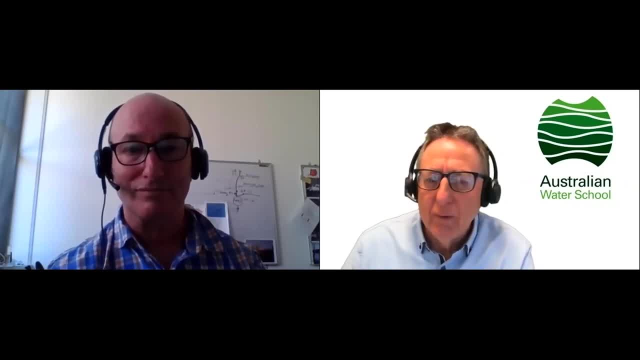 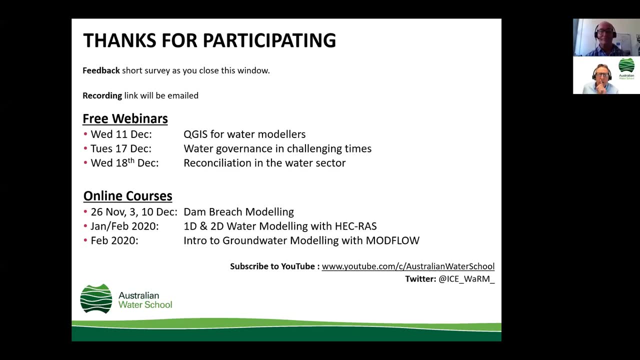 loud and clear. Well, I think we're just about there. I reckon we should close this down. Maybe just have a look at this last page. here We've got feedback. We'll be really appreciating it. We'll send you a recording. 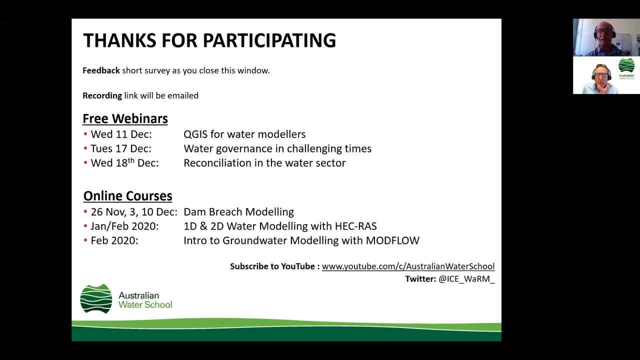 a link to the recording of this. everyone Fantastic. There's three webinars coming up there and they're filling up fast. I can tell you that Online courses down there. I won't say any more except to say we're so delighted. 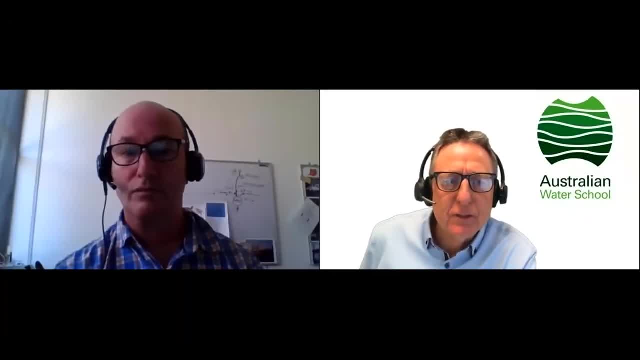 that everyone's joined us and joined in the discussion, And thanks so much for your preparation and your time in all of this. Ian, It's been a great to work with you. Hope we can do it again- I would love to- And thanks to you, Trevor. 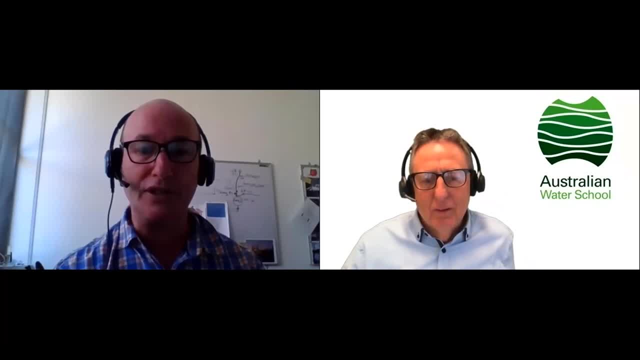 Ice Swarm, And thanks for all the participants. They were really good questions too. And thanks for the encouragement- Absolutely wonderful. We'll do this again. Thanks everyone for joining us today. We'll see you again. And see you again, Ian, for sure.